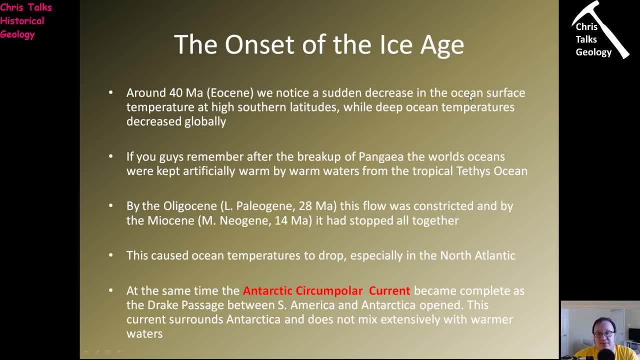 very, very broad sense. Okay, so we're talking about factors that, will you know, contribute towards the Ice Age, but they are not the cause of the last Ice Age. Okay, there's many factors combined together which led to the onset of the last Ice Age. I should point out that we will not 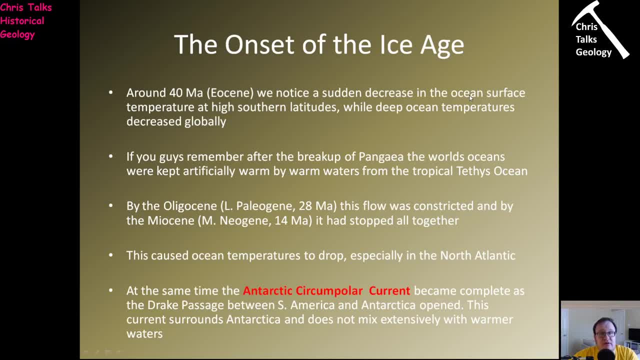 be dealing with something called Milankovitch cycles. Okay, so Milankovitch cycles are cycles to do with the position of the earth relative to the sun and the tilt of the earth. So these are contributing factors as well to the onset of Ice Ages. 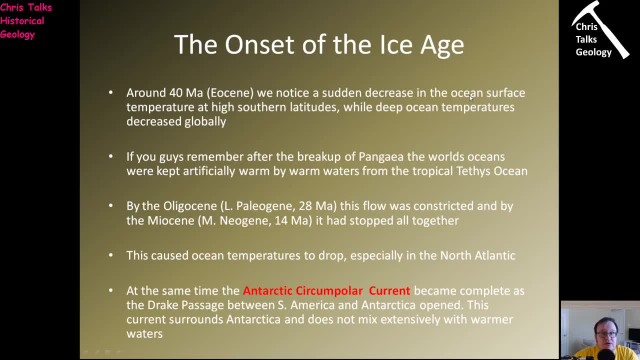 If you want to know about them, you will find them in the textbook and you'll also find a pretty reasonable discussion actually on Wikipedia. So all right, let's get talking about the onset of the last Ice Age. Okay, so around 40 million years ago, we begin to notice a couple of things. We notice, first of all, there's a decrease in ocean surface temperatures at high southern latitudes, So we begin to see that water temperatures begin, towards Antarctica, begin to get colder. We also notice that, on a global scale, deep ocean temperatures begin to get colder as well. 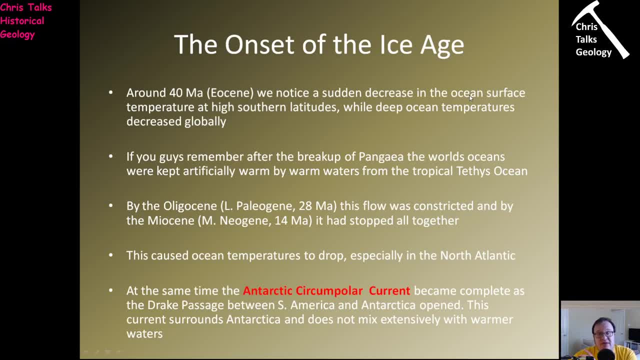 So what's this telling us? Well, if you remember, we've spoken already about this- nice you know- circulation of water coming from the Indian Ocean, going into the Atlantic and then going into the Pacific, and that helps to keep the Atlantic and the Pacific that little bit warmer. 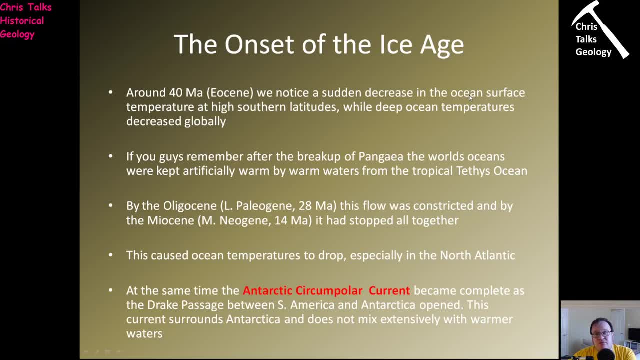 than they should be. So what's this telling us? Well, it's telling us that this flow of water is possibly beginning to become a little warmer. So what's this telling us? Well, it's telling us, a little bit more constricted So by the Oligocene about 28 million years ago. we begin to see this. 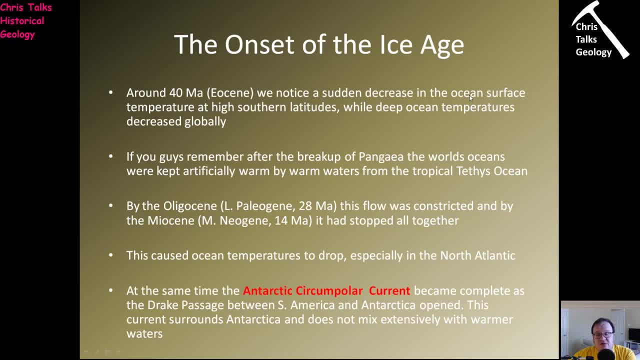 flow really slowing down. Okay, so the situation is, the flow is very constricted by this point and by the Miocene, 14 million years ago. the flow has stopped altogether. Okay, and we see this, and we see this as changes in ocean temperature, and the North Atlantic was especially hard hit by the loss of this warm water. 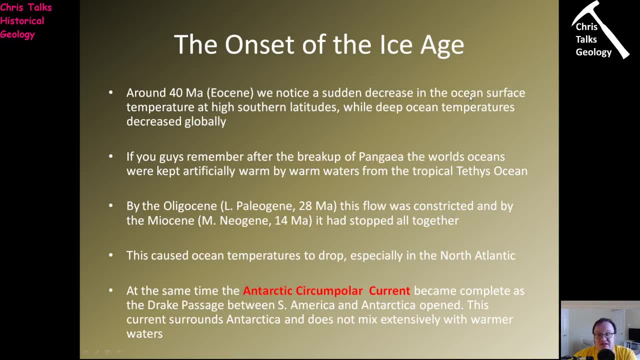 At the same time that this is happening, we have the establishment of the Antarctic circumpolar current, and this essentially is a current that rings Antarctica and it essentially separates it from the other bodies of water, and the water in the in the Antarctic circumpolar current is cold, so it helps to keep the climate of Antarctica cold. so you know it. 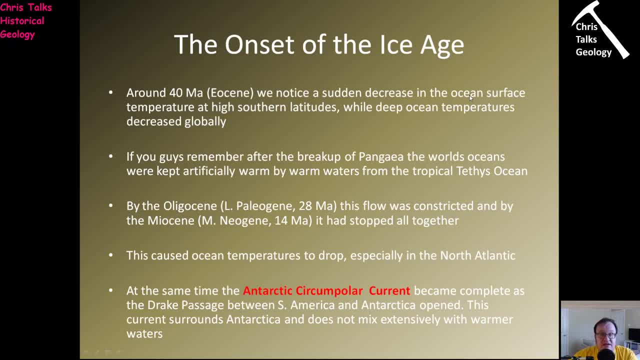 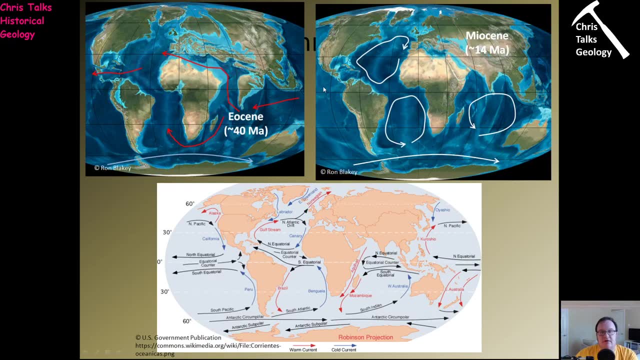 helps to contribute to the- you know the Antarctic ice sheets formation. There we go, Okay, so these maps are going to kind of show you generally what was going on. so we have the Oligocene over here. so this is this flow of warm water. it's coming from the Indian. 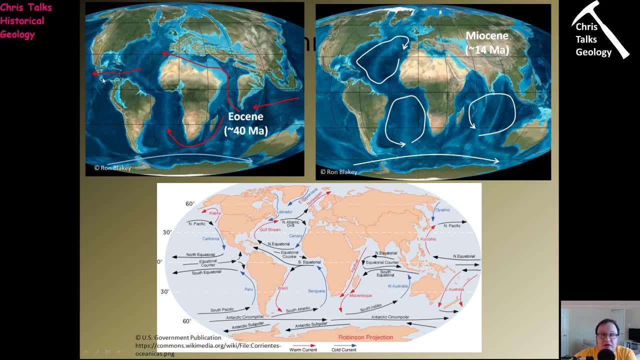 Ocean, going into the Atlantic and then going into the Pacific. You will begin to notice, though. look here, the continental shelf of Africa is starting to head towards Europe. This area is starting to get tighter, so the flow will be slowing down Now, obviously, as we can see over here, the the 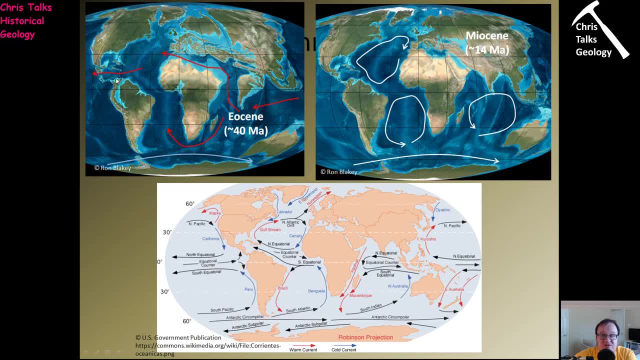 the link between North and South America is also steadily establishing itself. Okay, by the time we're in the Miocene well, Africa has made full contact with Europe and the flow of warm water from the Indian Ocean into the Atlantic has been completely cut. Now, you'll notice, by the 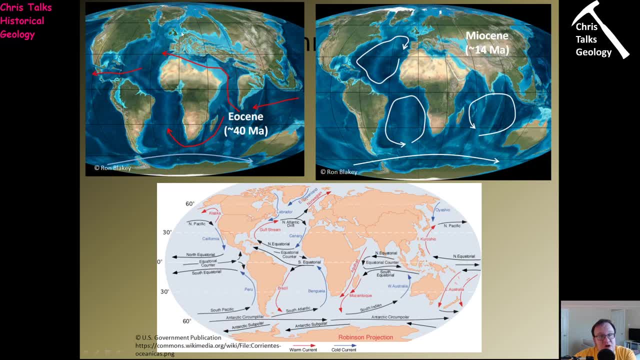 way that the flow itself, as it comes in here, would have been focused primarily on the North Atlantic. so that's why the North Atlantic is so hard hit, because all of a sudden all that warm water gone. Now you will notice there is a. you do have the capacity to communicate between. 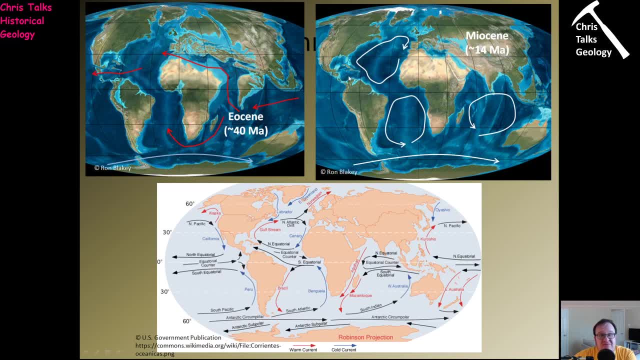 the Atlantic and the Pacific just about, but that doesn't really mean much anymore. So, okay, you can see, by 14 million years ago we have these individually circulating bodies of water, each with their own individual climate. and if we come down here and look at this diagram at 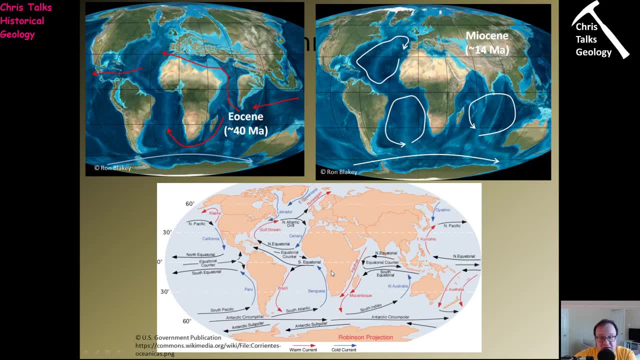 the bottom, you can see them more clearly. so we have the North Atlantic, the South Atlantic, South Pacific, North Pacific and South Atlantic Pacific, the Indian Ocean and the Antarctic Circumpolar Current, And these are the main circulating bodies of water. 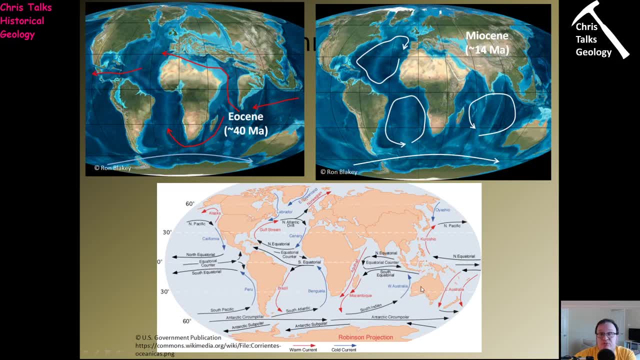 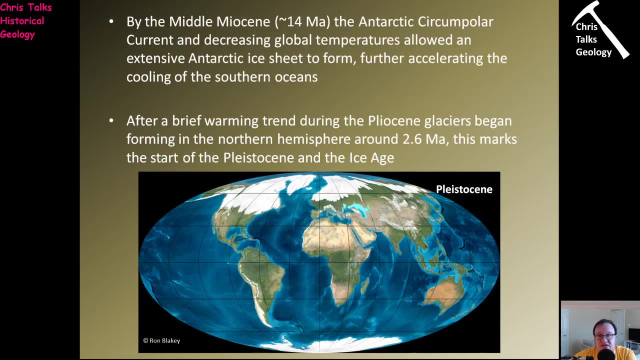 Now there are some smaller ones, don't get me wrong, but on the whole these are the main bodies. So by the middle of Mars, seen about 14 million years ago, we have the Antarctic Circumpolar Current establishing itself and we see a decrease in global temperature. 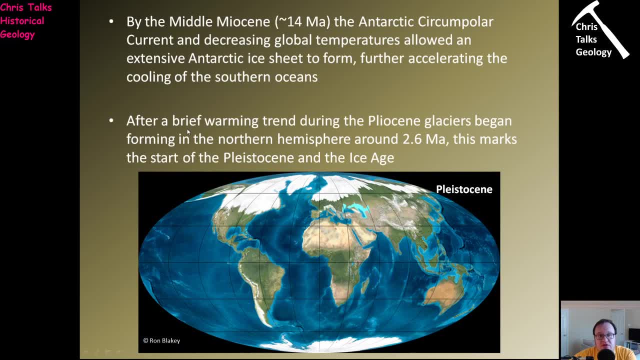 And now this establishment of the Antarctic Circumpolar Current essentially allows the Antarctic Ice Sheet to grow a bit larger, and this, of course, will help the colour of the Earth get slightly lighter, meaning more solar radiation will be reflected back into space, so it's going to help cool global temperatures. 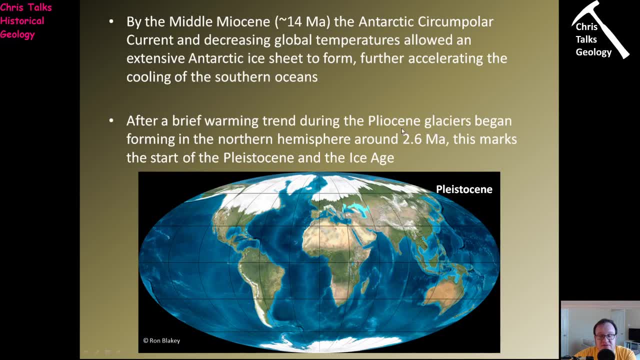 So we also see a brief warming trend in the Pliocene, so just before the last Ice Age, and we begin to see glaciers forming In the Northern Hemisphere around 2.6 million years ago, so after the Pliocene, And this marks the start of the Pleistocene and the Ice Age. 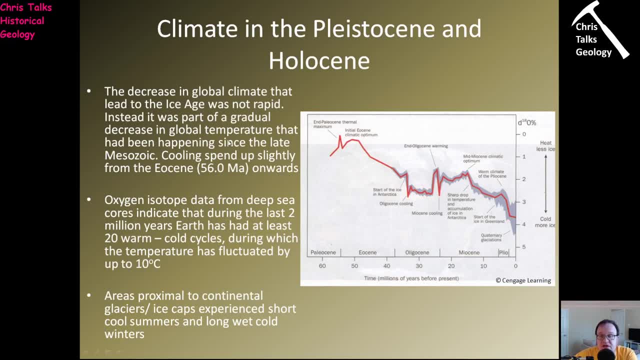 So, in terms of the global climate during the Cenozoic, what do we see? Well, you'll notice that there is a general downward trend. Now there are several periods where we have peaks, Okay- Where we have essentially increases in the global temperature. 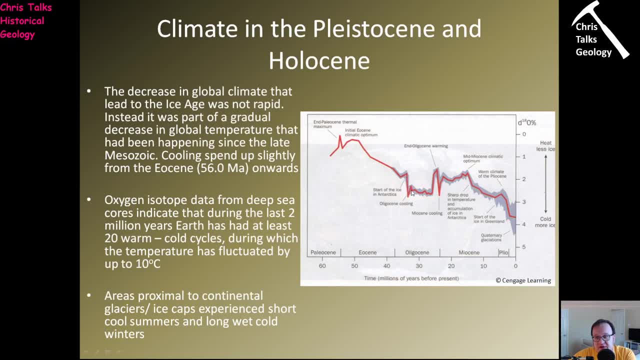 So it's not a smooth downward trend And there are also periods where we have sudden decreases in the global temperature, But on the whole, you can see we have a general downward trend. Now we'll notice that when we look at this downward trend we don't have any temperature. 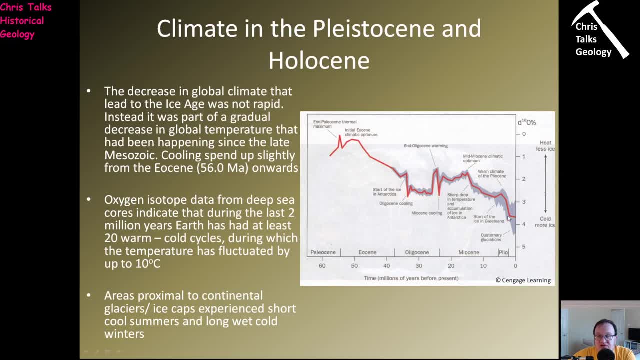 values Okay. What we have over here, though, are the oxygen isotope values, and we can see, in general, that If the oxygen isotopes are going this way, we have cold weather, so more ice. If they're going this way, we have hot weather, so less ice. 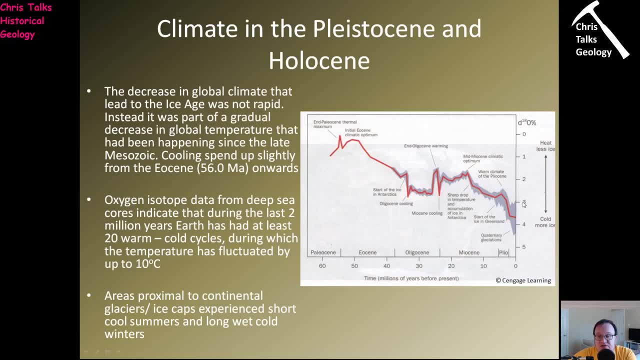 Which kind of makes sense, doesn't it? So this is how we're plotting this. you know, decrease in temperature. We're not, you know, getting temperature values, but we're getting a general idea of what the trend was. Okay. 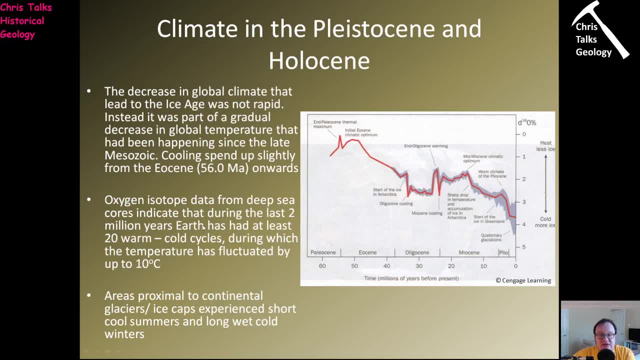 So the general trend indicates that during the last 2 million years, the Earth has had at least 20 warm-cold cycles. We know that from the oxygen isotope data. Okay, We also know that there's been a fluctuation in temperature of up to 10 Celsius. 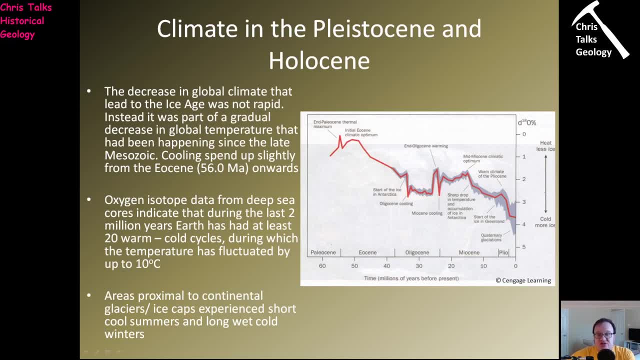 What we also begin to notice during this period is we begin to see that there's a shift in local climates as well, And so we begin to notice. in the more norvally areas, we noticed that areas which are located close to glaciers and ice caps, obviously the temperature begins to drop even more. in 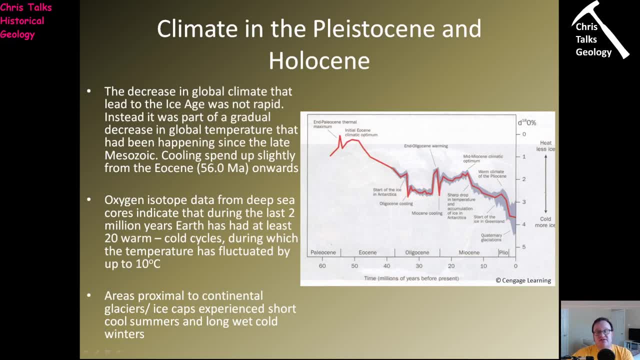 those areas and that's going to encourage the formation of ice and it's going to encourage ice to start growing. It's growing outwards from these locations, okay, because you know, if you think about it, if the area directly in front of the glacier is nice and cold, that's going to encourage. 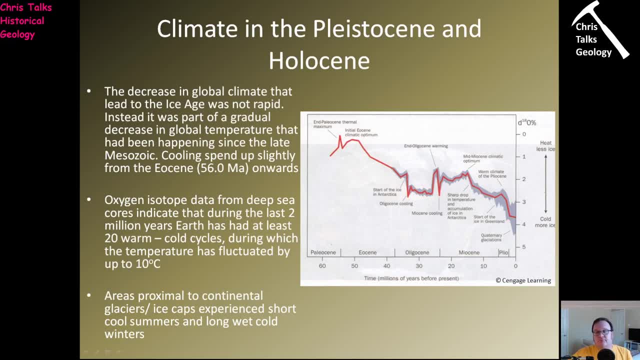 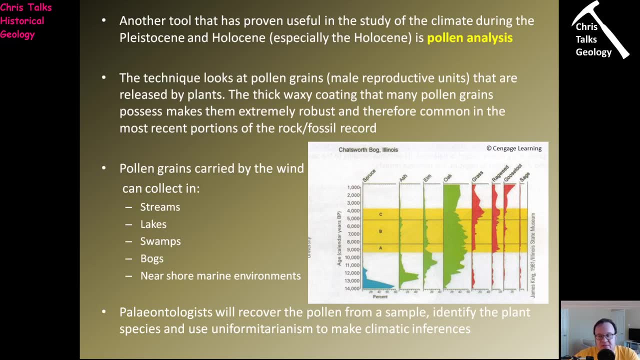 the glacier to move into that area. So one of the other ways that we can tell and get some idea about what was happening during this timeframe is pollen analysis. So we've generally been speaking about, you know, oxygen isotope analysis using things from the ocean. 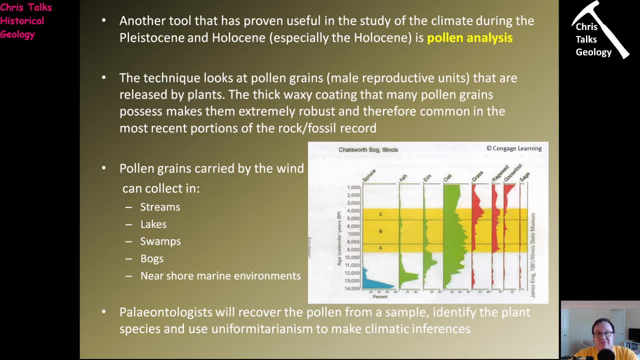 Okay, So we get an idea, using pollen analysis, of what was happening on land. Now, this isn't really helpful in terms of telling us what was happening during the ice age, because obviously these areas were covered in ice. so you know. not much help there. 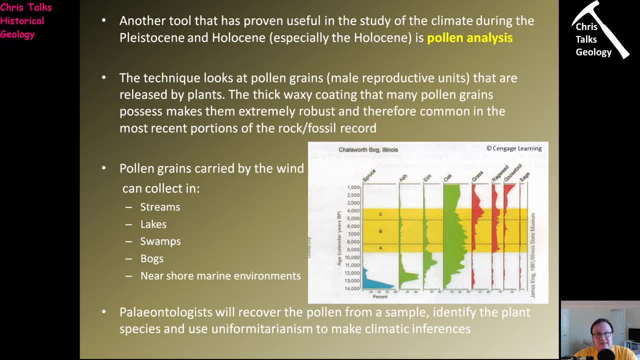 But they are more helpful in telling us about when the ice age was ending. Okay, It's not going to tell us about, you know, the huge changes in the environment. It's going to give us some kind of hints about what was happening, though. 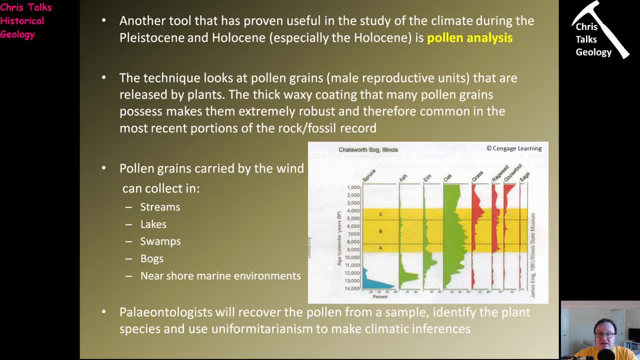 So pollen analysis. So pollen analysis uses pollen, pollen grains collected from, essentially, environments where they will be retained, So environments like rivers, lakes, swamps, bogs and near shore marine environments. So we can take sediment, take sediment samples and we can essentially wash them until we. 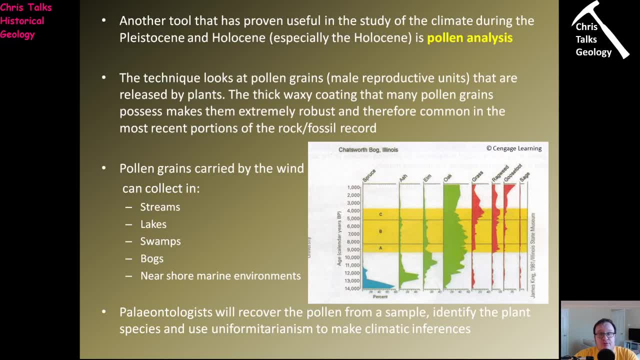 get the pollen grains out and then the pollen grains can be analysed down the microscope. So one of the things that we know is that individual different plants have different pollen grains, essentially, So we can identify the plant by the pollen grain. So this is information from the Chatsworth Bog in Illinois. 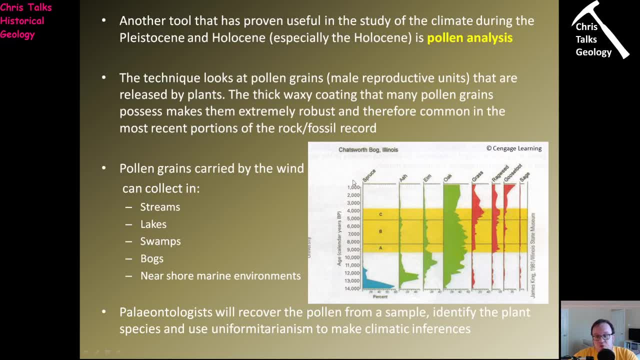 So here's an age range so 14,000 years ago to 1,000 years ago. So what we're going to see is we're going to see changes in the plant life depending on the conditions. So okay, So around 14,000 years ago, you can see we have quite a large amount of spruce pollen. 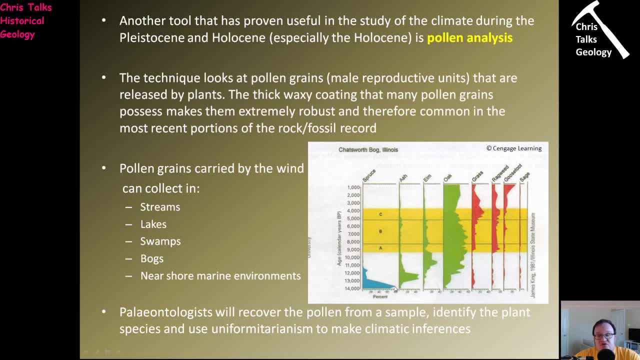 Now, spruce is a coniferous tree. It's the kind of tree that makes up a large part of the boreal forest. Now, this is the kind of forest that you get in northern Canada, northern Europe and northern Asia. Okay, 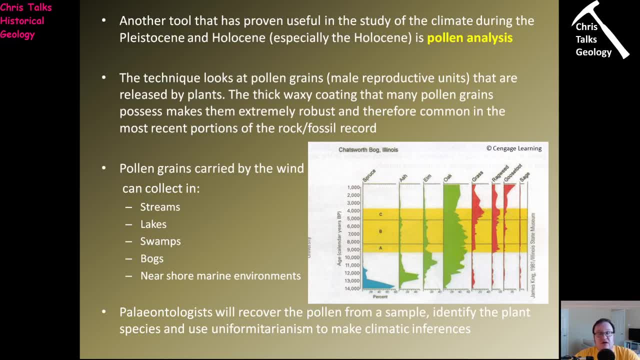 It's made up of lots and lots of, essentially, pine trees- for want of a better term for them, spruce trees, Okay, And so this is a cold weather forest, And so what you can see happening though, around 14,000 years ago to 13,000 years, you can see. 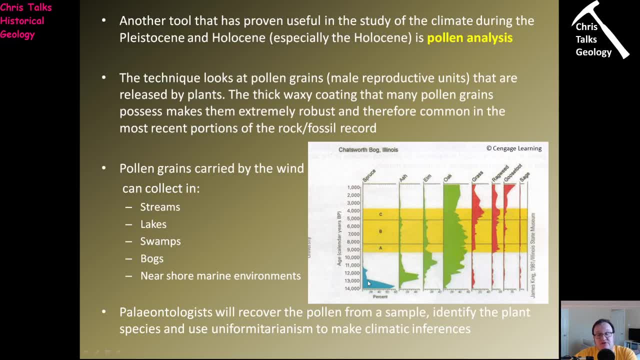 the amount of pollen is dropping off hard. Okay, So this is telling us that the ice sheet is really retreating now. Global temperatures are on the way up, The ice sheet is going to be retreating quickly, And you can also see the same thing happens for this cold weather forest. 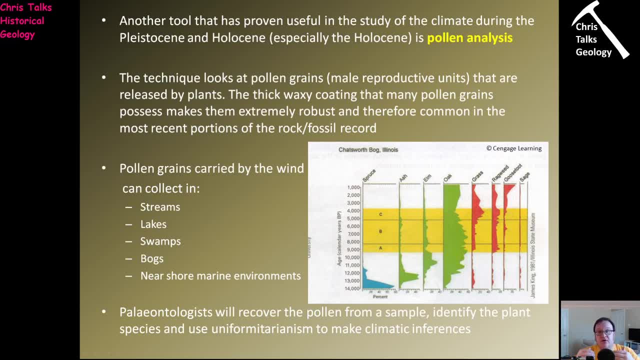 It's dying back very, very fast and essentially it's having to follow the glaciers northwards. Now what we notice is that the spruce trees are replaced by ash trees, So ash is the first tree that forms. It forms in a deciduous forest. 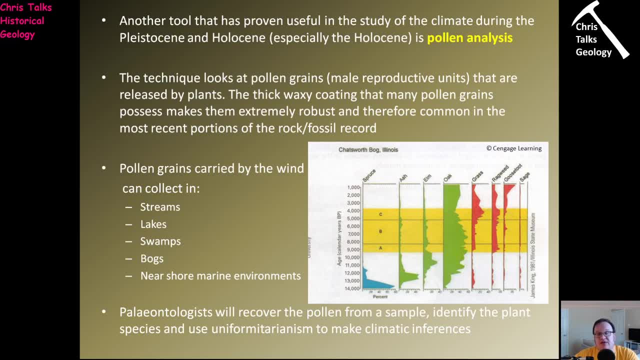 Okay. So if I was to go, you know? oh, I should point out that it's also an indicator of temperate conditions. Okay So, colder winters and autumns, but warmer summers and springs. So what this means is if I was to go to somewhere like the United Kingdom and I would just take 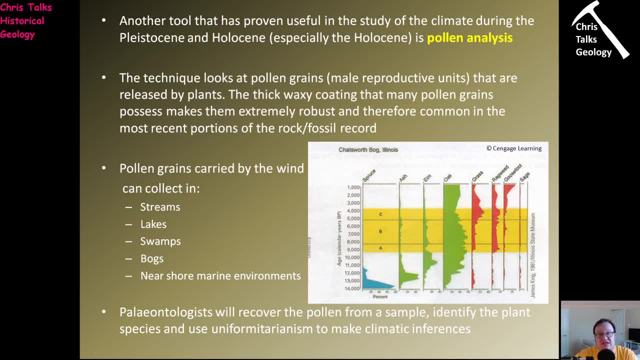 an acre of land and I just left it, completely left it, left it to nature. the first tree that would appear to appear growing on that land would be Ash. trees is an indicator that deciduous forest has started growing Now. the ash doesn't last particularly long because it's very quickly out-competed by 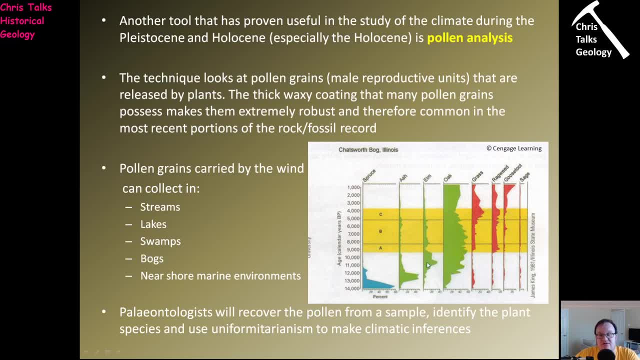 both Elm and Oak, Okay. So they take over pretty quickly, And essentially what we have at this point is: we've established ourselves a forest. Now what we begin to notice is that occasionally the amount of grass increases and then decreases. That corresponds quite nicely to changes in the amount of Oak. 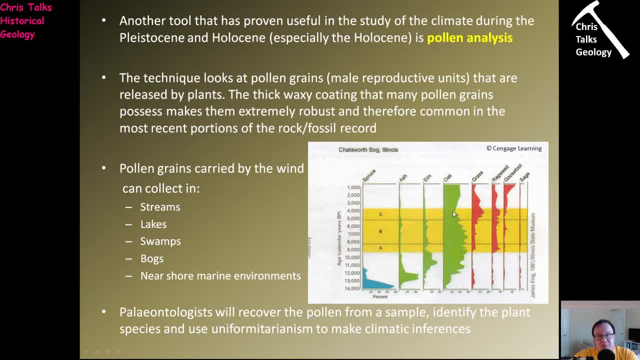 So this is telling us at this point that the Oak forest is dying back and it's being replaced by grasses Now. this can indicate a range of different conditions, but one of the conditions it can it can suggest is a warming in the climate. 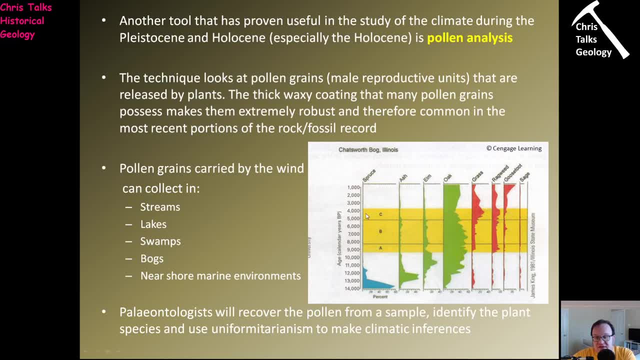 So, you know, this might suggest that somewhere around four and a half thousand years ago, global temperatures might've gone up a little bit. Okay, Now you'll notice, though, that there's then a decrease in the in the grass, and it's then. 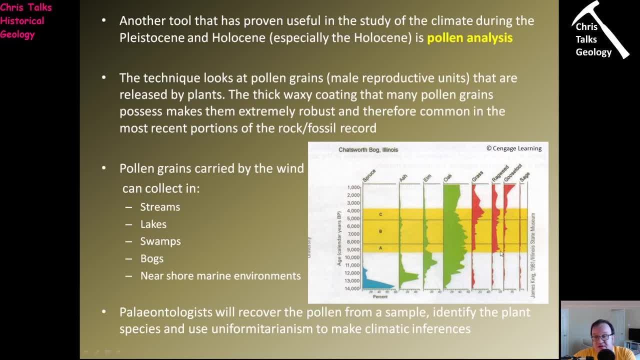 an increase in the Oak that match it. Now you'll notice, throughout this entire period we have an increase in ragweed and goosefoot and these kind of these indicate that we're dealing from. you know, we're moving from a kind of very dense forest to a more kind of open, sparse kind of set of conditions. 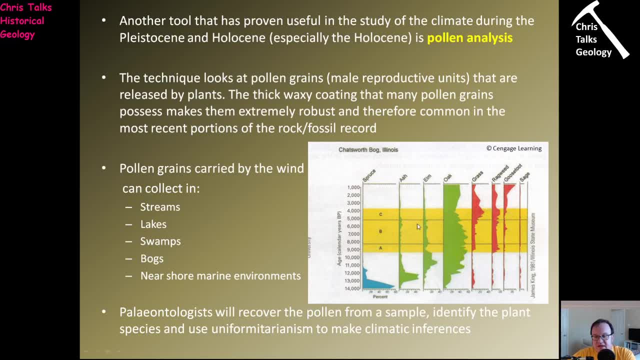 So it's telling us something about the forest development. So you know, down here It looks like We have a very, very dense forest and then slowly, over time you'll notice the forest is becoming more and more open. you know, essentially a a bit of a looser configuration. 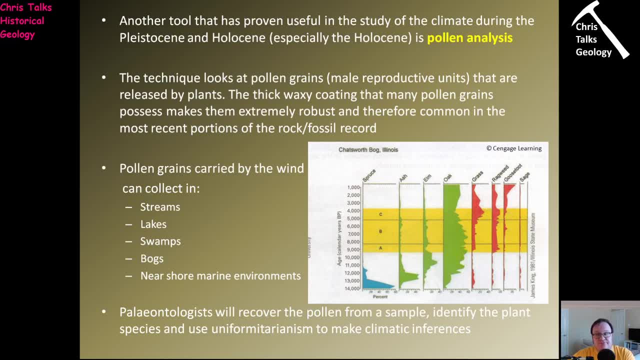 And so there's more grasses in between the trees. So that's what we're seeing, and it's obviously telling us quite a lot to this poll analysis. It's pretty good. Now, if you combine that with tree viewing analysis, then you're really well away. 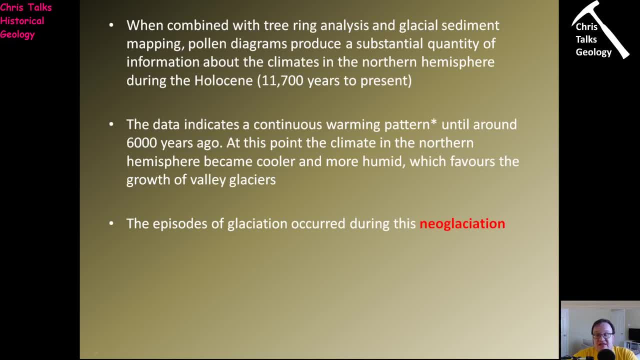 Now the thing about tree viewing and that tree viewing analysis is: tree viewing Analysis can actually be used to give us solid numbers. We can get solid dates, and tree viewing analysis can actually go quite a long way back. Now one of the things we see from this data is: the data indicates a continuous warming. 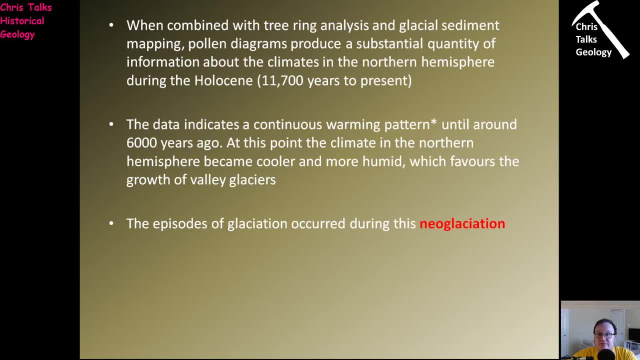 period until around 6,000 years ago. Okay, So in general the climate was getting warmer. So at this point we begin to see the climate of the Northern hemisphere especially become cooler and more humid, and that's going to favor the growth of glasses, especially Valley. 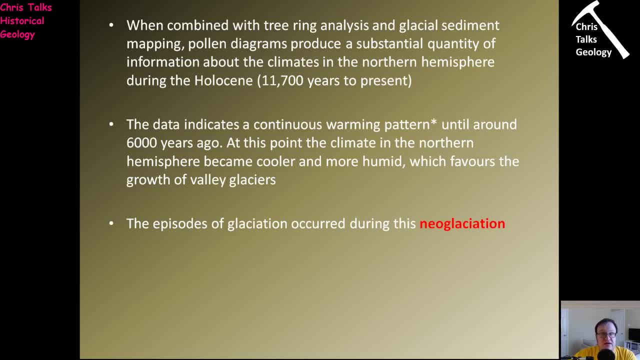 glasses. So mountainous areas. now. obviously, since then we've seen the temperature pop back up very, very recently. So the episodes of glaciation occurred during this. so the the episodes of glaciation occurred during this neo-glaciation. 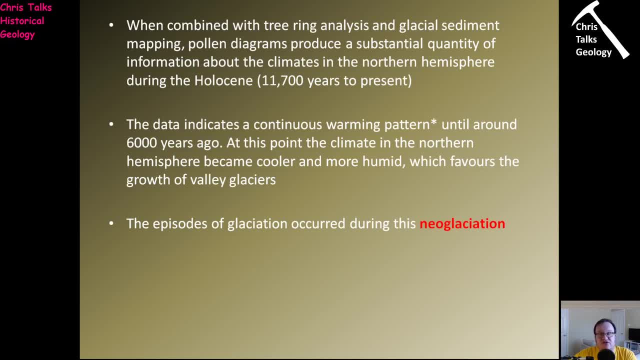 Okay, This is the the start of the glacial period. Now what am I saying? It's essentially. sorry, I do apologize, I'm saying myself completely mixed up there. This is a small glacial period within the uh, the Holocene. 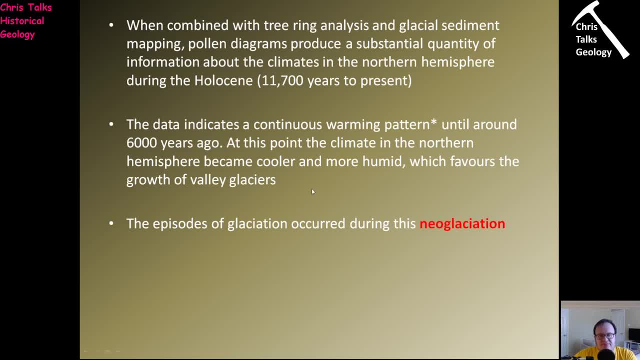 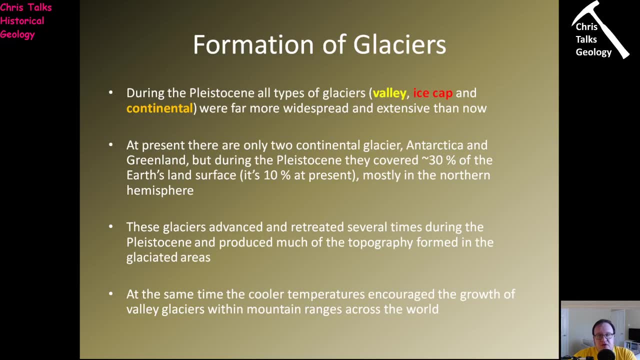 Sorry about that. Got horribly confused. I lost track of my dates. So how did glaciers actually form? So during the Pleistocene we had all types of glaciers: Valley glaciers, ice caps and continental glaciers. Now, at the moment, we have Valley glaciers and two continental glaciers. 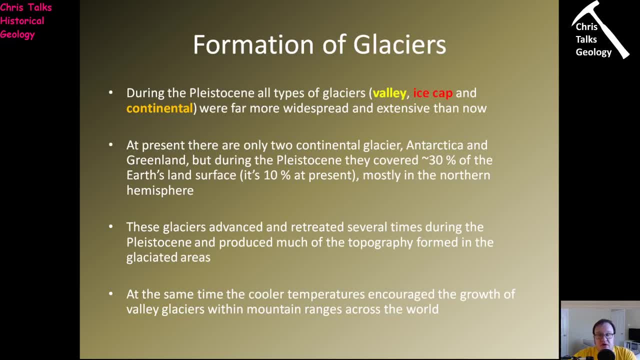 Those are the types that dominate. So as at present there's only two continental glaciers, but during the Pleistocene continental glaciers covered 30% of the earth's surface, And now at mo, now at the moment, you know, it's kind of about 10%, give or take a little. 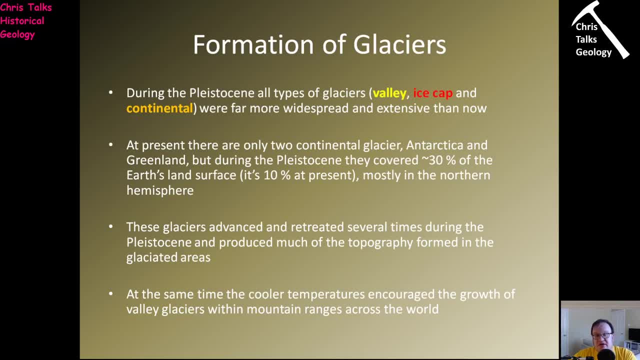 bit And those and that, uh, that cover is mostly in the Northern hemisphere in the form you know, in terms of you know what's on land, It's actually. that statement is completely wrong, Isn't it? 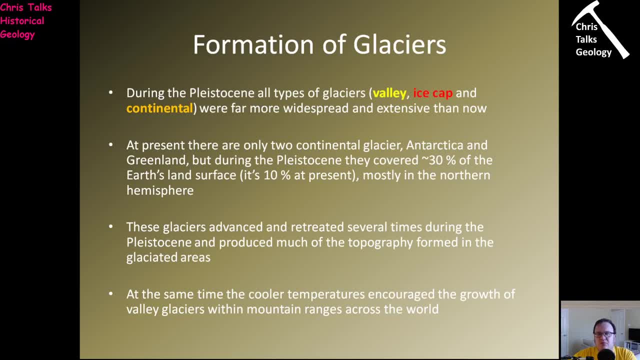 That's good. That's a really wrong statement. Yes, Ignore me on that one. Yeah, No, just ignore me. Essentially, We have two continental glasses. Just stick with that. I don't know what I was writing there. What's what going through my mind? 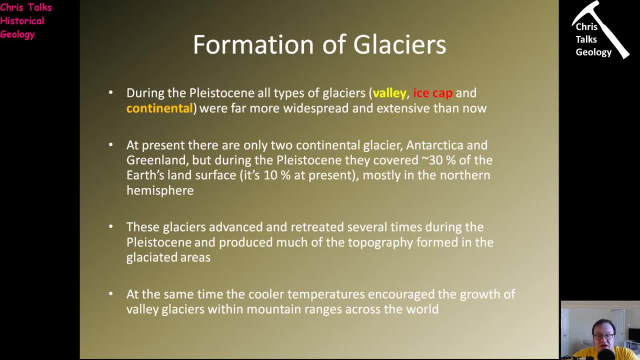 So, uh, these glaciers advanced and retreated several times during the Pleistocene and produced much of the topography formed in the associated glaciated areas. So as a glaciers retreat backwards and forwards, it's going to affect the topography of the area. 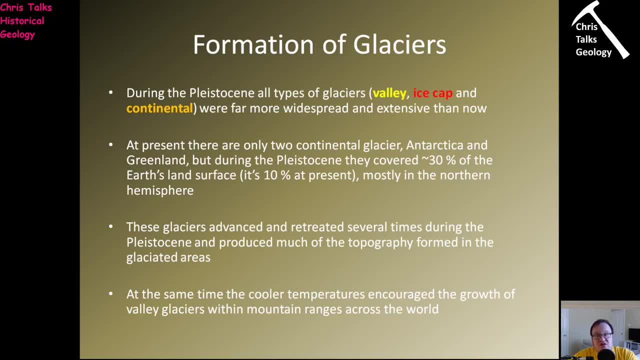 You know, as, as we mentioned, it's going to, you know, grind down the topography in those locations. So, at the same time, the cooler temperatures obviously encouraged the growth of valley glaciers in mountainous areas. So we're going to see the numbers and signs of valley glasses also increasing during periods. 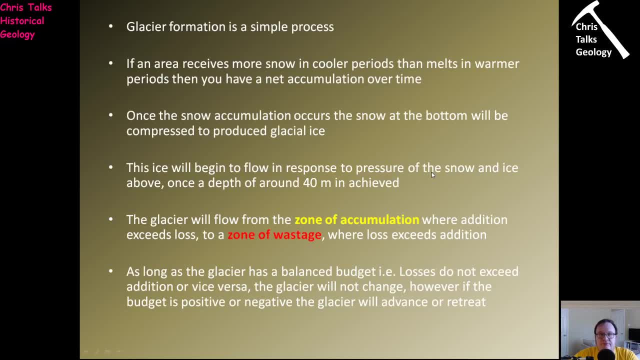 of glaciation, So glacier formation is actually a surprisingly simple process. So in areas that receive more snow In cooler periods than essentially we want, an area that receives more snow in cooler periods, the melts in warmer periods, So you get a net accumulation over time. 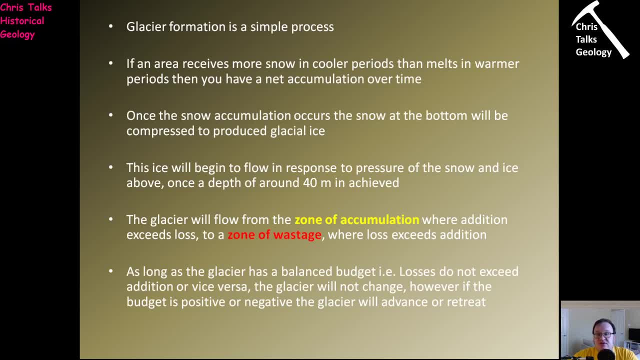 So once the snow accumulation occurs, the snow at the bottom will be compressed and that will produce ice. And this ice will begin to flow in response to pressure as more snow and ice forms above it. So think about it: as more and more weight is put on it, it will naturally want to start. 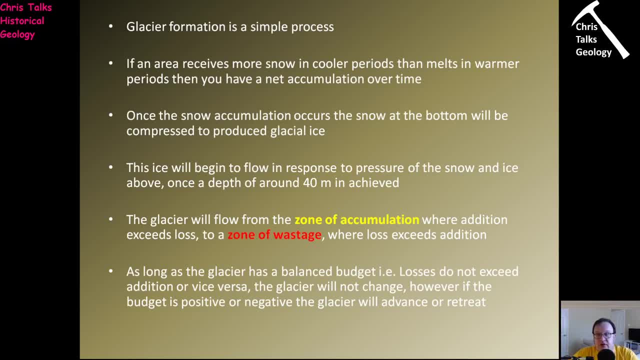 flowing away And that point under gravity, So typically you'll need about 40 meters to make this start to happen. So the glacier will then flow from this zone of accumulation, where you get more snow being being deposited than is lost, And it will essentially go down and to the zone of wastage. the zone of wastage is the. 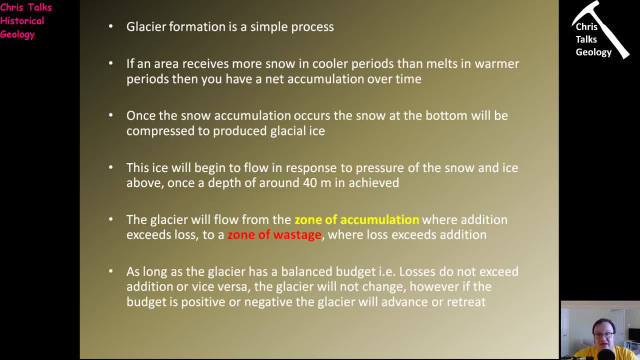 area where you lose more ice and snow than you gain in the colder periods, And that's pretty much it. It's a pretty straightforward process when you think about it. So, as long as the glacier has a balanced budget, so the losses do not exceed the addition and 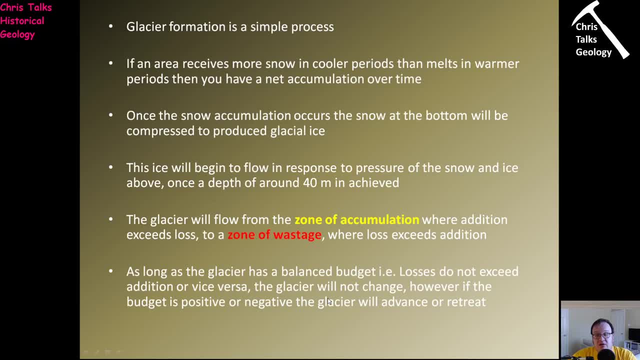 vice versa. the glacier won't change or be stable. However, if the budget changes, obviously the glacier will shift. So at the moment we've seen temperatures going up, So that means the zone of wastage has essentially been moving up the glacier. 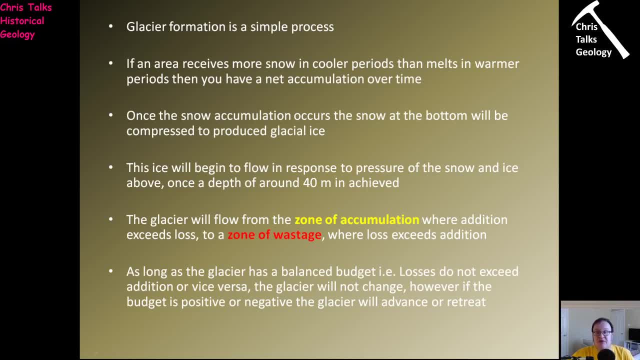 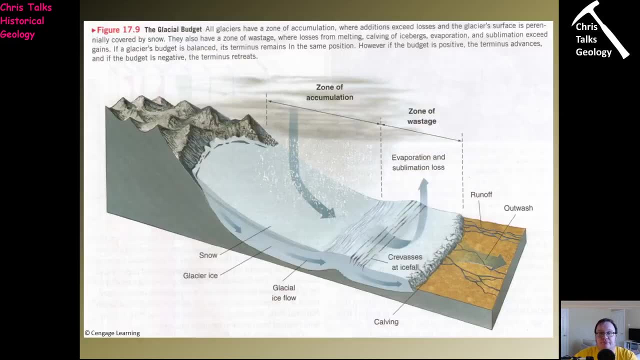 So that means the glacier has slowly been melting away because it's not been maintaining equilibrium. It's trying to, but it hasn't found its equilibrium yet. So here we go. So this is the basic diagram. So we have the zone of accumulation here. 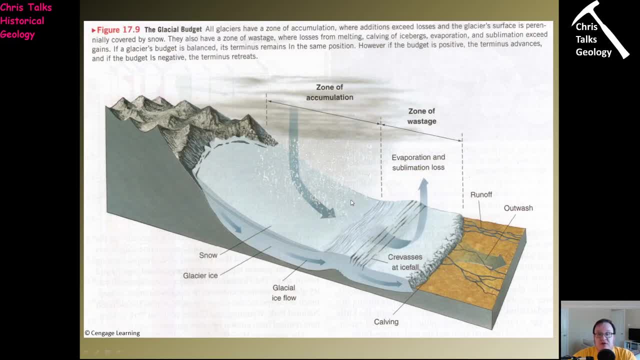 This is where we essentially retain more snow from the cold periods than we lose, So we have a buildup of glacial ice here. The glacial ice will flow downstream under gravity until eventually it meets the zone of wastage, where it will begin to melt and it will begin to deposit any sediment that. 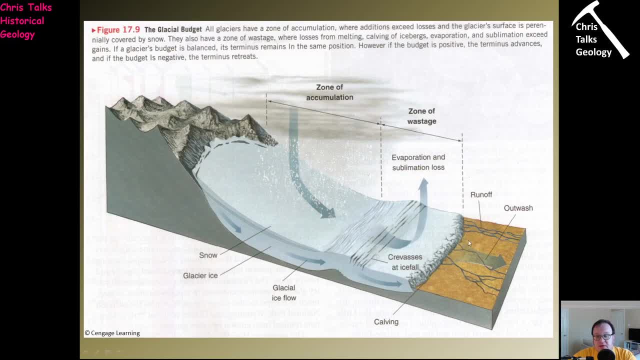 it forms And, of course, if you remember, at the front of the glacier here we're going to have loads and loads of glacial till being deposited, forming a moraine. Obviously, we've also got quite a lot of water coming off the front of this glacier, as it 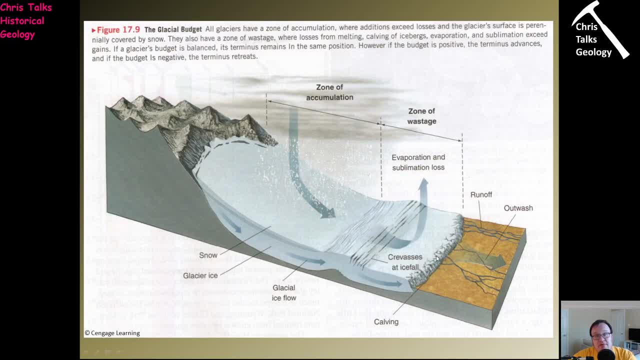 melts That's going to rework some of that moraine, So it's going to transport sediments away from the moraine and it's going to redistribute those sediments here in this area which is referred to as the outwash. So the outwash is an area of sediment. 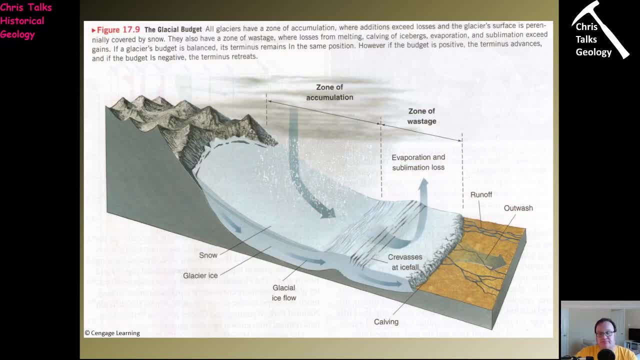 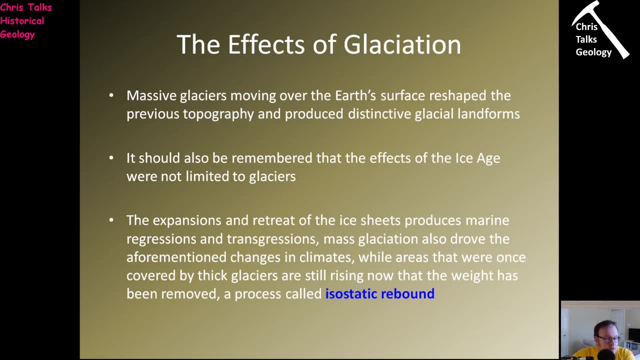 It's going to be redistributed by rivers in front of the glacier. So what are the effects of glaciation? Well, the effects of glaciation are massive glaciers moving over the Earth's surface will obviously reshape it. That's pretty much a given, isn't it? 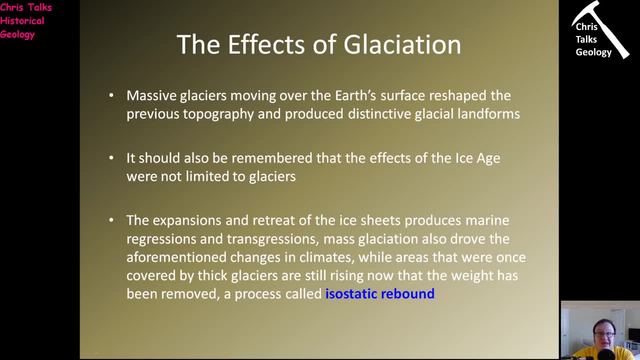 So the previous topography before glaciation is going to take a pretty big hit and we're going to get a completely different topography afterwards. So it should be remembered that the effects of the ice age were not limited to glaciers, So the expansion and the retreat of the ice age produced marine regressions and transgressions. 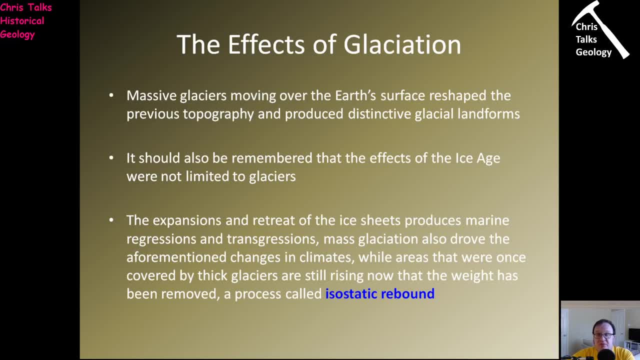 So mass glaciations also drove the aforementioned changes in climate. Remember, the temperate zone got pushed down into what now are dry areas like the Sahara or the southwestern United States. So there are other situations Where areas which were once covered in very thick glaciers are currently bouncing back. 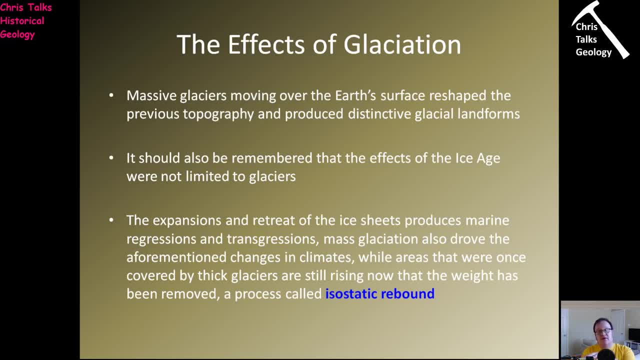 up. Remember, 3 kilometers of ice weighs a lot. That's literally going to push, it's going to cause the crust to warp downwards just due to the weight. And now what's happened is, since the glaciers have been removed, that crust has been slowly. 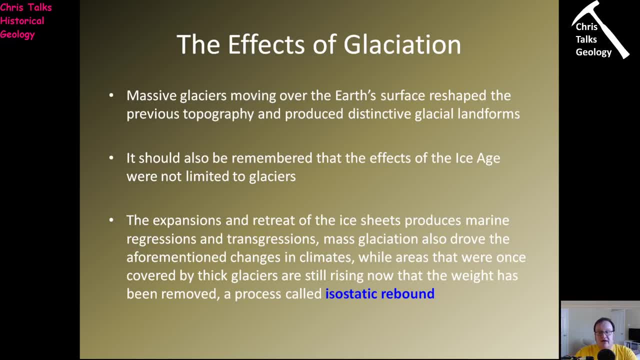 bouncing back upwards, And that's referred to as isostatic rebound. And so what we're seeing there is the crust bouncing back upwards. words: now: the ice has been removed. so the glaciers alone? yes, they cause effects, but there's also several effects which are related to them, you know, in a kind of distal fashion. 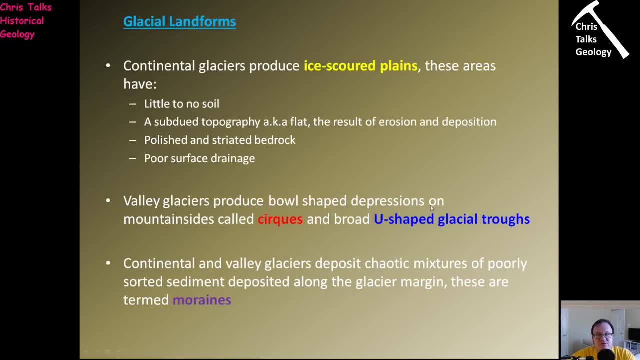 so okay. so what are the landforms which are associated with glaciers? well, one of the most obvious ones is called the ice scoured plain. so remember, this is the area where the glaciers acted like a bulldozer. so there is little to no soil, there is subdued. 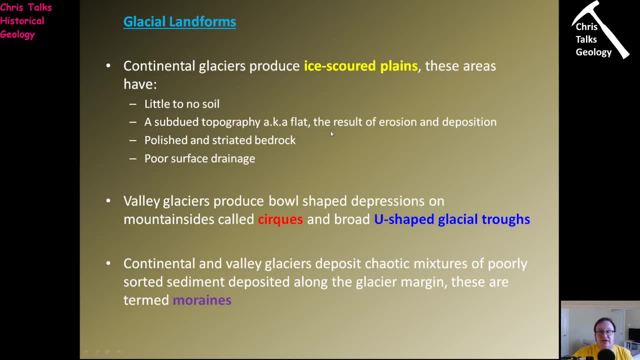 topography. so the area is really, really flat. once again, the glaciers bulldozed away. topography: the rocks themselves are polished and striated- we discussed why that is earlier- and there's very poor surface drainage. well, that's simply because the area is very, very flat. 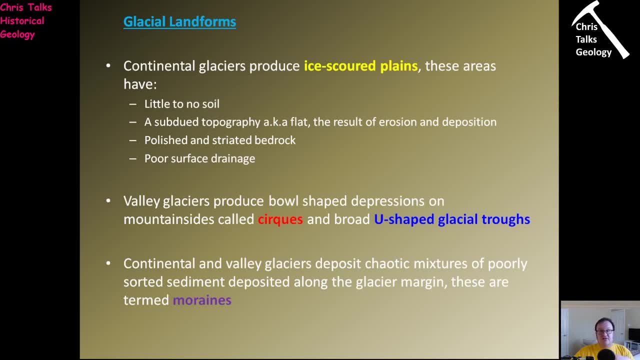 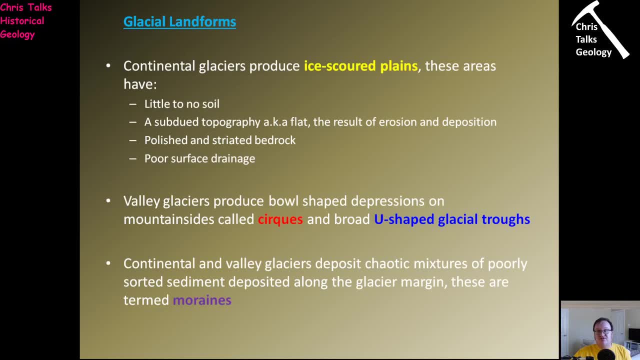 that means no gradient. no gradient means the. that means no gradient. no gradient means the water can't really move anywhere, can it? water can't really move anywhere, can it? water can't really move anywhere, can it? so the water just sits there in terms of valley, glaciers, valley. 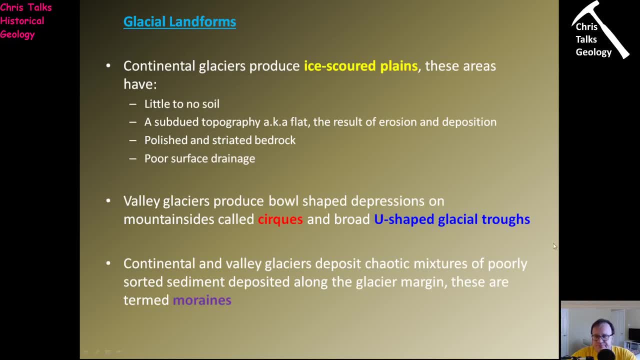 in terms of valley, glaciers, valley in terms of valley, glaciers, valley glaciers will form a couple of glaciers, will form a couple of glaciers, will form a couple of distinct forms. obviously we've already distinct forms. obviously we've already distinct forms. obviously we've already discussed the u-shaped valleys. that's a 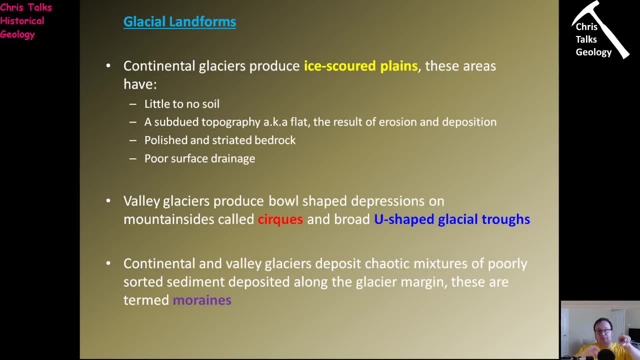 discussed the u-shaped valleys. that's a. discussed the u-shaped valleys. that's a steep valley side either side and a steep valley side either side and a steep valley side either side and a relatively flat bottom in the middle, relatively flat bottom in the middle, relatively flat bottom in the middle, producing that u-shape it will also. 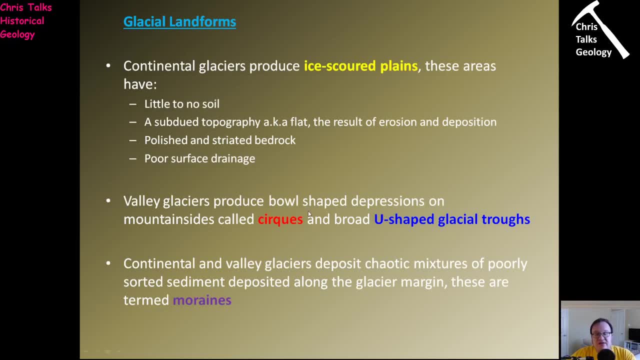 producing that u-shape, it will also producing that u-shape, it will also produce another feature, which are produce another feature, which are produce another feature, which are referred to as circs, and these are small referred to as circs, and these are small referred to as circs, and these are small kind of uh. 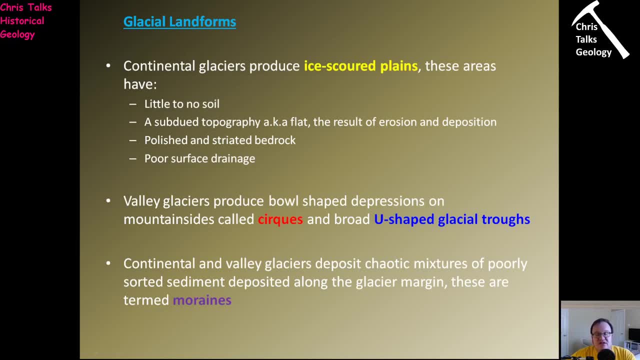 kind of uh. kind of uh. how can i put it? these are small. how can i put it? these are small. how can i put it? these are small depressions in the size inside. sorry of depressions in the size inside. sorry of depressions in the size inside. sorry of the uh topography either side of the. 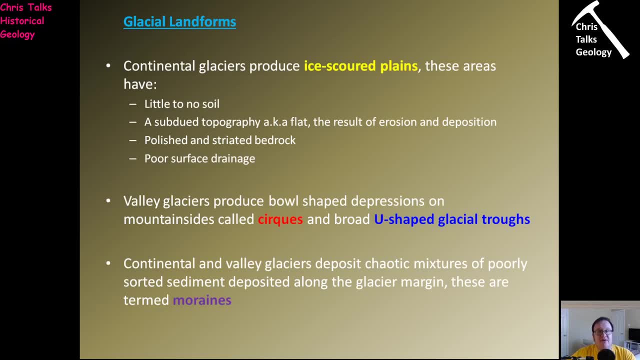 the uh topography, either side of the the uh topography, either side of the of the uh, of the uh, of the uh of the valley glacier. so, if you remember, of the of the valley glacier, so, if you remember, of the of the valley glacier. so, if you remember, the valley glacier is limited to a valley. 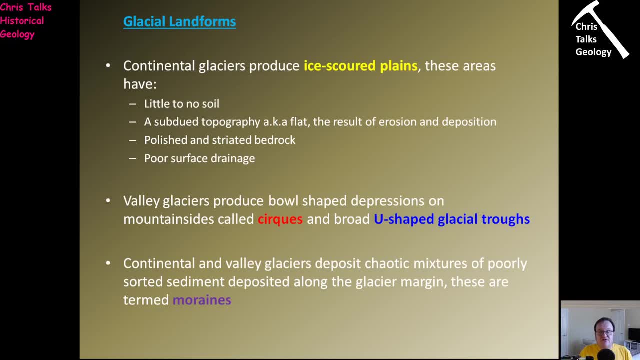 the valley glacier is limited to a valley. the valley glacier is limited to a valley, isn't it? there's high ground either. isn't it there's high ground either? isn't it there's high ground either side side side, now a cirque, essentially is a small. 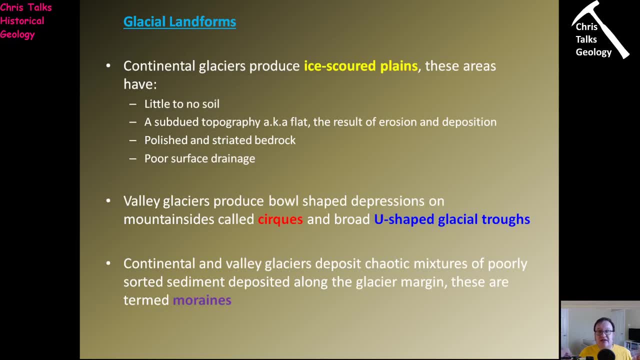 now a cirque, essentially is a small now a cirque, essentially is a small glacier that forms on this high ground glacier. that forms on this high ground glacier. that forms on this high ground typically, you know, typically on the, typically, you know typically on the, typically, you know typically on the sides of a valley glacier. 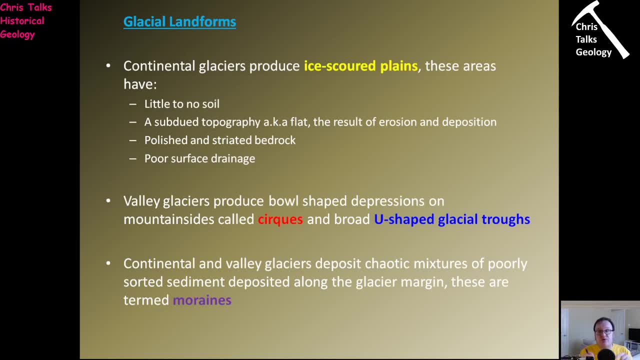 sides of a valley glacier. sides of a valley glacier- okay, and the circle, this kind of cirque, okay, and the circle, this kind of cirque, okay, and the circle, this kind of cirque. glacier will contribute ice to the valley. glacier will contribute ice to the valley. 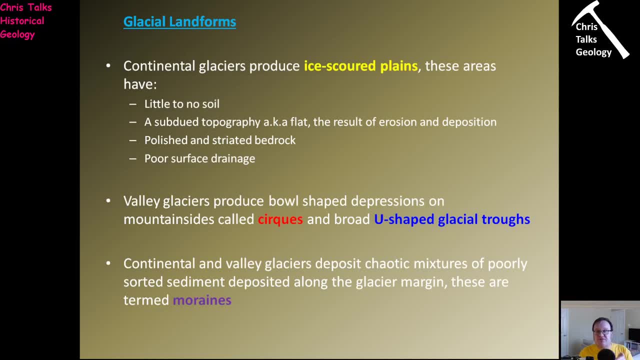 glacier will contribute ice to the valley glacier and the cirque itself will glacier and the cirque itself will glacier and the cirque itself will will be a bowl shaped feature that forms will be a bowl shaped feature that forms will be a bowl shaped feature that forms. okay, think of it kind of like a. 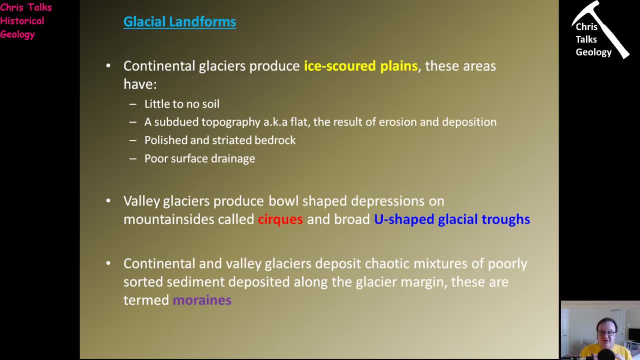 okay, think of it kind of like a. okay, think of it kind of like a tributary going into a river. that's the tributary going into a river. that's the tributary going into a river. that's the kind of same kind of system we have here. 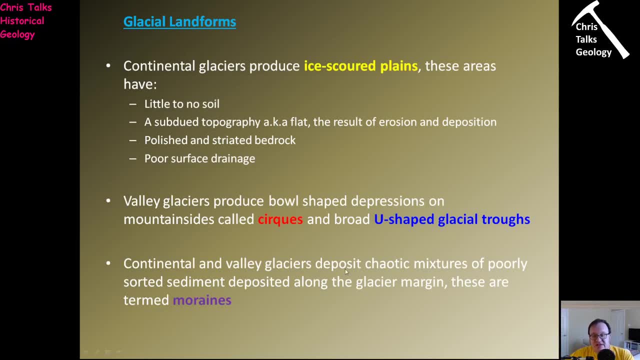 now obviously continental and valley, now obviously continental and valley, now obviously continental and valley. glaciers will deposit this chaotic glaciers will deposit this. chaotic glaciers will deposit this chaotic mixture of sediments right at their front, mixture of sediments right at their front, mixture of sediments right at their front, which we refer to as a moraine. 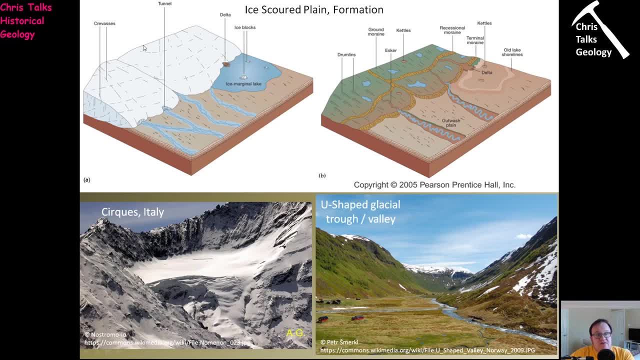 which we refer to as a moraine, which we refer to as a moraine area under here. it's obviously pushing down area under here. it's obviously pushing down area under here. it's obviously pushing down the crust to start with the crust, to start with the crust to start with. it is essentially acting like a bulldozer. 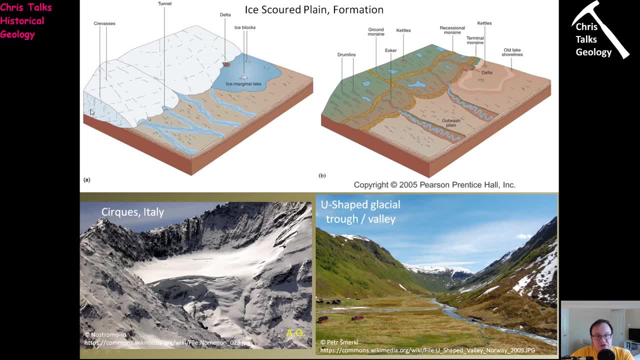 it is essentially acting like a bulldozer. it is essentially acting like a bulldozer. the soil goes, the soil goes, the soil goes. topography gets essentially subdued, gets. topography gets essentially subdued, gets. topography gets essentially subdued, gets, you know, you know, you know, scoured down for one to a better way of. 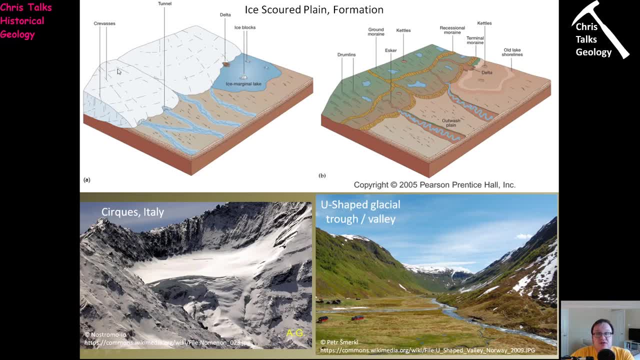 scoured down for one to a better way of scoured down for one to a better way of describing it. describing it, describing it. the rocks themselves become polished. they, the rocks themselves become polished. they, the rocks themselves become polished. they have striations on them, have striations on them. 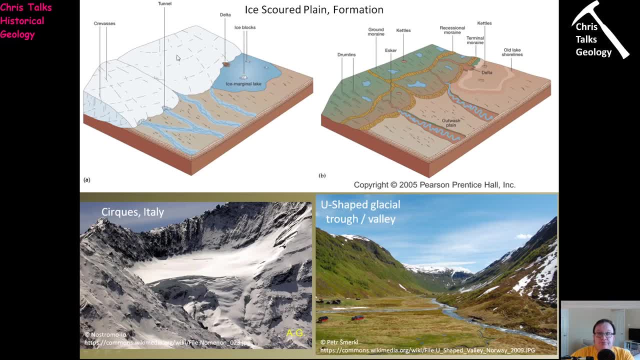 have striations on them, and the sir and the surface drainage is, and the sir and the surface drainage is, and the sir and the surface drainage is very, very poor, very, very poor, very, very poor. okay, and this is what it looks like once. okay, and this is what it looks like once. 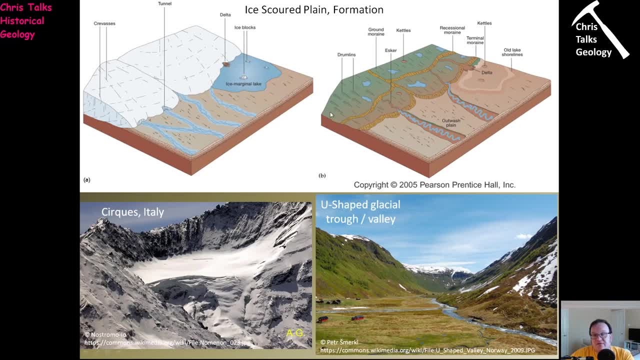 okay, and this is what it looks like- once the ice has gone, so we have our moraines. the ice has gone, so we have our moraines. the ice has gone, so we have our moraines. we have our very, very subdued topography. we have our very, very subdued topography. 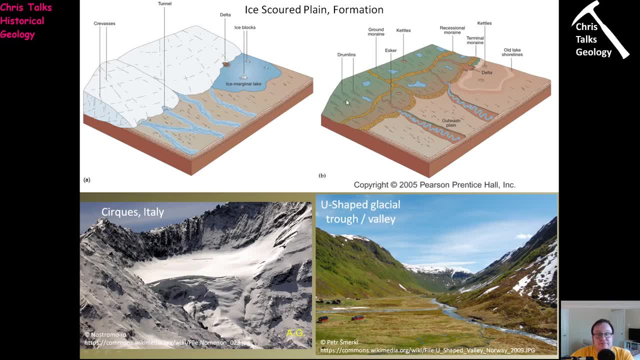 we have our very, very subdued topography and we have water building up on the and we have water building up on the and we have water building up on the surface, surface, surface in terms of the valley glacier. so here's in terms of the valley glacier. so here's. 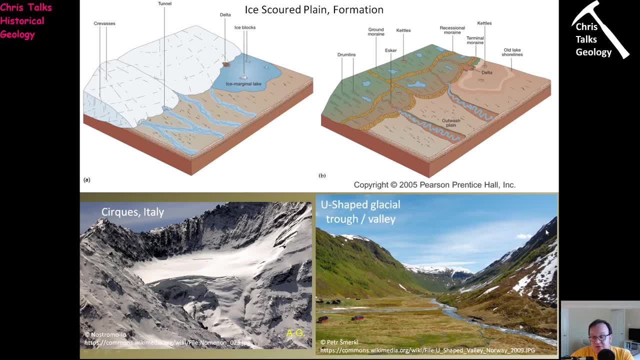 in terms of the valley glacier. so here's a lovely example of a nice u-shaped and this is a circle. you can see it here and this is a circle. you can see it here and this is a circle. you can see it here. so it essentially forms this bowl shaped. 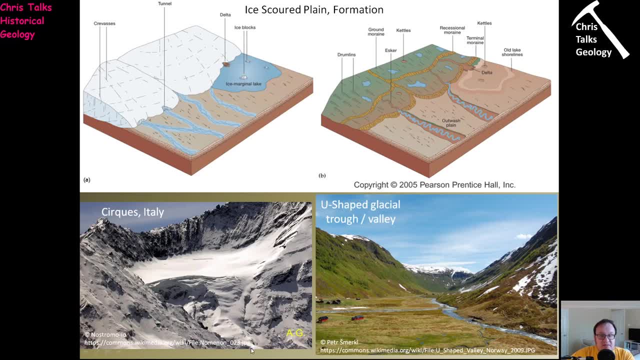 so it essentially forms this bowl shaped. so it essentially forms this bowl shaped, feature, feature, feature and, as you can see, the glacier is and as you can see, the glacier is and as you can see, the glacier is coming down here and there's a very good coming down here and there's a very good. 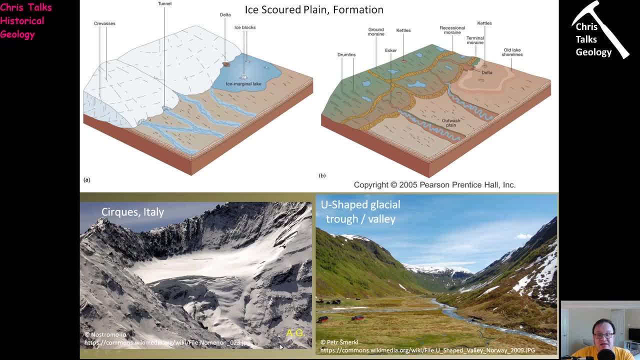 coming down here and there's a very good chance this glacier will actually join. chance, this glacier will actually join chance. this glacier will actually join a larger valley glacier which we can't, a larger valley glacier which we can't, a larger valley glacier which we can't see in the picture. 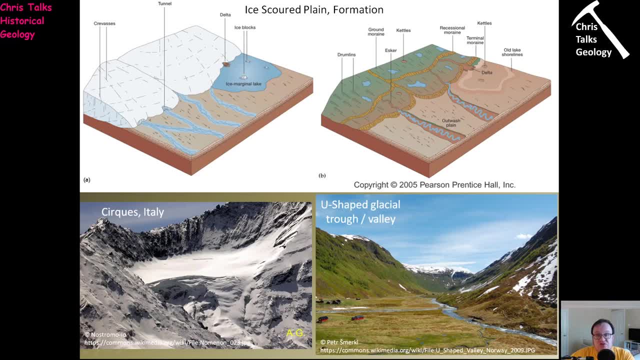 see in the picture. see in the picture. so once again kind of like a tributary. so once again kind of like a tributary. so once again kind of like a tributary joining a much larger river, joining a much larger river, joining a much larger river. so just going back to the ice scoured. 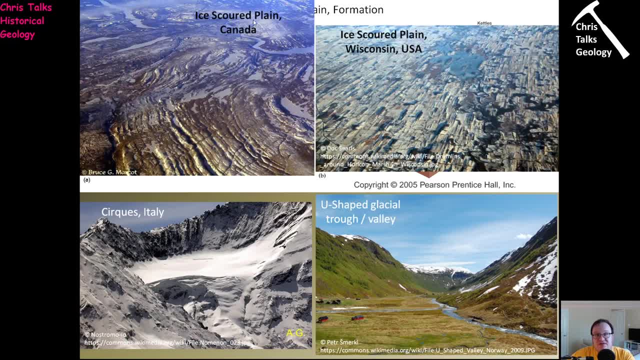 so just going back to the ice scoured. so just going back to the ice scoured: plains for a second, plains for a second, plains for a second. here's a couple of pictures. okay, so this here's a couple of pictures. okay, so this here's a couple of pictures. okay, so this is the ice scour plane. this is an ice. 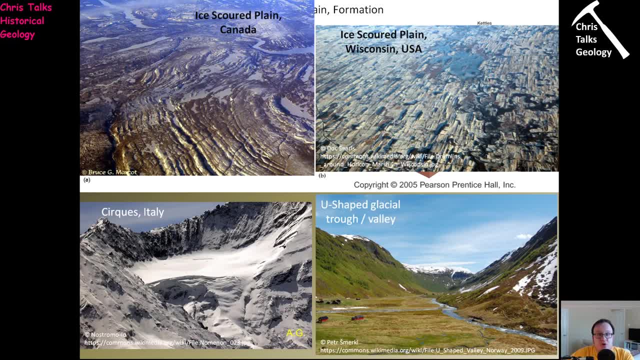 is the ice scour plane. this is an ice is the ice scour plane. this is an ice scour plane in canada. scour plane in canada. scour plane in canada. and this is one from wisconsin, so what? and this is one from wisconsin, so what? and this is one from wisconsin. so what can we see? well, first of all, we can see. 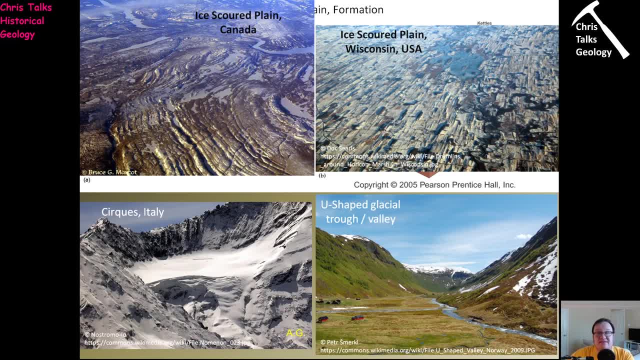 can we see, well, first of all, we can see. can we see, well, first of all we can see. look at that topography, it has been. look at that topography, it has been. look at that topography. it has been planed almost flat, hasn't it? 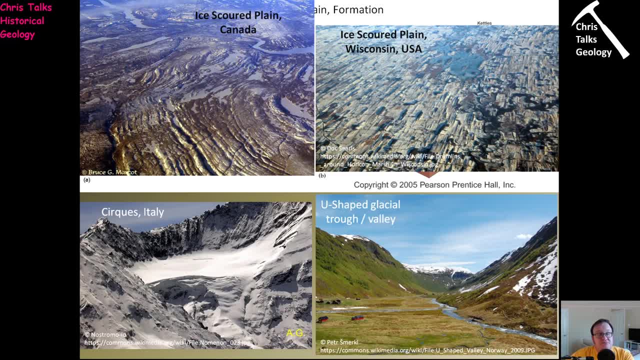 planed almost flat, hasn't it planed almost flat, hasn't it? so topography is non-existent. soil, so topography is non-existent. soil, so topography is non-existent. soil, non-existent, non-existent, non-existent. surface drainage: absolutely terrible you. surface drainage, absolutely terrible you. 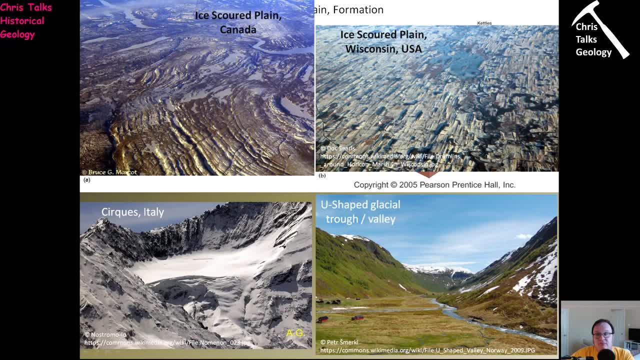 surface drainage- absolutely terrible. you can see that we have. we have a buildup. can see that we have. we have a buildup. can see that we have. we have a buildup of water here. can't we of water here? can't we of water here, can't we? then the question is is: can you see any? 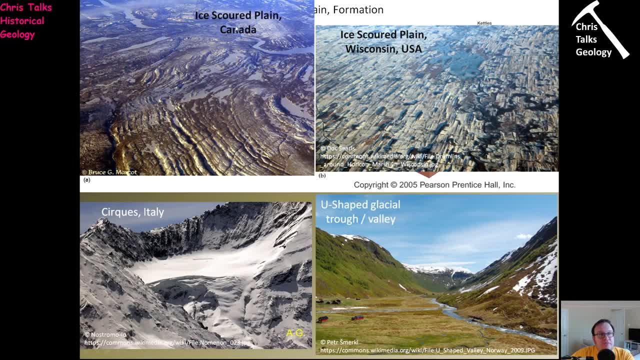 then the question is is: can you see any? then the question is is: can you see any rivers- well, we've got a river here. rivers- well, we've got a river here. rivers- well, we've got a river here, but apart from that, but apart from that, but apart from that, there's nothing draining these bodies of. 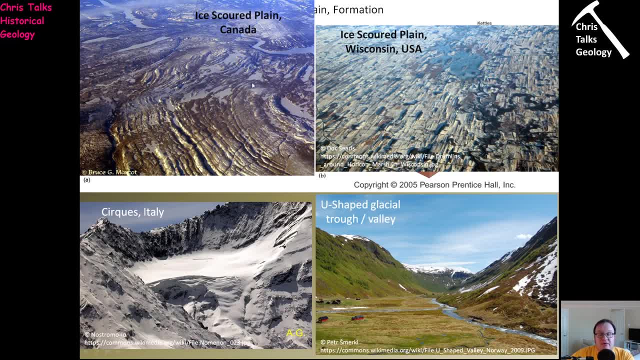 there's nothing draining these bodies of. there's nothing draining these bodies of water. the water just builds up here in water. the water just builds up here in water. the water just builds up here in any depression that it can, any depression that it can, any depression that it can. so you know that's. 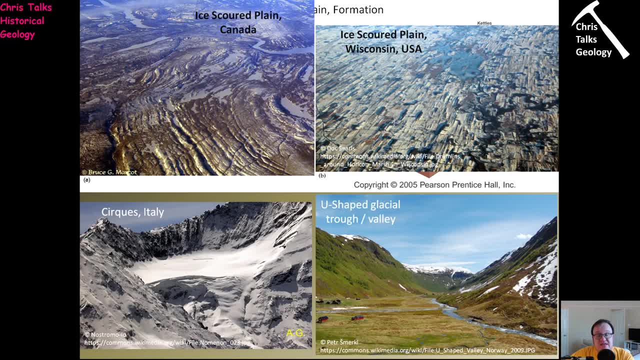 so you know that's. so you know that's pretty much it. the water doesn't really pretty much it. the water doesn't really pretty much it. the water doesn't really escape these areas very, very easily. so escape these areas very, very easily. so escape these areas very, very easily. so it builds up on the surface. 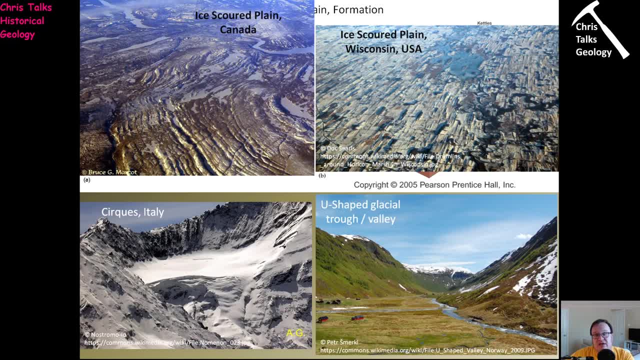 it builds up on the surface. it builds up on the surface. that's why you know areas like canada. that's why you know areas like canada. that's why you know areas like canada and other in the northern plains of, and other in the northern plains of, and other in the northern plains of the northern. 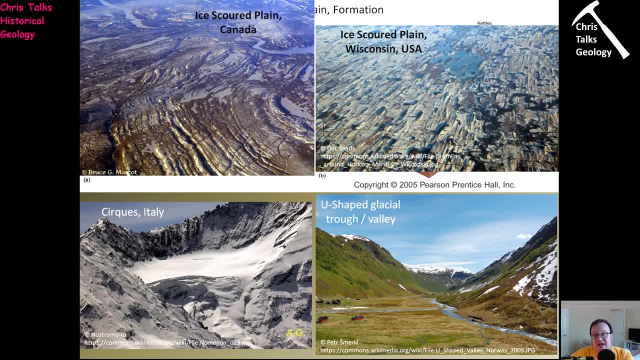 the northern. the northern us states that have been affected by us, states that have been affected by us, states that have been affected by glaciation will tend to have glaciation, will tend to have glaciation, will tend to have quite large lakes associated with them. 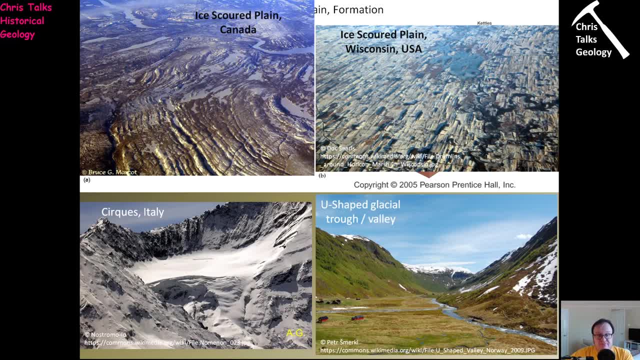 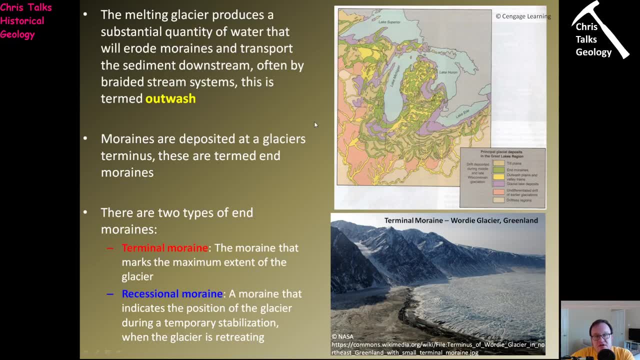 quite large lakes associated with them. quite large lakes associated with them because the water can't go anywhere. it's because the water can't go anywhere. it's because the water can't go anywhere, it's just stuck there. so, in terms of the moraines, well what? 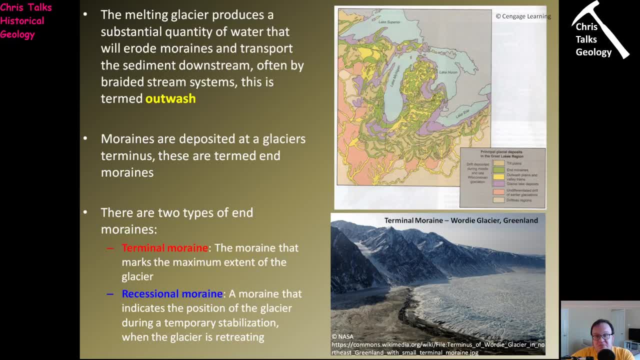 so, in terms of the moraines? well, what so in terms of the moraines? well, what do we see? well, we know the moraine is a build-up. well, we know the moraine is a build-up. well, we know the moraine is a build-up of material. we've discussed that. i'm of material. we've discussed that. i'm of material. we've discussed that. i'm actually just going to go back to the, actually just going to go back to the, actually just going to go back to the previous picture. so if you remember when- previous picture, so if you remember when, 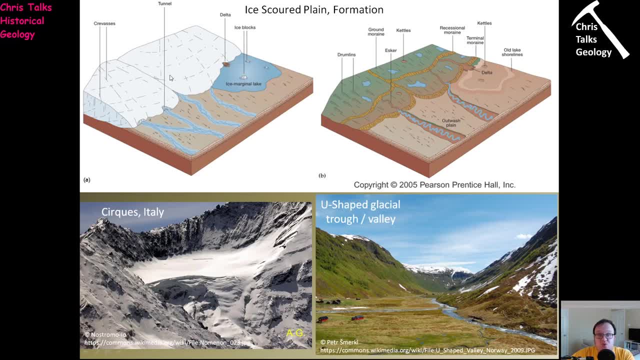 previous picture. so, if you remember, when our, our, our, when our glacier is melting, it's when our glacier is melting, it's when our glacier is melting, it's obviously going to produce quite large, obviously going to produce quite large, obviously going to produce quite large quantities of water. 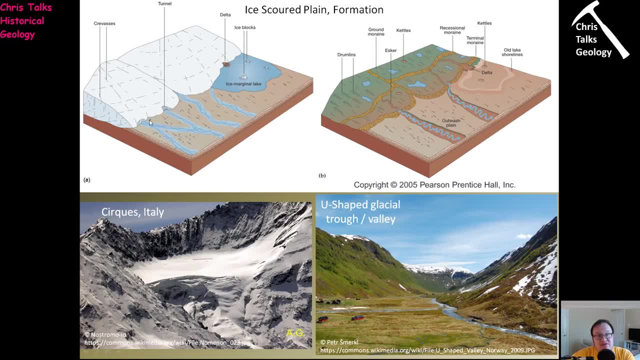 quantities of water. quantities of water, and we have the moraine here along the, and we have the moraine here along the, and we have the moraine here along the front of it, front of it, front of it, and the sediment being deposited which, and the sediment being deposited which. 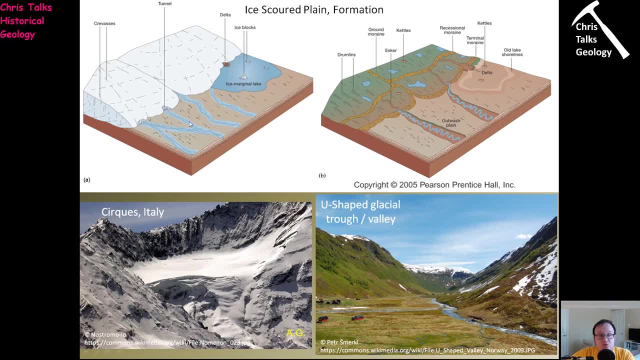 and the sediment being deposited, which makes the moraine will be reworked. washed makes the moraine will be reworked. washed makes the moraine will be reworked. washed away by this water, away by this water, away by this water. okay, and this area in front of the 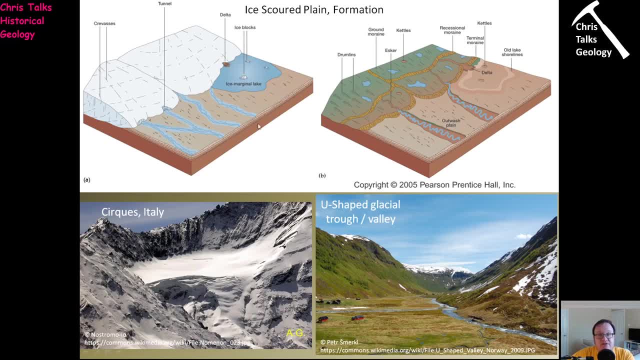 okay, and this area in front of the okay and this area in front of the glacier is referred to as the outwash glacier, is referred to as the outwash glacier is referred to as the outwash plane, plane, plane. this is where sediment being reworked by 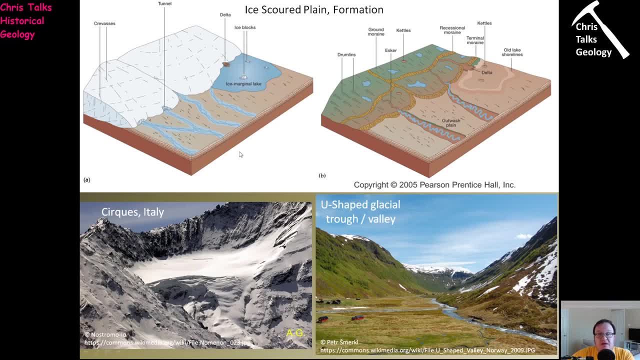 this is where sediment being reworked by, this is where sediment being reworked by the river is essentially distributed. the river is essentially distributed. the river is essentially distributed again. so over here we have the outwash again. so over here we have the outwash again. so over here we have the outwash plane in front of the glacier. 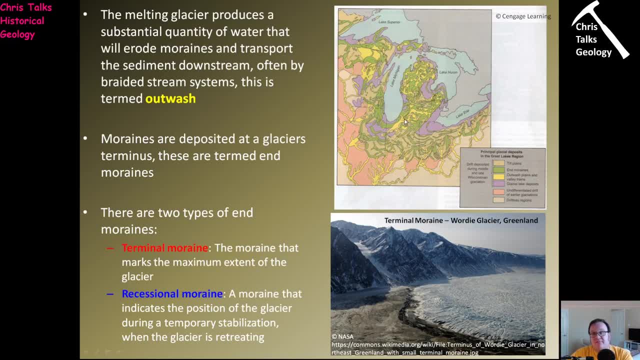 plane in front of the glacier, plane in front of the glacier, so this area is referred to as outwash. so this area is referred to as outwash. so this area is referred to as outwash. now, if we look at this diagram over here. now, if we look at this diagram over here: 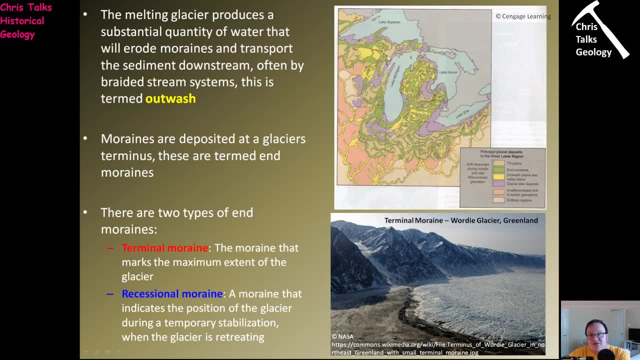 now, if we look at this diagram over here, okay, so this is the diagram, so let's okay, so this is the diagram, so let's okay, so this is the diagram. so let's look at where we are, so we are currently. look at where we are, so we are currently. 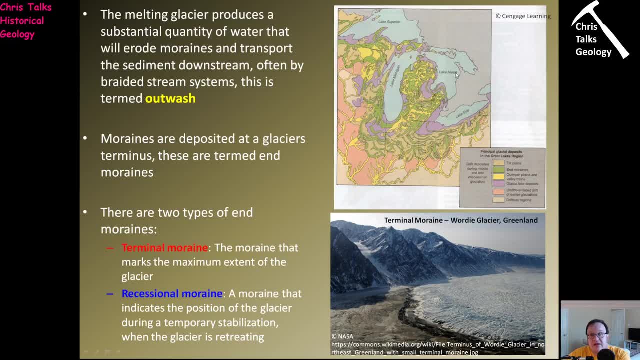 look at where we are. so we are currently in the northern us states. we've got lake in the northern us states. we've got lake in the northern us states. we've got lake michigan right here. okay, lake huron michigan right here. okay, lake huron. 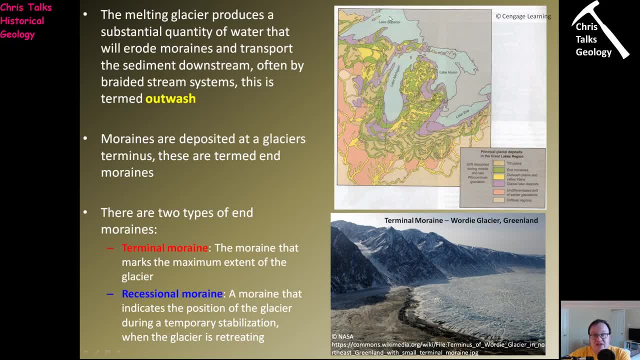 michigan right here, okay, lake huron over here, lake erie here and lake over here, lake erie here and lake over here, lake erie here and lake superior right there. so that should give superior right there, so that should give superior right there. so that should give you some idea of where we are. 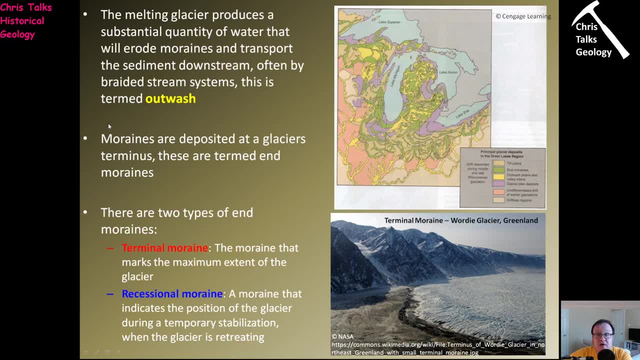 you some idea of where we are? you some idea of where we are? okay, now, the other thing i'm going to. okay, now, the other thing i'm going to. okay, now, the other thing i'm going to keep an eye out for are the moraines. keep an eye out for are the moraines? 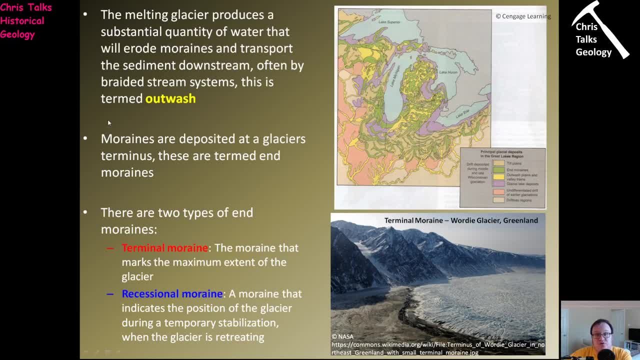 keep an eye out, for are the moraines themselves themselves themselves. okay, remember. and the moraine is okay, remember. and the moraine is okay, remember. and the moraine is caused whenever the glacier pauses caused, whenever the glacier pauses caused, whenever the glacier pauses and deposits sediment. 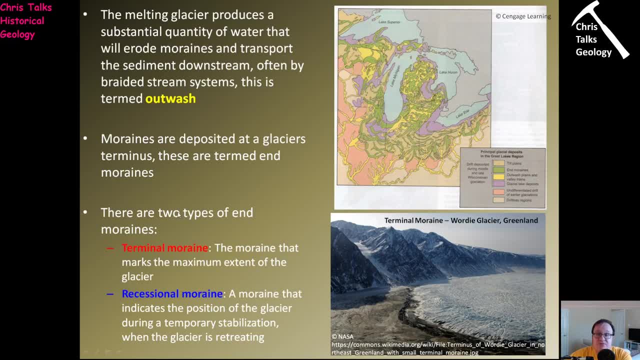 and deposits, sediment and deposits, sediment. okay, okay, okay. so there are two types of moraines, so there are two types of moraines. so there are two types of moraines. the first type of rain is called the. the first type of rain is called the. the first type of rain is called the terminal moraine. 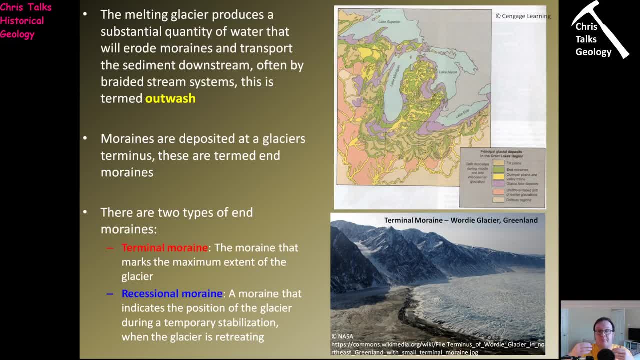 terminal moraine. terminal moraine, now that's produced when the glacier. now that's produced when the glacier. now that's produced when the glacier reaches its reaches, its reaches, its maximum extent, maximum extent, maximum extent. okay, that's as far as the glacier. okay, that's as far as the glacier. 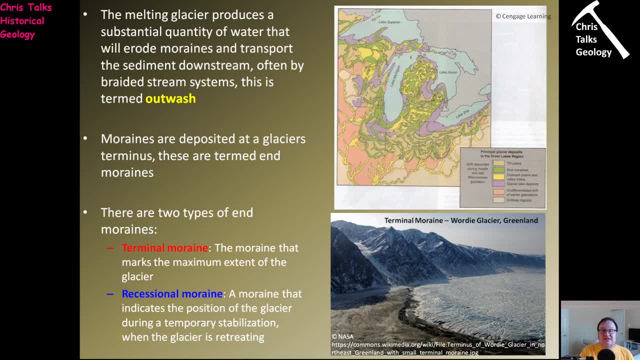 okay, that's as far as the glacier ever made it, ever made it, ever made it. when it reaches its maximum extent, it when it reaches its maximum extent, it when it reaches its maximum extent, it deposits a moraine there and it never. deposits a moraine there and it never. 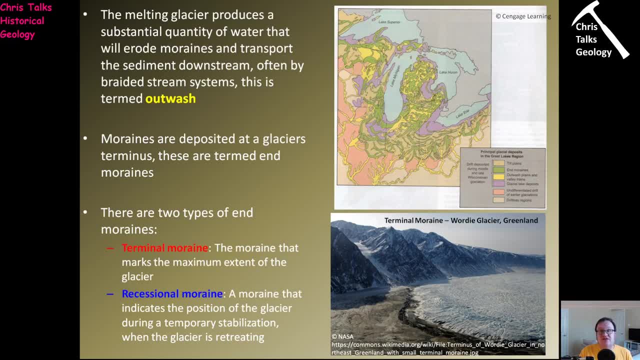 deposits a moraine there and it never goes any further, goes any further, goes any further. from that point on, the only thing, the from that point on the only thing, the from that point on, the only thing the glacier can do is retreat. glacier can do is retreat. 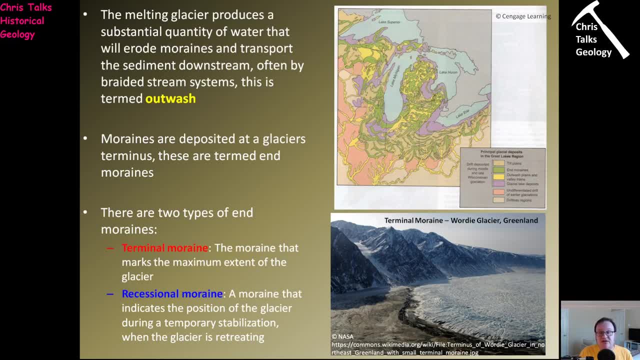 glacier can do is retreat. so then we have what are referred to as so, then we have what are referred to as so. then we have what are referred to as recessional moraines. so as your recessional moraines, so as your recessional moraines, so as your glasses: retreating, it's not a smooth. 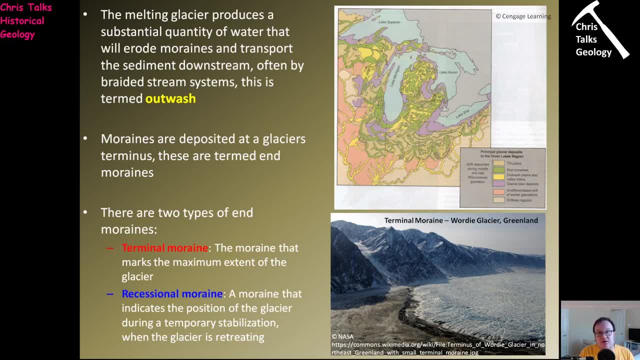 glasses retreating. it's not a smooth glasses retreating. it's not a smooth retreat: retreat, retreat. instead, your glacier will retreat for a. instead, your glacier will retreat for a. instead, your glacier will retreat for a while and stop while, and stop while, and stop, at which point it will form a recessional. 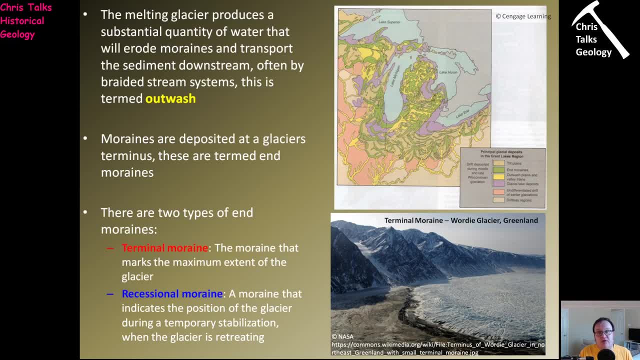 at which point it will form a recessional, at which point it will form a recessional moraine. it will then retreat again moraine. it will then retreat again moraine. it will then retreat again. stop and form another recessional moraine. stop and form another recessional moraine. 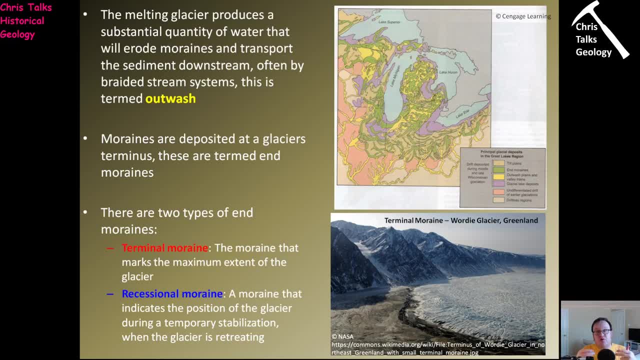 stop and form another recessional moraine. retreat again, retreat again, retreat again. stop form another recessional rain, and so stop form another recessional rain. and so stop form another recessional rain, and so on. so as it retreats, it will form on. so as it retreats, it will form. 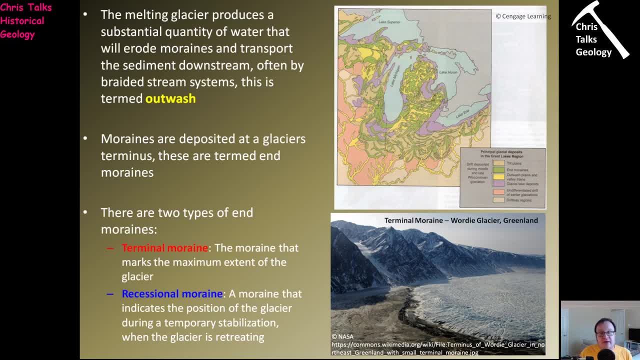 on. so as it retreats, it will form several recessional moraines, several recessional moraines, several recessional moraines. okay, okay, okay. so what we're going to do now is: i'm so. what we're going to do now is: i'm so. what we're going to do now is i'm just going to show you this picture down. 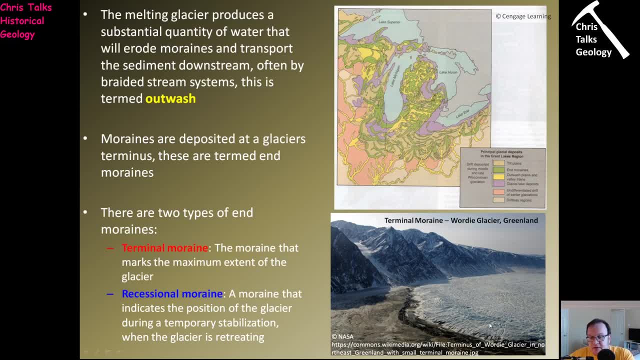 just going to show you this picture down, just going to show you this picture down here. so here's a lovely example. so here's a lovely example. so here's a lovely example. so here's a here's our glacier. here's a here's our glacier. here's a here's our glacier, and you can see right in front of it. 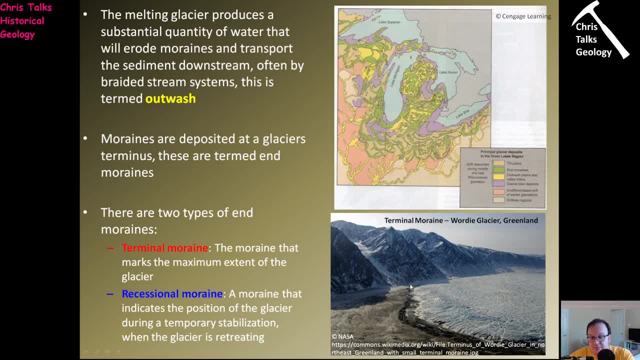 and you can see right in front of it. and you can see right in front of it. there there is the moraine. here is this. there there is the moraine. here is this. there, there is the moraine. here is this. build up of material, build up of material. 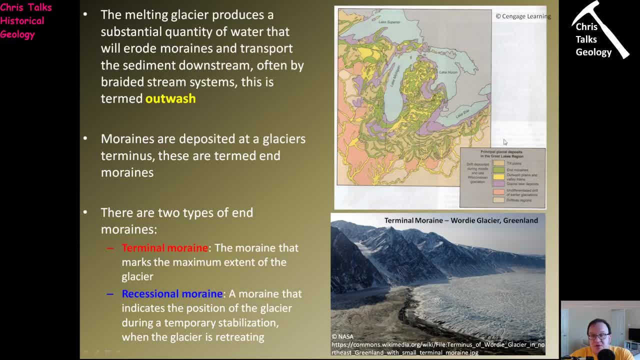 build up of material. okay, okay, okay. now this picture here once again is now this picture here once again, is now this picture here once again- is showing us, showing us, showing us essentially an area around wisconsin, essentially an area around wisconsin, essentially an area around wisconsin, and what we're seeing here is we are. 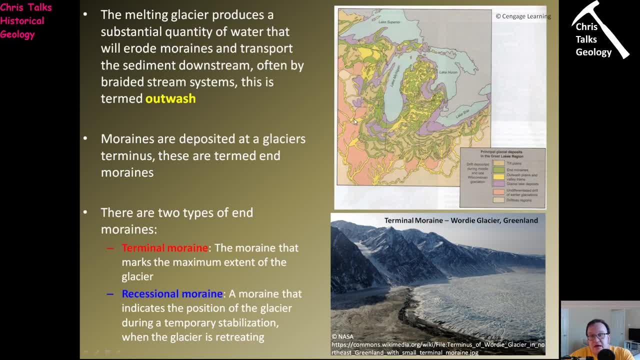 and what we're seeing here is we are, and what we're seeing here is we are seeing, seeing, seeing the lake the great lakes, and we are the lake the great lakes, and we are the lake the great lakes, and we are looking at a geologic map showing 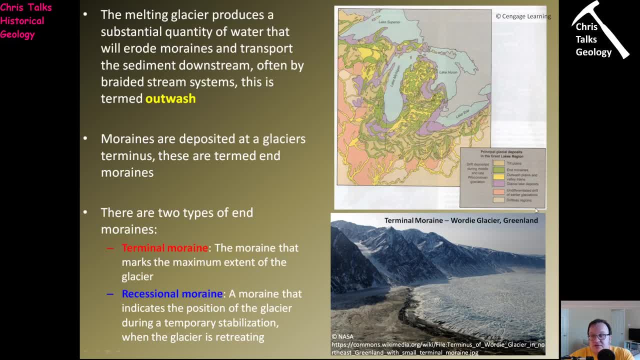 looking at a geologic map showing. looking at a geologic map showing glacial sediment distribution: glacial sediment distribution- glacial sediment distribution. okay, so, okay, so, let's try and work out. okay, so, okay, so, let's try and work out. okay, so, okay, so, let's try and work out what's going on. all right, so? 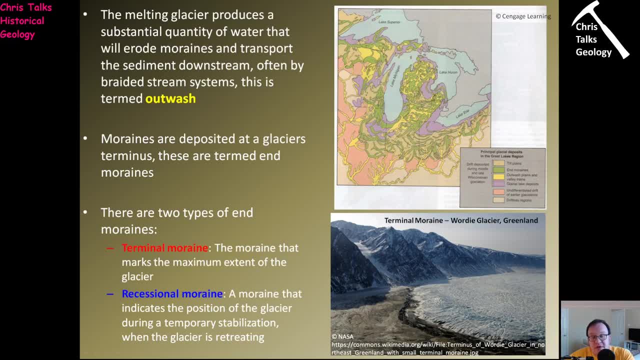 what's going on all right. so what's going on all right? so in yellow: here we have the outwash. in yellow: here we have the outwash. in yellow: here we have the outwash. so remember the outwash forms on this. so remember the outwash forms on this. 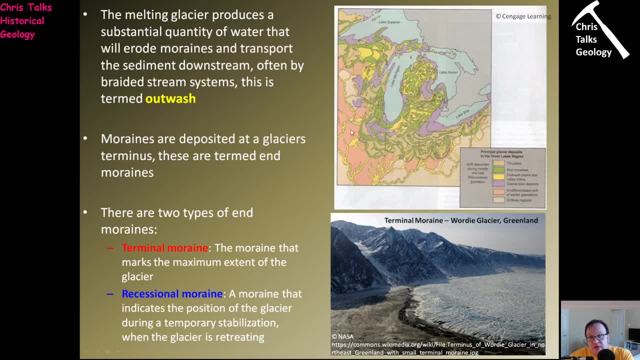 so remember the outwash forms on this front edge of the glacier. so look at front edge of the glacier. so look at front edge of the glacier. so look at where the outwash is located, where the outwash is located, where the outwash is located. okay, 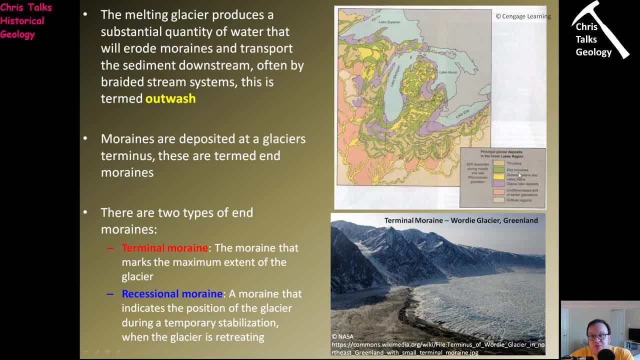 okay, okay, now, now. now we're then going to look at what's. we're then going to look at what's. we're then going to look at what's referred to as the end moraine, so these referred to as the end moraine, so these referred to as the end moraine. so these are the marines that are forming at the 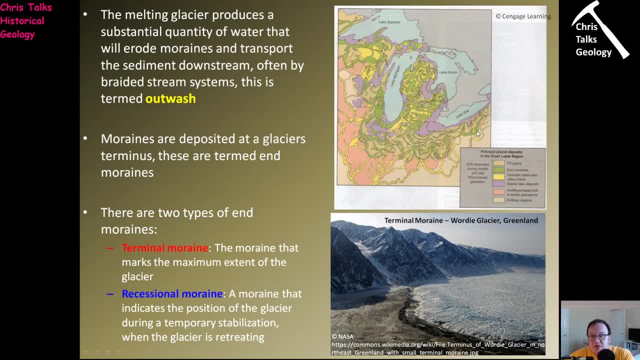 are the marines that are forming at the. are the marines that are forming at the end of the glacier? now look carefully. end of the glacier- now look carefully. end of the glacier, now look carefully. look. this is where. look, this is where. look, this is where the moraines 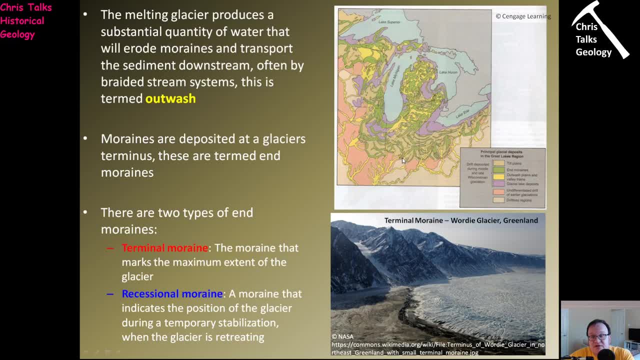 the moraines. the moraines are reaching their maximum extent? isn't are reaching their maximum extent? isn't are reaching their maximum extent, isn't it? yes it, yes it, yes. so these are going to be the terminal. so these are going to be the terminal. so these are going to be the terminal moraines. 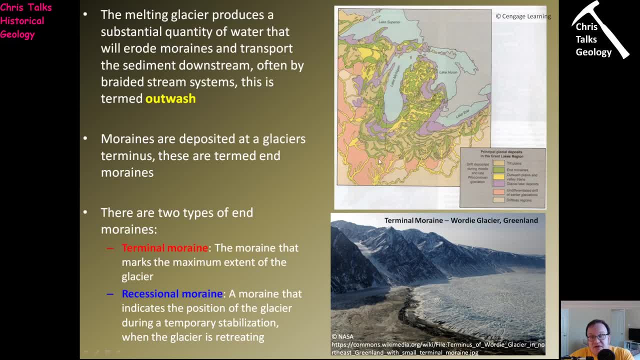 moraines, moraines for the ice sheet. that's as far as it for the ice sheet. that's as far as it for the ice sheet. that's as far as it ever reached, ever reached, ever reached. now, look, this also corresponds quite. now, look, this also corresponds quite. 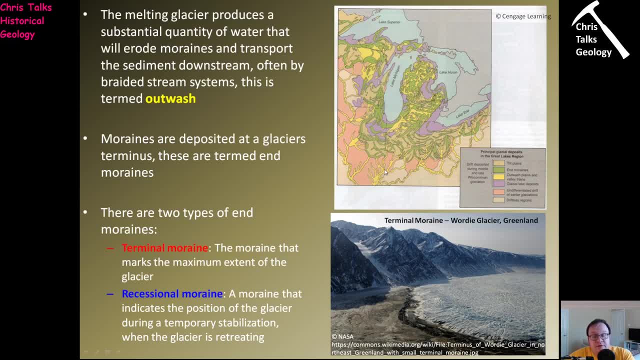 now look, this also corresponds quite nicely with the outwash planes, doesn't nicely with the outwash planes, doesn't nicely with the outwash planes, doesn't it? it it okay. remember the outwash planes. is okay, remember the outwash planes is okay. remember the outwash planes. is depositing all this undifferentiated. 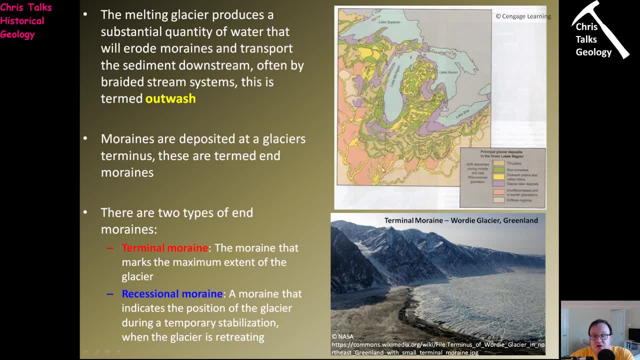 depositing all this undifferentiated. depositing all this undifferentiated stuff which is here in pink stuff, which is here in pink stuff, which is here in pink, okay, so we can see these essentially okay, so we can see these essentially okay, so we can see these essentially looks quite reasonable. 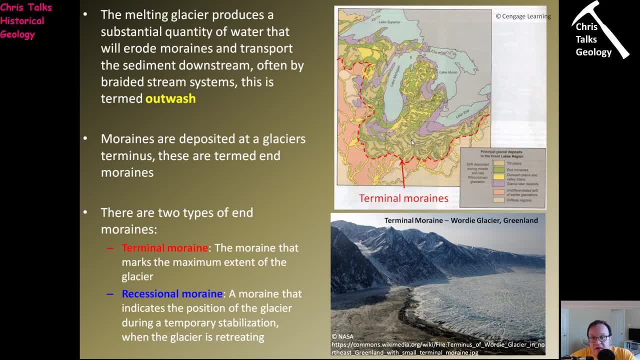 looks quite reasonable, looks quite reasonable now, then you'll notice. if you look here now, then you'll notice. if you look here now, then you'll notice. if you look here, for instance, we have one moraine, for instance, we have one moraine, for instance, we have one moraine followed by another moraine, followed by. 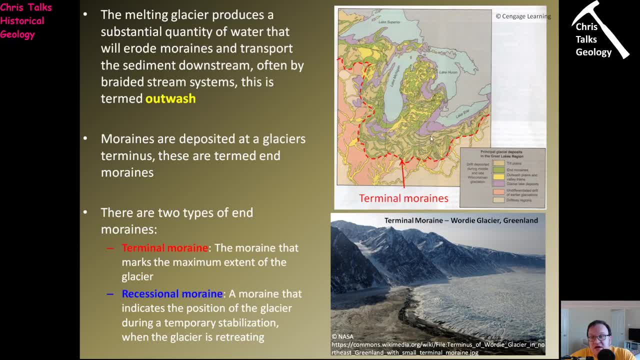 followed by another moraine, followed by: followed by another moraine, followed by another moraine, another moraine, followed by another moraine, another moraine, followed by another moraine. so these are the recessional moraines. so these are the recessional moraines. so these are the recessional moraines. okay, produced as the glaciers. 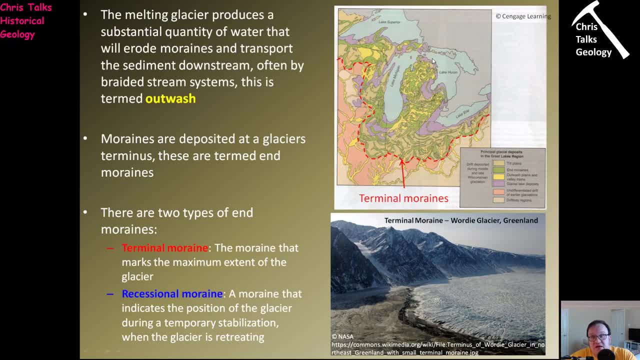 okay, produced as the glaciers. okay, produced as the glaciers retreating along now, obviously, as you retreating along now, obviously, as you retreating along now, obviously, as you can quite clearly see here, can quite clearly see here, can quite clearly see here, a lot of this stuff is extremely chaotic. a lot of this stuff is extremely chaotic. a lot of this stuff is extremely chaotic. you can it's very difficult to work out. you can. it's very difficult to work out. you can. it's very difficult to work out what's going on. what's going on. 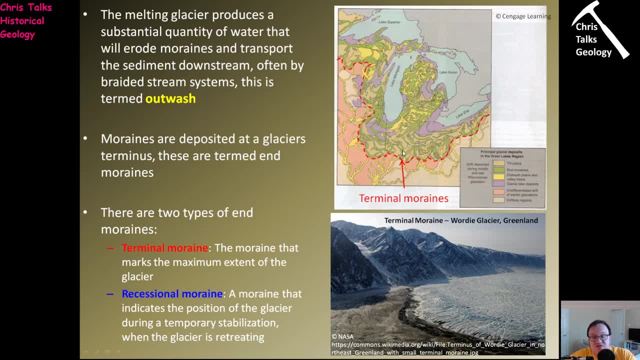 what's going on. but this area down here is particularly, but this area down here is particularly, but this area down here is particularly nice in showing us these recessional nice, in showing us these recessional nice, in showing us these recessional moraines as the glacier is retreating. 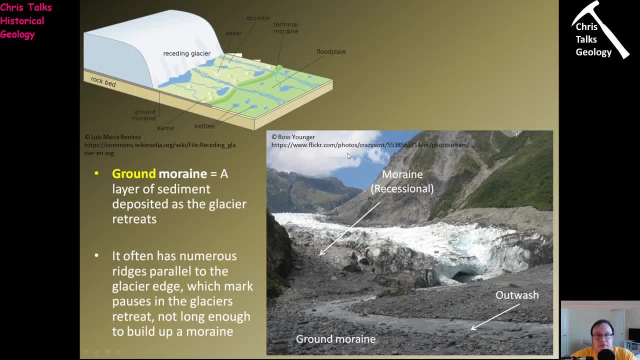 moraines as the glacier is retreating. moraines as the glacier is retreating, okay, so, so, so we've already gone and discussed this. so we've already gone and discussed this. so we've already gone and discussed this. so, as our glacier retreats, we have our 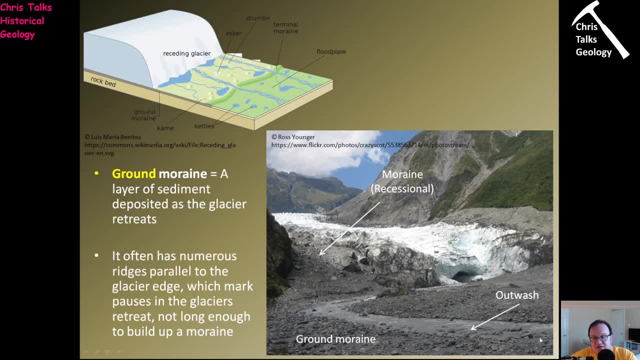 as our glacier retreats. we have our as our glacier retreats. we have our moraine forming. we have our outwash here, moraine forming. we have our outwash here, moraine forming. we have our outwash here. you can see it in this picture here. so 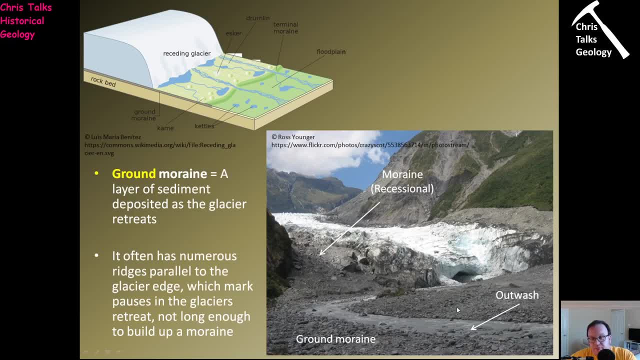 you can see it in this picture here. so you can see it in this picture here. so this is the sediment being redistributed. this is the sediment being redistributed. this is the sediment being redistributed from the moraine, from the moraine, from the moraine. now, this is our recessional moraine right. 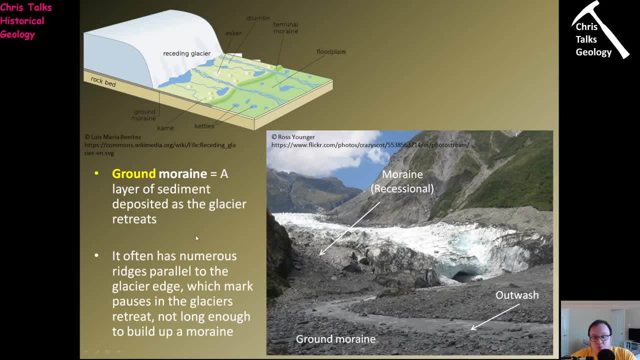 now. this is our recessional moraine right now. this is our recessional moraine right here. it's actually not a particularly here. it's actually not a particularly here, it's actually not a particularly great one. great one, great one. but there is one more type of moraine. 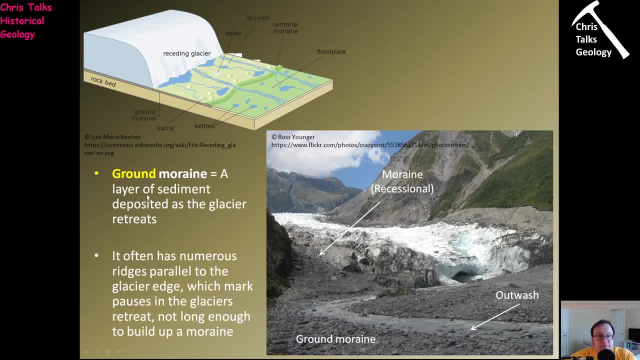 but there is one more type of moraine. but there is one more type of moraine which we need to discuss, and it's which we need to discuss, and it's which we need to discuss and it's referred to as a ground moraine. referred to as a ground moraine. 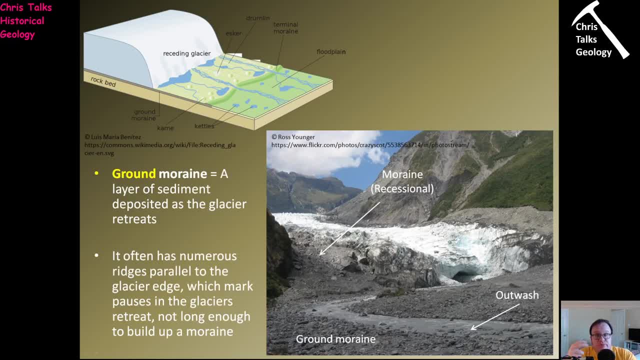 referred to as a ground moraine. so a ground moraine is simply the. so a ground moraine is simply the. so a ground moraine is simply the sediment deposited as the glacier sediment, deposited as the glacier sediment, deposited as the glacier retreats, retreats, retreats, so as the glacier is retreating and it's 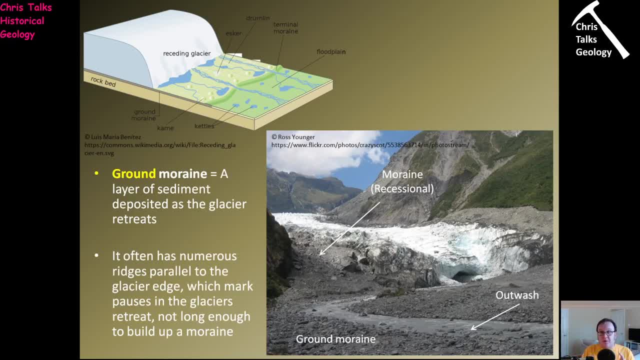 so as the glacier is retreating. and it's so as the glacier is retreating and it's moving, moving, moving. remember if it needs to stop to form a remember if it needs to stop to form a, remember if it needs to stop to form a moraine, because it needs to, it needs to. 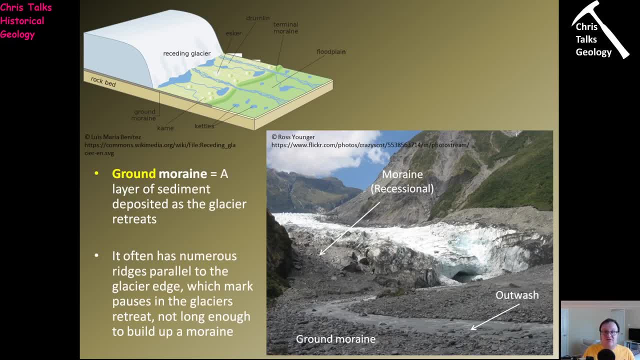 moraine because it needs to. it needs to moraine because it needs to, it needs to build up sediment. but if the glacier is build up sediment, but if the glacier is build up sediment, but if the glacier is moving, it can't, you know, it can't build. 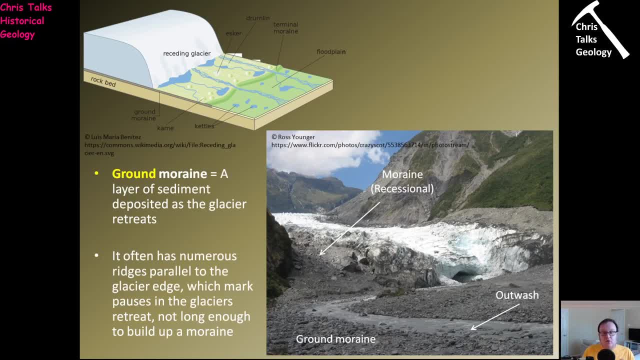 moving it can't you know it can't build. moving it can't you know it can't build up a hill of sediment. can it up a hill of sediment? can it up a hill of sediment, can it so? instead, all that happens is as the so instead, all that happens is as the 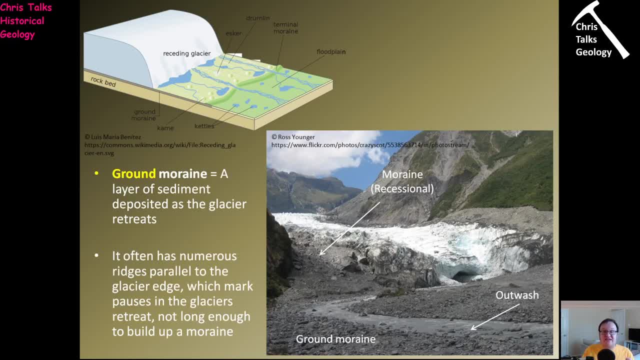 so instead, all that happens is, as the glacier retreats, it simply deposits a glacier retreats. it simply deposits a glacier retreats. it simply deposits a blanket of sediment as it goes. blanket of sediment as it goes, blanket of sediment as it goes, and it's blanket of sediment that it. 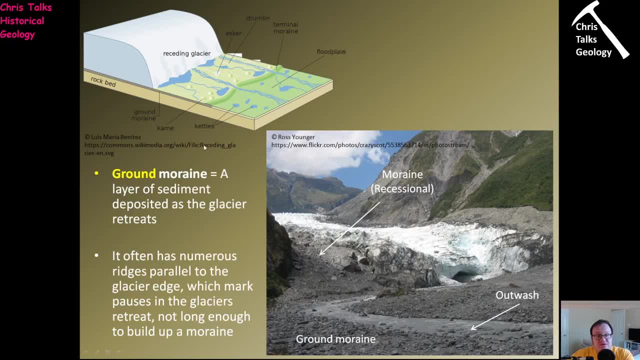 and it's blanket of sediment that it and it's blanket of sediment that it deposits as it retreats when it's moving. deposits as it retreats when it's moving. deposits as it retreats when it's moving, remember, is referred to as a ground. deposits as it retreats when it's moving, remember, is referred to as a ground. 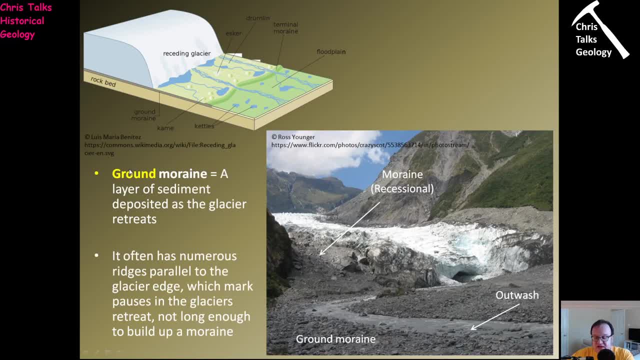 deposits as it retreats when it's moving, remember, is referred to as a ground moraine, moraine moraine, okay, so a ground moraine forms when the okay. so a ground moraine forms when the okay. so a ground moraine forms when the glacier is moving. 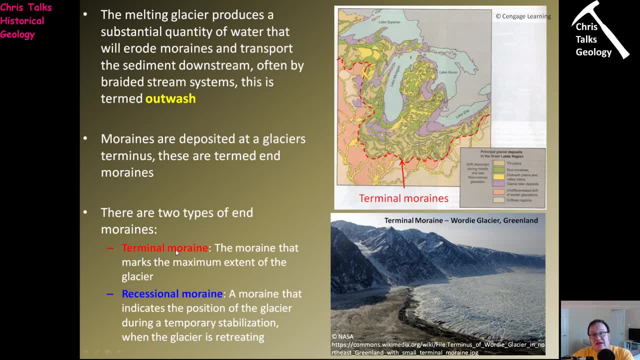 glacier is moving. glacier is moving whereas recessional marines and terminal, whereas recessional marines and terminal, whereas recessional marines and terminal, rains can only form when the glacier rains can only form, when the glacier rains can only form when the glacier is still, is still. 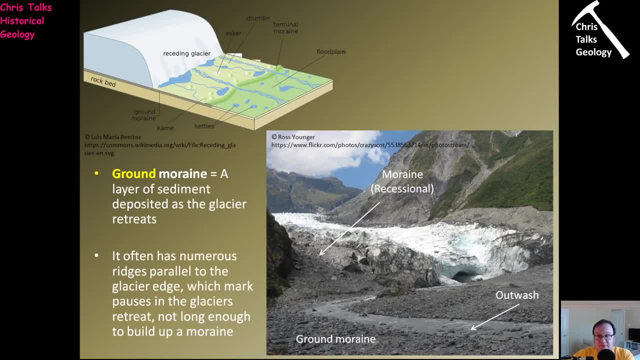 is still all right. so all right, so all right. so there we go there, we go there, we go. perfect that pretty much covers. you know, perfect, that pretty much covers. you know, perfect, that pretty much covers. you know the the general, you know things, we will. the the general, you know things, we will. 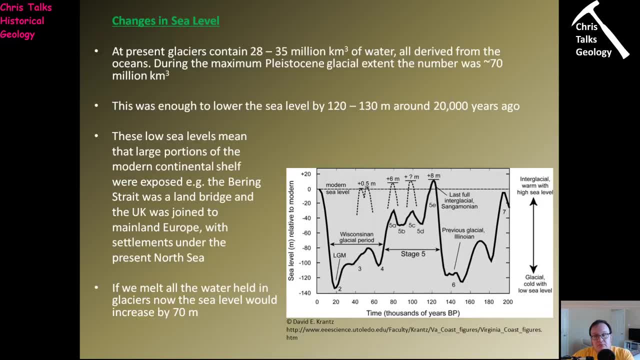 the, the general. you know things we will see when we look at glasses in terms of see, when we look at glasses in terms of see, when we look at glasses in terms of the morphology. so another thing we need to think about. so another thing we need to think about. 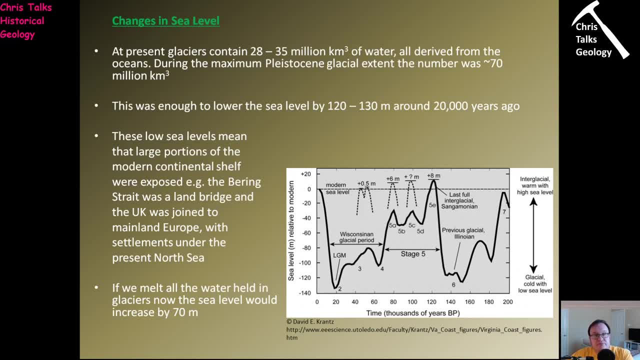 so another thing we need to think about are the changes in sea level that we see. are the changes in sea level that we see? are the changes in sea level that we see now remember? changes in sea level are now remember. changes in sea level are now remember. changes in sea level are very often associated with glaciation, if 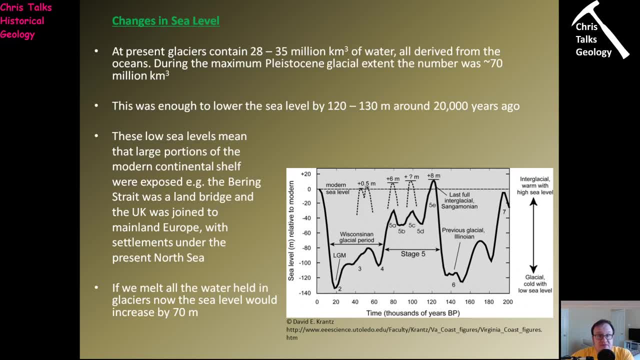 very often associated with glaciation, if very often associated with glaciation. if we have a lot of glaciers, that means we have a lot of glaciers. that means we have a lot of glaciers. that means lots of water is locked up in in ice, and lots of water is locked up in in ice and 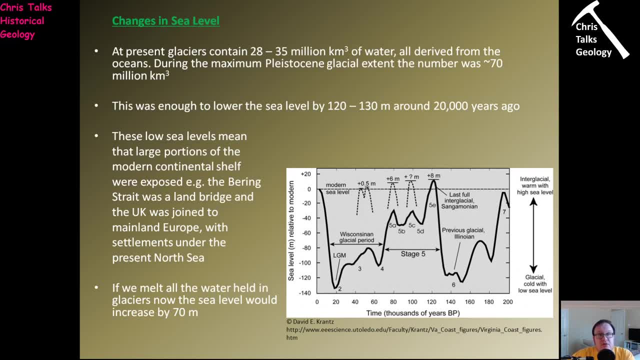 lots of water is locked up in in ice, and so the sea level will drop, won't it? so the sea level will drop, won't it? so the sea level will drop, won't it? so? at present, glaciers contain about 28, so at present, glaciers contain about 28. 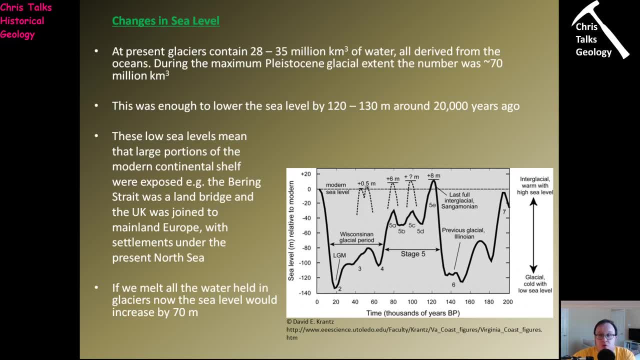 so at present, glaciers contain about 28 to 35 million cubic kilometers of water to 35 million cubic kilometers of water. to 35 million cubic kilometers of water. and now all that water comes from the. and now all that water comes from the and now all that water comes from the oceans. okay, 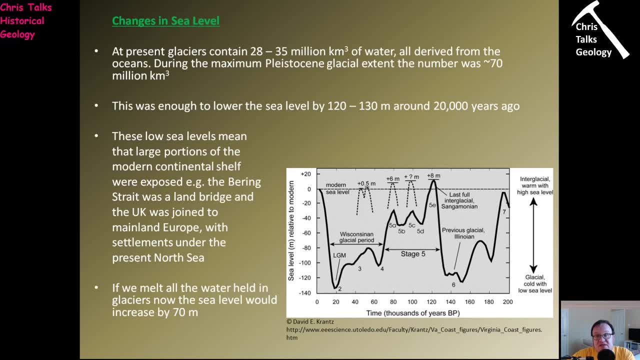 oceans, okay, oceans okay, so, so, so, during the maximum pleistocene glacial, during the maximum pleistocene glacial, during the maximum pleistocene glacial extent: the number was approximately 70 extent. the number was approximately 70 extent. the number was approximately 70 million. 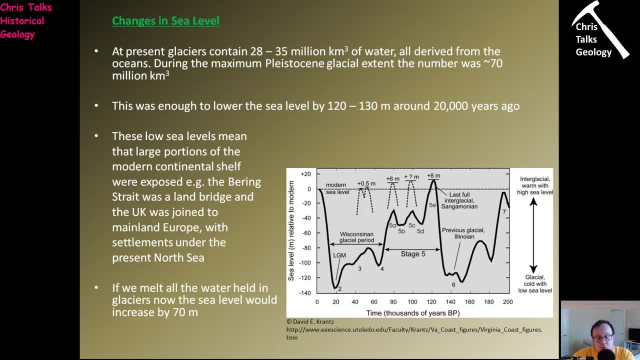 million million cubic kilometers. so you can see that's a cubic kilometers. so you can see that's a cubic kilometers. so you can see that's a lot more ice, a lot more water. sorry, has lot more ice, a lot more water. sorry, has lot more ice, a lot more water. sorry, has been removed from the oceans. 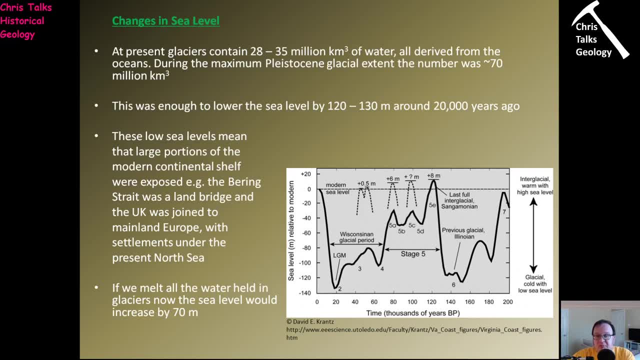 been removed from the oceans, been removed from the oceans, so this would have been enough to to, so this would have been enough to to, so this would have been enough to to lower the ocean sea levels by about 120: lower the ocean sea levels by about 120. 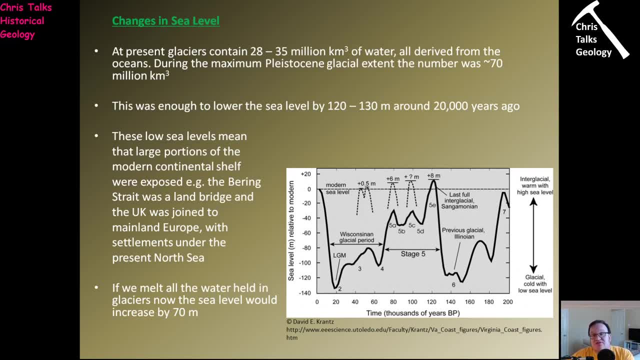 lower the ocean sea levels by about 120 to 130 meters for around 20 000 years to 130 meters for around 20 000 years to 130 meters for around 20 000 years. so that is a pretty big amount of water. 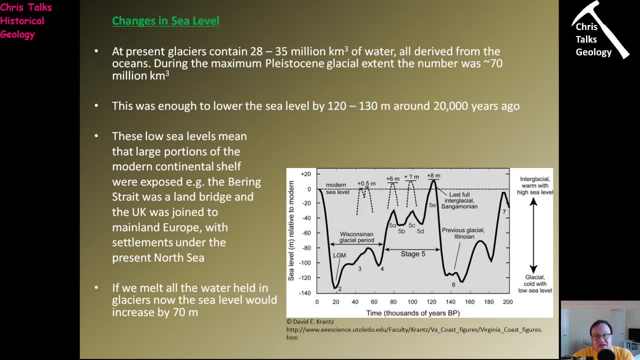 so that is a pretty big amount of water. so that is a pretty big amount of water. amount of water lost: that's a pretty big amount of water lost. that's a pretty big amount of water lost. that's a pretty big drop in sea level. drop in sea level. 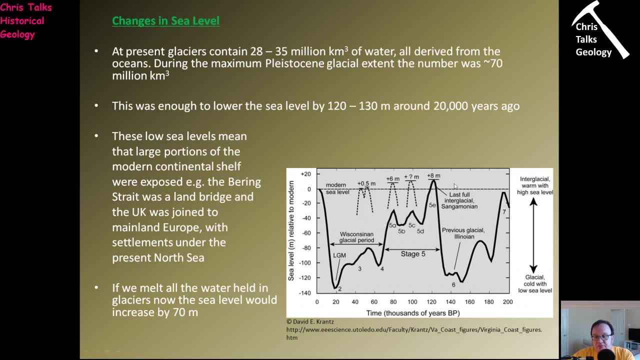 drop in sea level. so if we look at this diagram here, so if we look at this diagram here, so if we look at this diagram here, what can we see? well, here's the sea. what can we see? well, here's the sea. what can we see? well, here's the sea level relative to modern. so zero is the 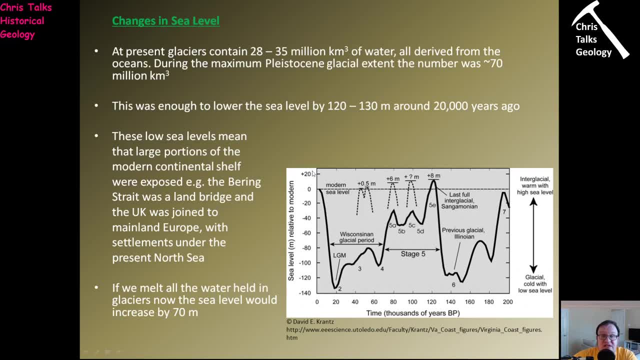 level relative to modern. so zero is the level relative to modern, so zero is the the present day sea level. the present day sea level, the present day sea level. so plus 20 as the sea level goes up. and so plus 20 as the sea level goes up. and 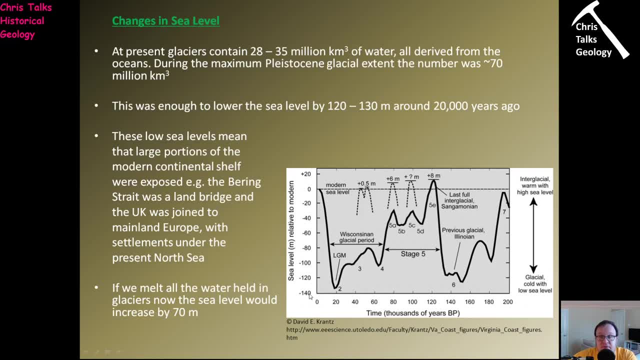 so plus 20 as the sea level goes up. and all these negative figures are saying. all these negative figures are saying all these negative figures are saying the sea level is going down, the sea level is going down, the sea level is going down. so what do we notice? well, okay, so what do we notice? well, okay. so what do we notice? well, okay. so right here we have the wisconsin. so right here we have the wisconsin, so right here we have the wisconsin glacial period. so if you remember that glacial period, so if you remember that, 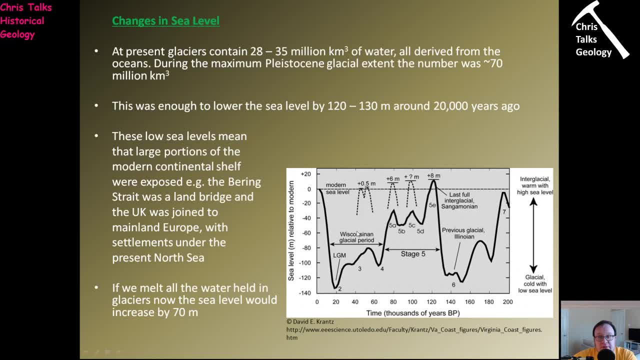 glacial period. so, if you remember, that was one of the very that was the most, was one of the very that was the most, was one of the very that was the most recent one, recent one, recent one, okay, and here we have. okay, and here we have. 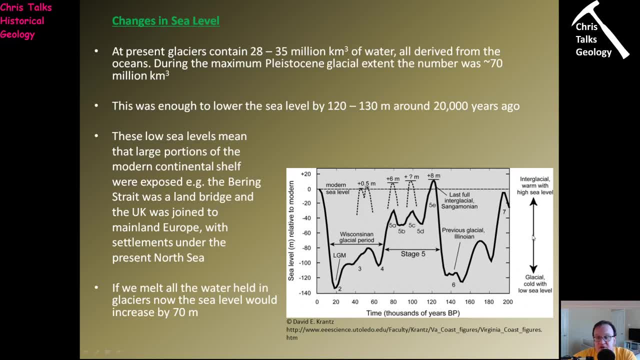 okay, and here we have an illinoinian glacial period, right, an illinoinian glacial period. right, an illinoinian glacial period, right here, here, here. so what you'll notice is here we go. so what you'll notice is here we go. 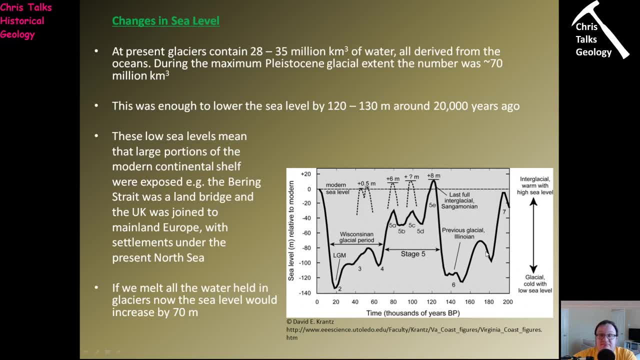 so what you'll notice is, here we go. glacial period- all of a sudden sea level. glacial period- all of a sudden sea level. glacial period: all of a sudden sea level plummets down, doesn't it plummets down? doesn't it plummets down? doesn't it not really a huge shock there, as soon as? 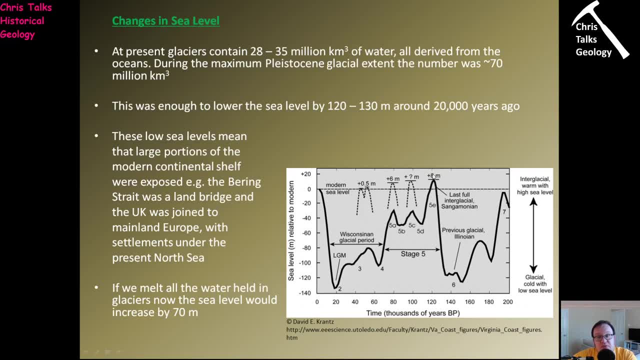 not really a huge shock there as soon as not really a huge shock there. as soon as we enter an interglacial ice melt sea. we enter an interglacial ice melt sea. we enter an interglacial ice melt sea. level goes up. level goes up. 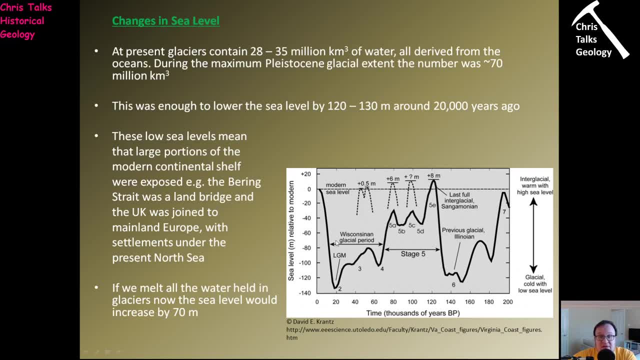 level goes up, and then as soon as we enter another, and then as soon as we enter another, and then as soon as we enter another, glacial sea level goes down again. glacial sea level goes down again. glacial sea level goes down again. so not really a huge surprise there. 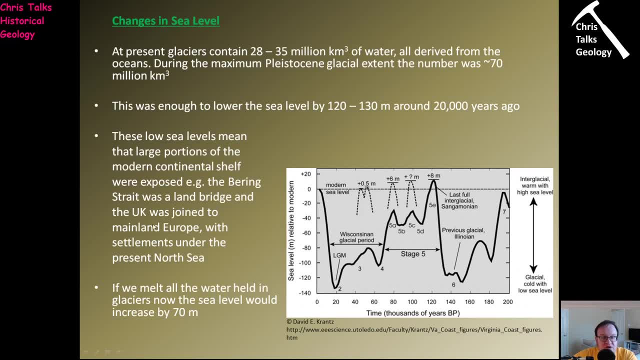 so not really a huge surprise there. so not really a huge surprise there. so there's a little bit of a blurb here. so there's a little bit of a blurb here. so there's a little bit of a blurb here about, you know, about, archaeology in the. 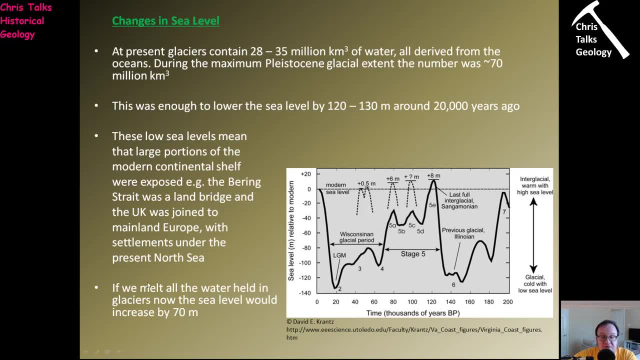 about you know about archaeology in the, about you know about archaeology in the uk, but that's not really that important uk, but that's not really that important uk, but that's not really that important. okay, so if we melt all the water held in. okay, so if we melt all the water held in. 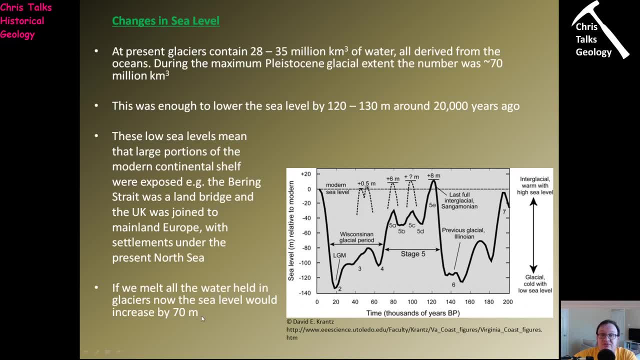 okay. so if we melt all the water held in glaciers- at the moment it's going to glaciers at the moment it's going to glaciers. at the moment it's going to see a sea level increase of about 70. see a sea level increase of about 70. 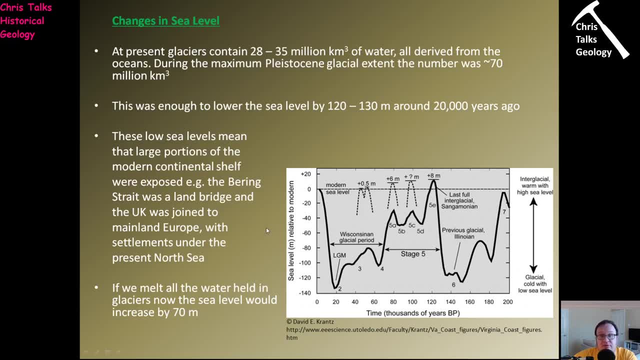 see a sea level increase of about 70 meters. that gives you some idea of you meters. that gives you some idea of you meters. that gives you some idea of you know of what can happen. now, another effect of the glaciation. now another effect of the glaciation. 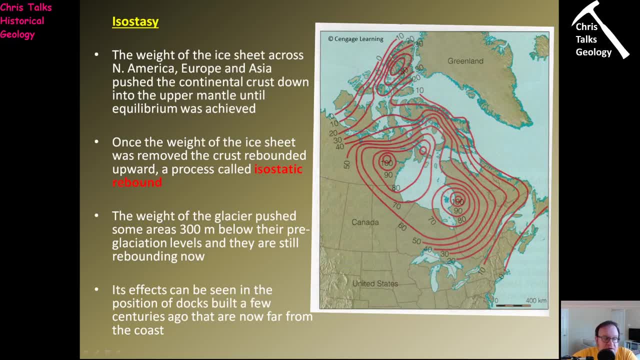 now. another effect of the glaciation that we see now is something called that we see now is something called. that we see now is something called isostasy, isostasy, isostasy. so, if you remember, we've discussed how. so, if you remember, we've discussed how. 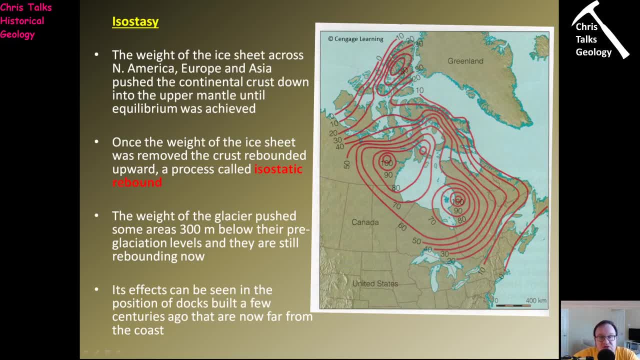 so, if you remember, we've discussed how the weight of the ice, the weight of the ice, the weight of the ice, would push down the continental crust, would push down the continental crust, would push down the continental crust. that's all. it's just the sheer weight. that's all. it's just the sheer weight. 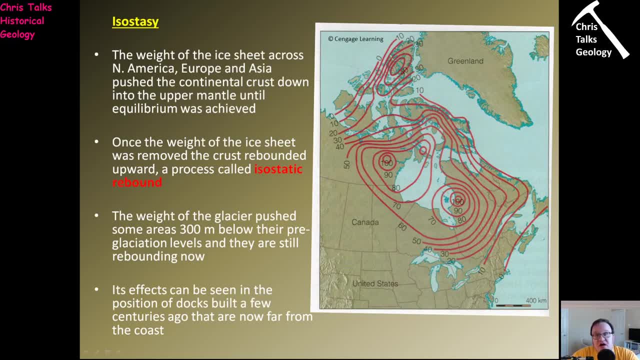 that's all. it's just the sheer weight of the ice can do this, of the ice can do this, of the ice can do this. so obviously, once the ice sheet is so obviously, once the ice sheet is so obviously, once the ice sheet is removed, well, the crust is going to. 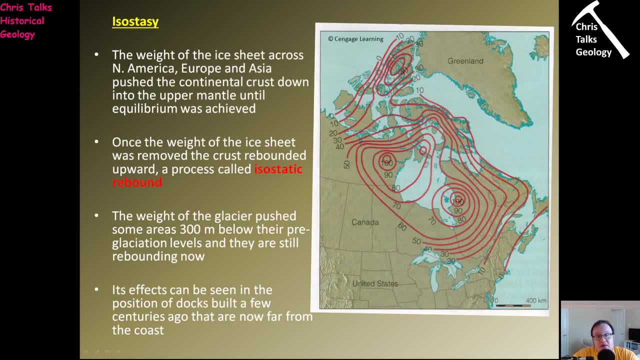 removed. well, the crust is going to removed. well, the crust is going to naturally just bounce straight back up. naturally, just bounce straight back up. naturally, just bounce straight back up, isn't it? isn't it, isn't it? well, yes, but that bounce doesn't happen. well, yes, but that bounce doesn't happen. 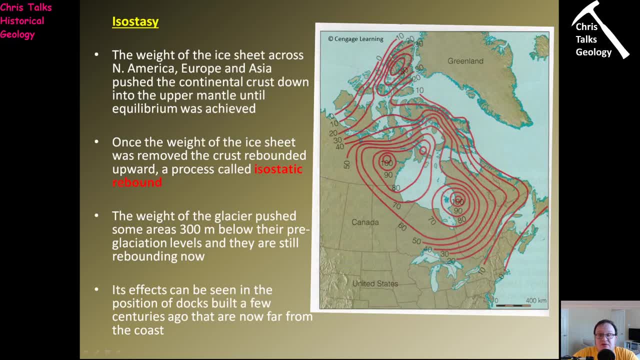 well, yes, but that bounce doesn't happen quickly. the bounce has been happening quickly. the bounce has been happening quickly. the bounce has been happening over, you know a very, very long period of over. you know a very, very long period of over. you know a very, very long period of time. 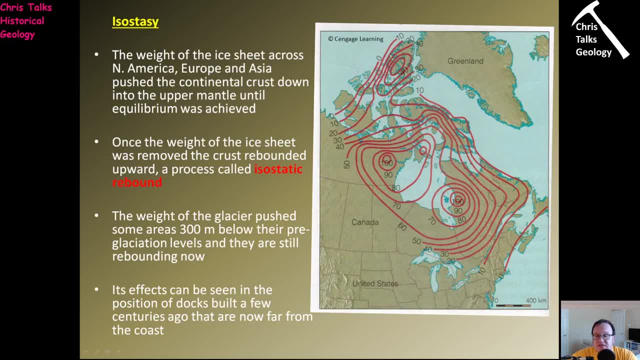 time, time, tens of thousands of years. so if we tens of thousands of years, so if we tens of thousands of years, so if we look at this map here, this is a map. look at this map here. this is a map. look at this map here. this is a map that shows us the isostatic rebound of 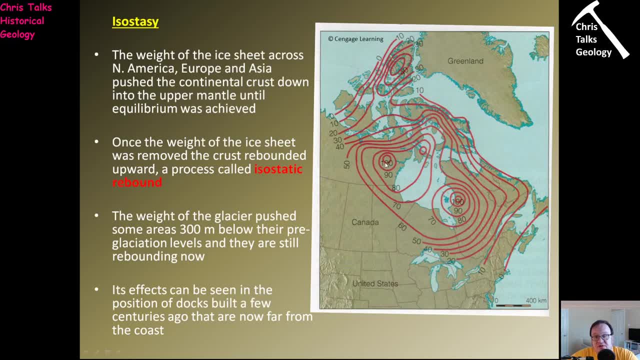 that shows us the isostatic rebound of, that shows us the isostatic rebound of northern canada, so essentially 100. northern canada, so essentially 100. northern canada, so essentially 100, essentially the area with the greatest, essentially the area with the greatest, essentially the area with the greatest rebound, and down around 10 and 0. that's. 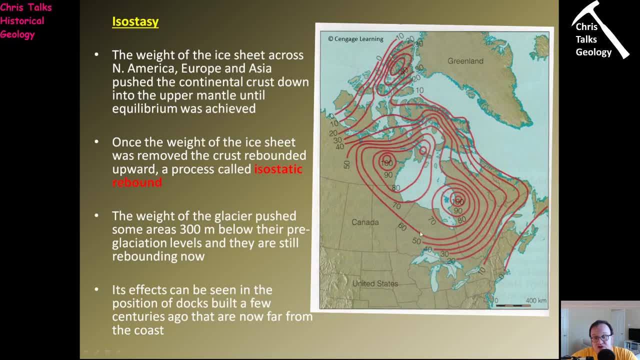 rebound, and down around 10 and 0, that's rebound, and down around 10 and 0, that's the area with the least rebound. and so the area with the least rebound, and so the area with the least rebound. and so these areas, number one is showing us. 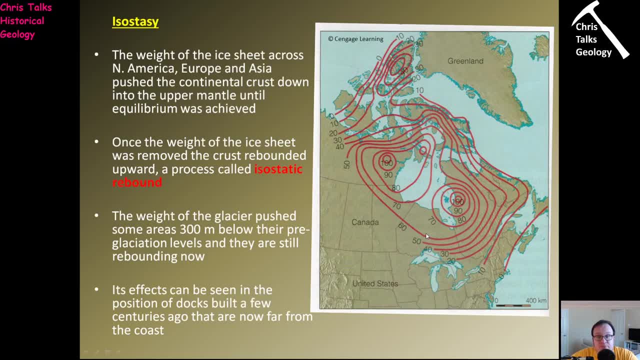 these areas. number one is showing us these areas. number one is showing us well, you know these areas were. well, you know these areas were. well, you know, these areas were definitely covered in very thick ice, definitely covered in very thick ice, definitely covered in very thick ice, weren't they? weren't, they weren't they. you know, so that's what's causing the. you know, so that's what's causing the. you know. so that's what's causing the isostatic rebound. it's just simply the isostatic rebound. it's just simply the. 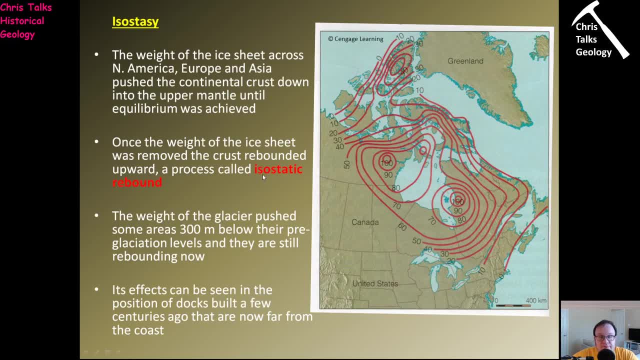 isostatic rebound. it's just simply the removal of the weight, and the cross is removal of the weight and the cross is removal of the weight. and the cross is just popping back up, just popping back up, just popping back up. okay, so the weight of the glaciers push. 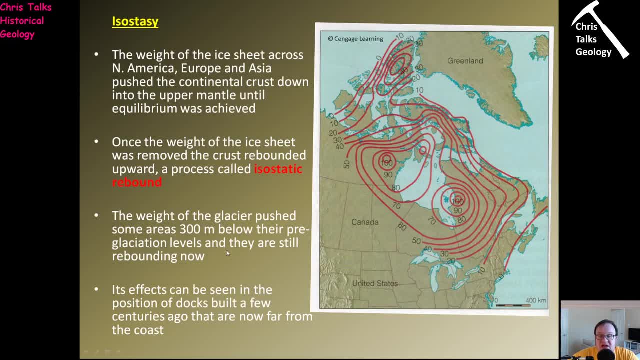 okay, so the weight of the glaciers push. okay, so the weight of the glaciers push some areas about 300 meters below their, some areas about 300 meters below their, some areas about 300 meters below their pre-glaciation level. so that's a pretty pre-glaciation level. so that's a pretty. 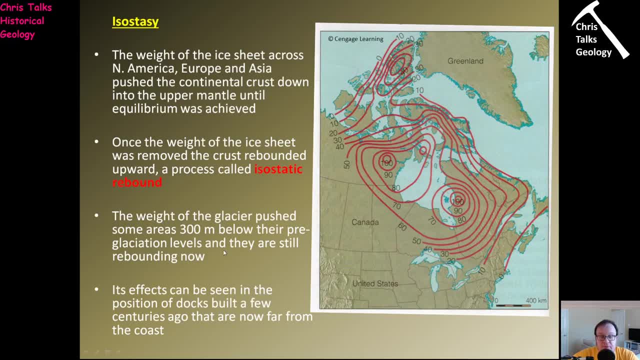 pre-glaciation level. so that's a pretty substantial, you know substantial, you know substantial, you know drop, drop, drop. so and essentially its effects can still so, and essentially its effects can still so and essentially its effects can still be seen now. so when we jump to the next, be seen now. so when we jump to the next, be seen now. so when we jump to the next page, what you're going to see is you're page. what you're going to see is you're page. what you're going to see is you're going to see a beach and it's going to 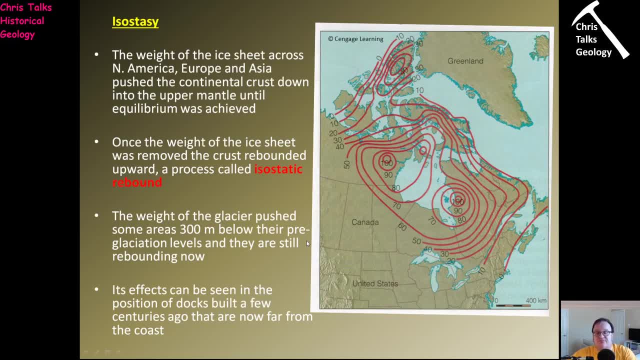 going to see a beach and it's going to going to see a beach and it's going to show you the indications of the steady, show you the indications of the steady, show you the indications of the steady rise of the beach. so here we go. so here's a beach in. 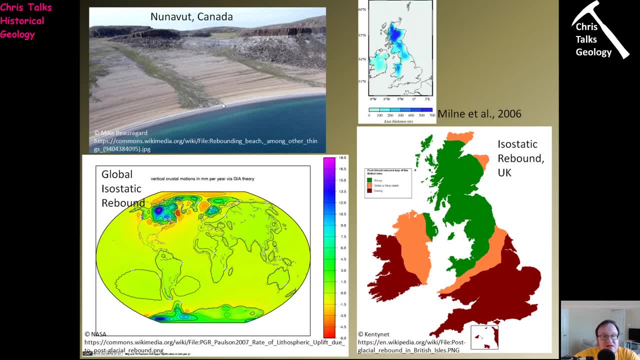 so here we go. so here's a beach in. so here we go. so here's a beach in. none of it in canada, none of it in canada, none of it in canada. and you can see these lines give you an, and you can see these lines give you an. 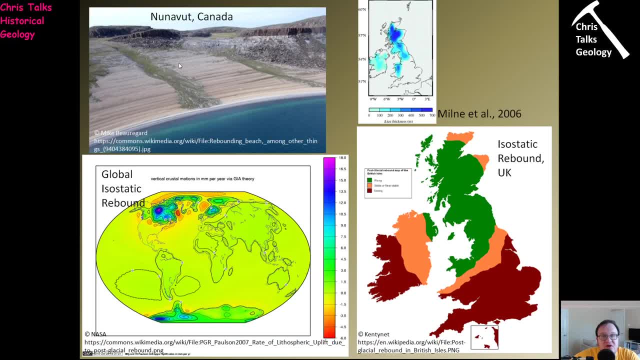 and you can see these lines give you an indication of the of the beach, slowly. indication of the of the beach slowly. indication of the of the beach slowly but surely rising relative to the sea, but surely rising relative to the sea, but surely rising relative to the sea. so this beach, you know this would have. 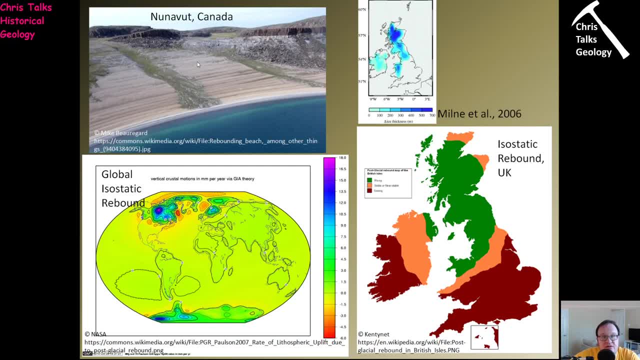 so this beach, you know this would have. so this beach, you know this would have been the beach i don't know been the beach, i don't know been the beach, i don't know. a few, you know, maybe a thousand years ago, a few, you know, maybe a thousand years ago. 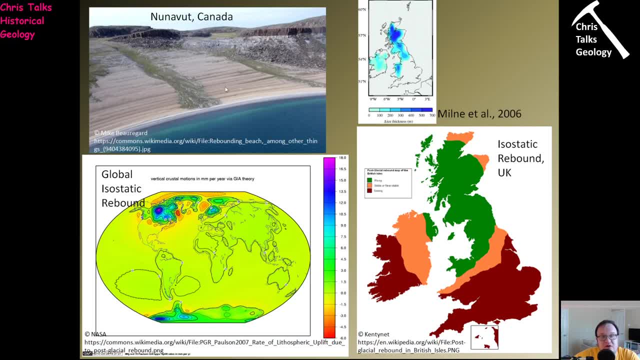 a few. you know, maybe a thousand years ago, and over the thousands of years, the, and over the thousands of years, the, and over the thousands of years, the beach has steadily been getting, beach has steadily been getting. beach has steadily been getting lower and lower and lower as the area 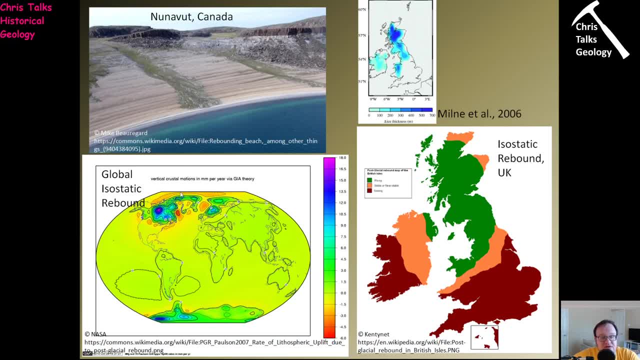 lower and lower and lower as the area, lower and lower and lower as the area of land here rises up of land here rises up, of land here rises up. we get quite a lot in northern europe. so we get quite a lot in northern europe, so we get quite a lot in northern europe. so scandinavia, we also get a little bit in. 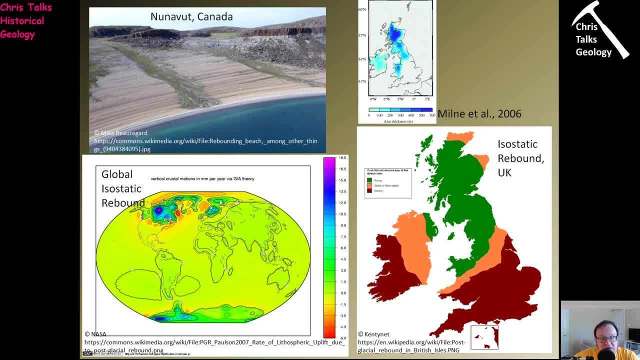 scandinavia. we also get a little bit in scandinavia, we also get a little bit in the united kingdom. the united kingdom, the united kingdom, and we get quite. you know, get quite a and we get quite. you know, get quite a and we get quite. you know, get quite a bit over here in some of the 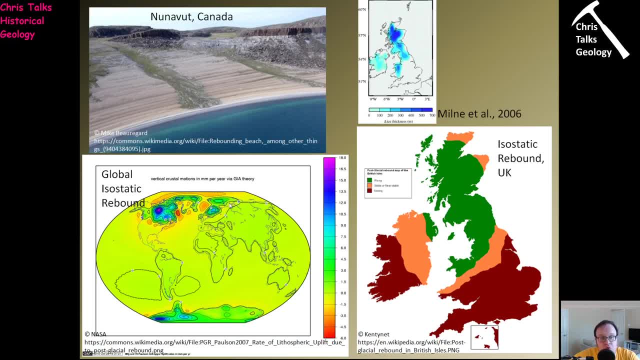 bit over here, in some of the bit over here, in some of the you know random little islands that we you know random little islands that we you know random little islands that we get uh, you know, get uh, you know, get uh. you know north of russia, north of you know. 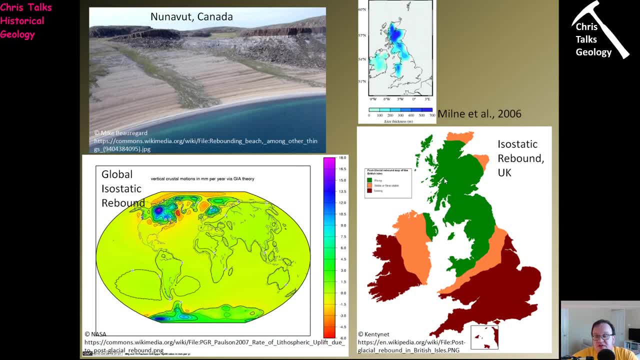 north of russia, north of you know, north of russia, north of you know, north of norway, north of norway. in terms of the united kingdom, the in terms of the united kingdom, the in terms of the united kingdom, the united kingdom is actually quite an. 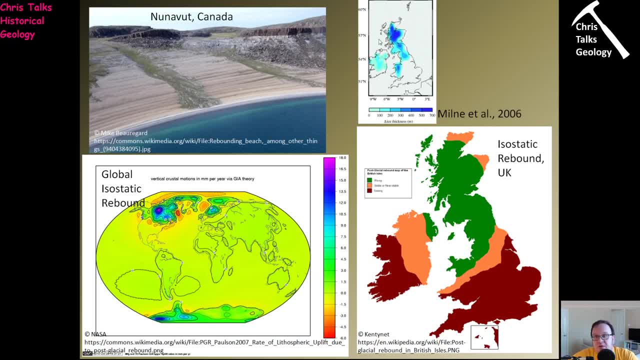 united kingdom is actually quite an united kingdom is actually quite an interesting case, interesting case. interesting case because, in terms of where we have the because, in terms of where we have the because, in terms of where we have the ice thickness, you can see we have a lot. 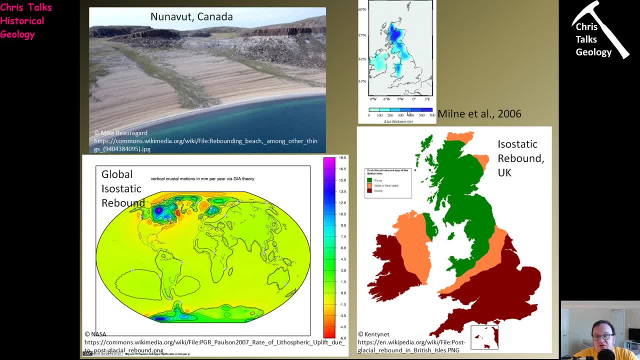 ice thickness. you can see we have a lot ice thickness. you can see we have a lot of ice thickness in scotland. here when of ice thickness in scotland. here. when of ice thickness in scotland. here, when you look at the color of it, the ice. 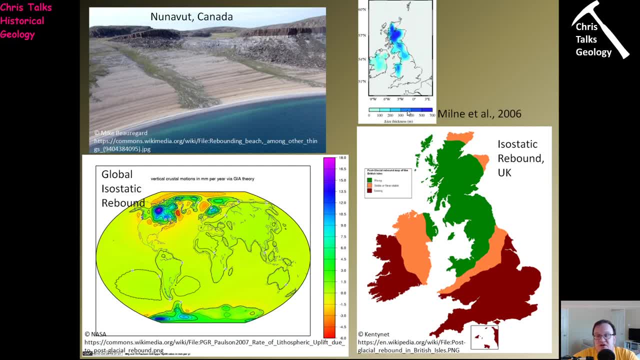 you look at the color of it- the ice. you look at the color of it, the ice would have been somewhere in the 300 to would have been somewhere in the 300 to would have been somewhere in the 300 to 400 meter range. so you know thick. 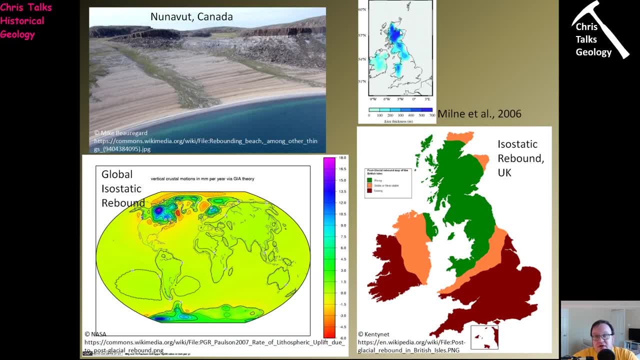 400 meter range. so you know thick, 400 meter range. so you know thick, quite heavy ice and it's pushed down the quite heavy ice and it's pushed down the quite heavy ice and it's pushed down the crust, crust, crust, and so scotland and a bit of northern. 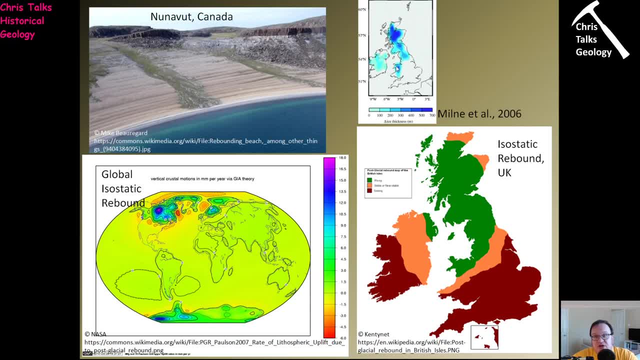 and so scotland and a bit of northern and so scotland and a bit of northern england and some of wales were areas england and some of wales were areas. england and some of wales were areas which were suffering depression, which were suffering depression. 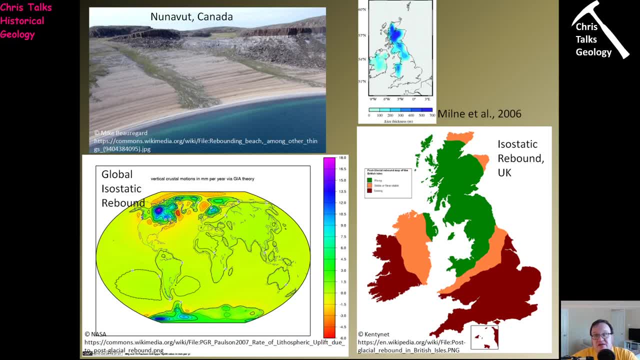 which were suffering depression. they were pushed down by the ice. now they were pushed down by the ice now. they were pushed down by the ice. now, obviously, that ice has now disappeared. obviously that ice has now disappeared. obviously that ice has now disappeared. and so, over the last few thousand years, 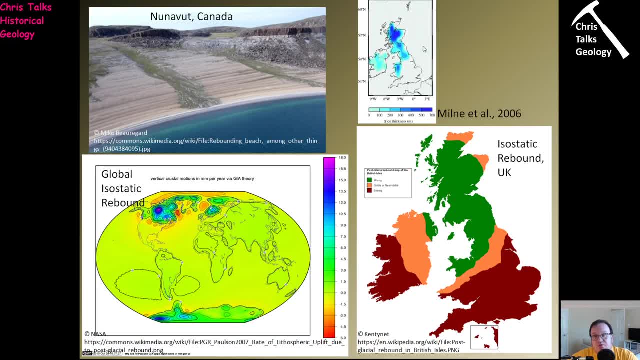 and so over the last few thousand years, and so over the last few thousand years, the united kingdom has literally been, the united kingdom has literally been, the united kingdom has literally been popping up. so the northern parts of popping up, so the northern parts of popping up, so the northern parts of, well, scotland, northern england and wales. 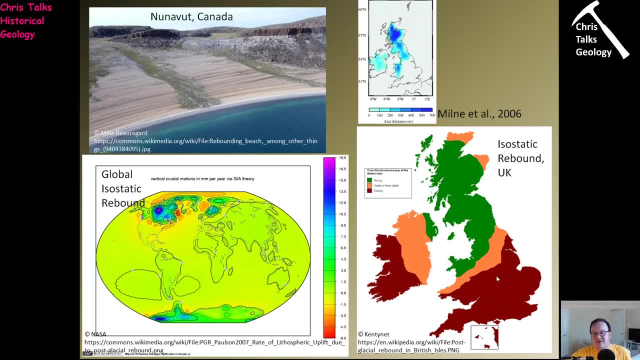 well, scotland, northern england and wales. well, scotland, northern england and wales are literally, are literally, are literally rising. that means the southern part of rising. that means the southern part of rising. that means the southern part of the uk, the uk, the uk is actually sinking the entire united 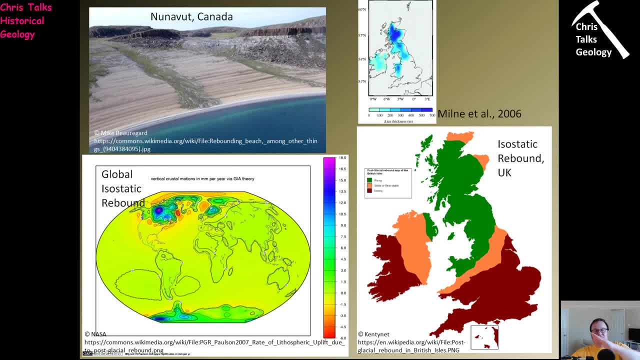 is actually sinking the entire united is actually sinking the entire united kingdom kingdom. kingdom is acting like a giant seesaw as scotland is acting like a giant seesaw as scotland is acting like a giant seesaw as scotland rises, rises, rises. the southern part of the united kingdom. 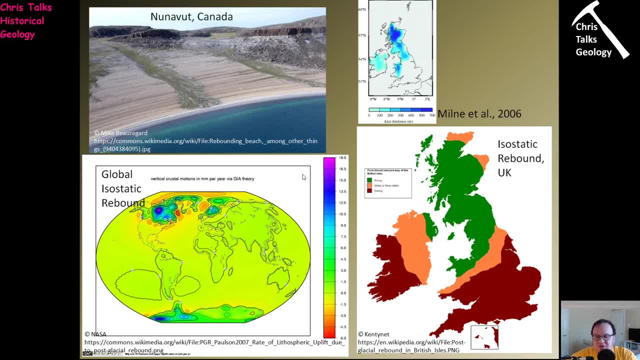 the southern part of the united kingdom. the southern part of the united kingdom goes down, which i think is quite fun. goes down, which i think is quite fun. goes down, which i think is quite fun. that's quite a good part of geology, it's. that's quite a good part of geology, it's. 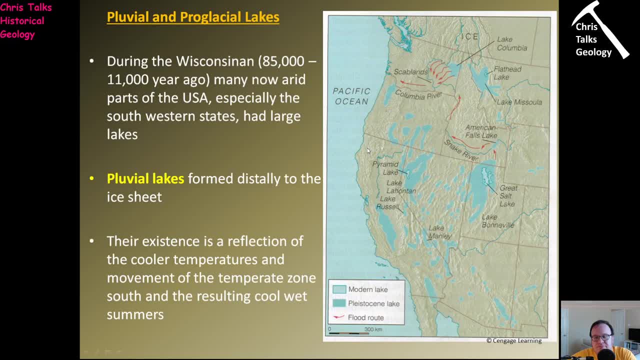 that's quite a good part of geology. it's quite interesting. so the final few things we have to think, so the final few things we have to think, so the final few things we have to think about- are what's happened to the water, about are what's happened to the water. 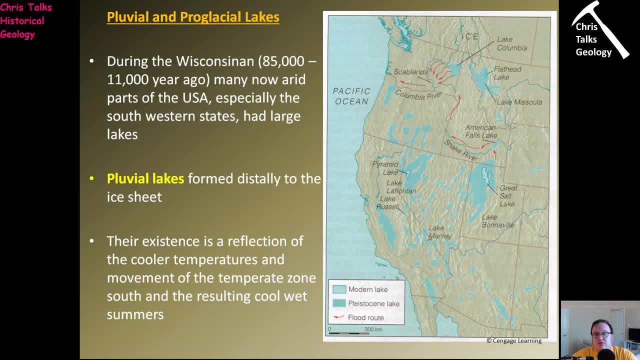 about are what's happened to the water that was produced by these glaciers, that was produced by these glaciers, that was produced by these glaciers? well, the water from the glaciers are well, the water from the glaciers are well, the water from the glaciers are going to form lakes. that's not really a 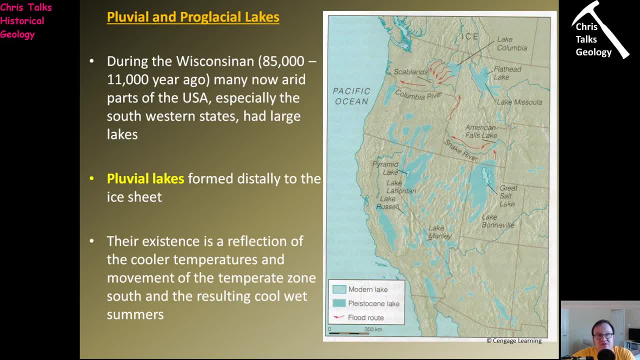 going to form lakes. that's not really a going to form lakes. that's not really a huge shock, huge shock, huge shock. so these lakes are referred to as. so these lakes are referred to as. so these lakes are referred to as pluvial lakes or proglacial lakes. 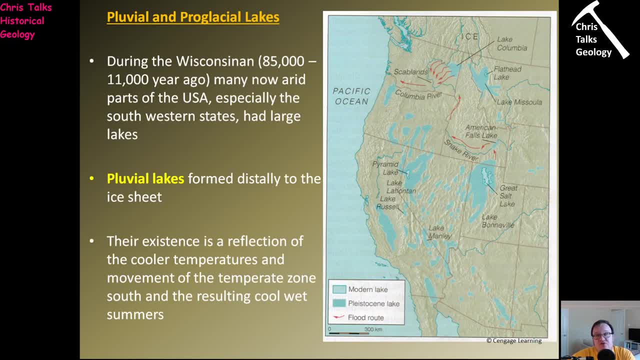 pluvial lakes or proglacial lakes. pluvial lakes or proglacial lakes, depending on where they're located, depending on where they're located, depending on where they're located. so during the wisconsin's, that's 85 to. so during the wisconsin's, that's 85 to. 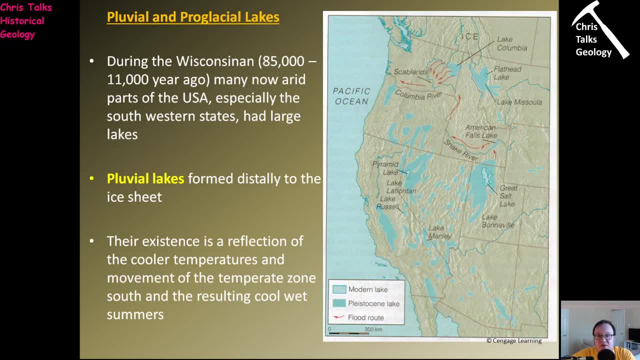 so during the wisconsin's, that's 85 to 11 000 years ago, 11 000 years ago, 11 000 years ago, many now arid parts of the us, especially many now arid parts of the us, especially many now arid parts of the us, especially in the southwest united states, had large 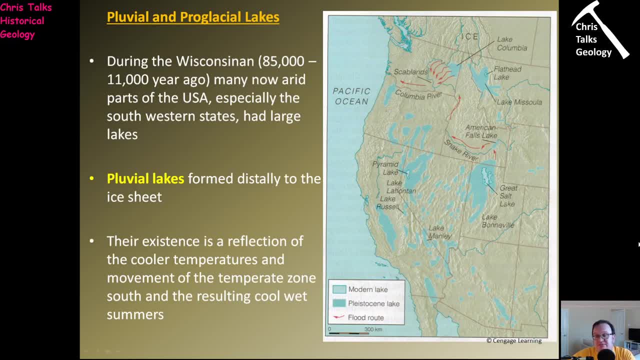 in the southwest united states had large in the southwest united states had large lakes, lakes, lakes. so we've discussed how this area. so we've discussed how this area, so we've discussed how this area essentially became temperate and the essentially became temperate and the essentially became temperate. and the ice water, well, the water coming off, the ice water. well, the water coming off the ice water, well, the water coming off the glaciers produce very, very large lakes. glaciers produce very, very large lakes. glaciers produce very, very large lakes in this area. so it would have been an in this area. so it would have been an. 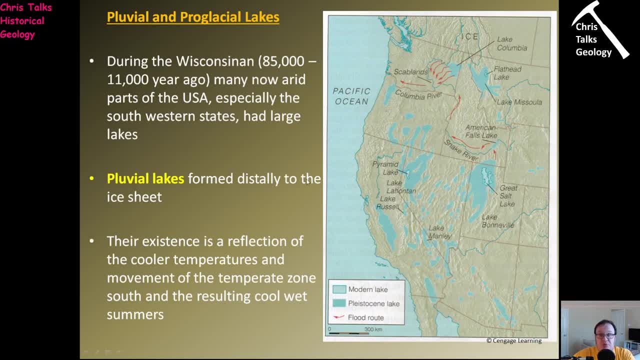 in this area. so it would have been an area of you know forests and grassland, area of you know forests and grassland, area of you know forests and grassland and large lakes would be quite a, and large lakes would be quite a, and large lakes would be quite a pleasant place, quite a pleasant place to 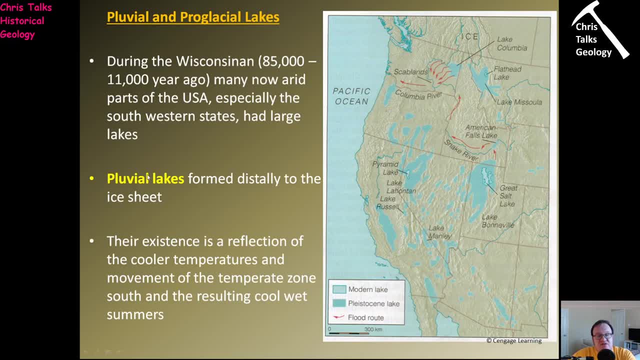 pleasant place, quite a pleasant place to pleasant place, quite a pleasant place to be, actually be, actually be actually now. the lakes that form away from the now, the lakes that form away from the now, the lakes that form away from the glacier, are referred to as pluvial lakes. 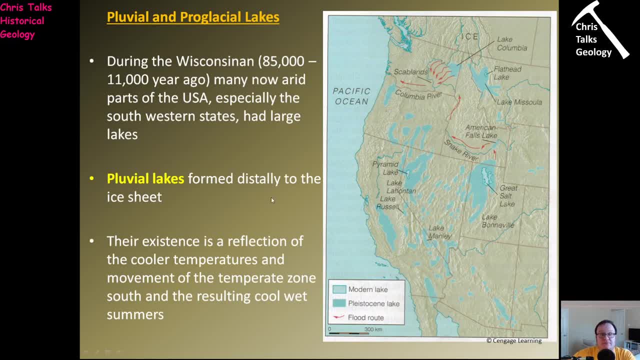 glacier are referred to as pluvial lakes. glacier are referred to as pluvial lakes. okay, so they're distal to the glacier. okay, so they're distal to the glacier. okay, so they're distal to the glacier. they formed away from it. they formed away from it. 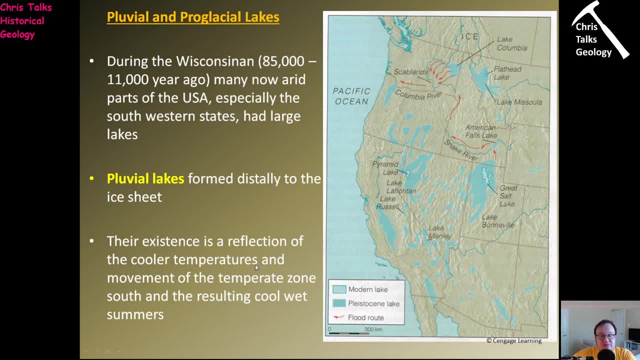 they formed away from it. so their existence is a reflection of, so their existence is a reflection of, so their existence is a reflection of the cooler temperatures, the cooler temperatures, the cooler temperatures, and the movement of the temperate zone and the movement of the temperate zone. 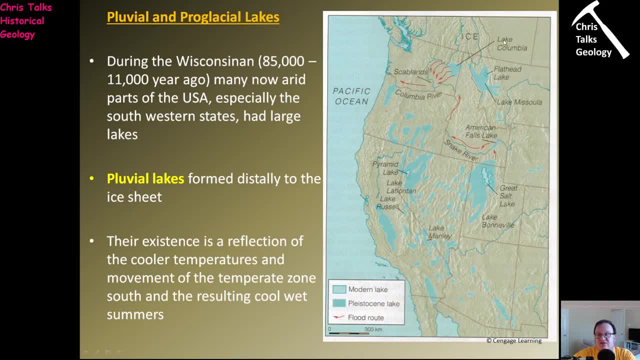 and the movement of the temperate zone south and the resulting cool wet summers south and the resulting cool wet summers south and the resulting cool wet summers. so you have essentially ice melt. so you have essentially ice melt. so you have essentially ice melt giving water to the area, but also you. 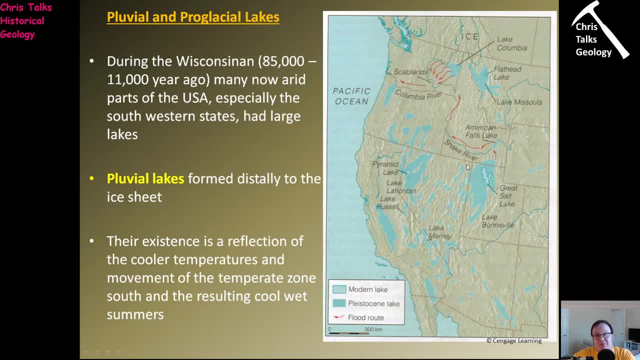 giving water to the area, but also you giving water to the area, but also you. so just to give you some idea, by the way, so just to give you some idea, by the way, so just to give you some idea, by the way. so you know, this is great salt lake here. so you know this is great salt lake here. so you know this is great salt lake here and you can see, you know this would have and you can see, you know this would have and you can see, you know this would have been the size of the lake. 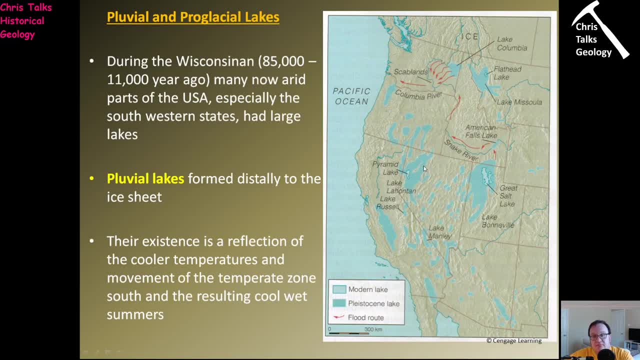 been the size of the lake, been the size of the lake during the pleistocene. so we had some during the pleistocene, so we had some during the pleistocene, so we had some huge, huge lakes here. so a classic example of a puvil that. 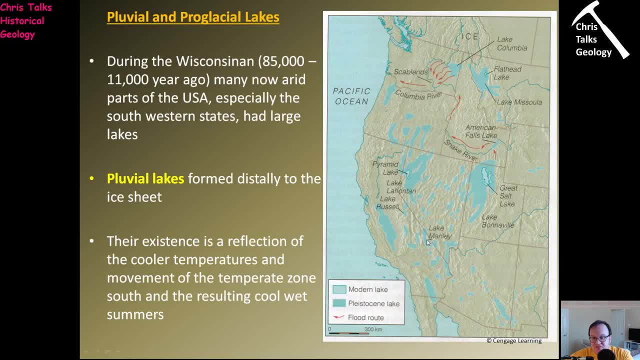 so a classic example of a puvil. that so a classic example of a puvil. that pluvial lake is lake manly. so lake pluvial lake is lake manly. so lake pluvial lake is lake manly. so lake manly is right here. just on the 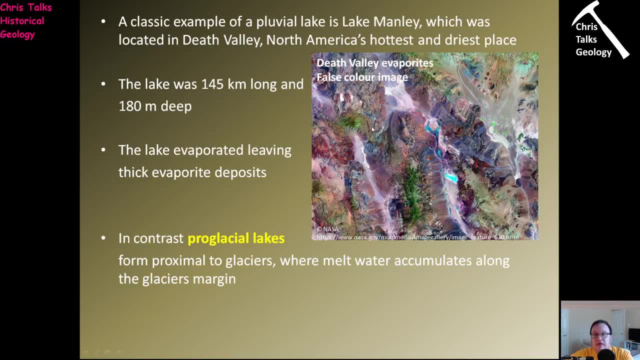 manly is right here, just on. the manly is right here, just on the california border, california border, california border, and it's now located in death valley. so, and it's now located in death valley. so, and it's now located in death valley. so bit of a changing climate, eh. 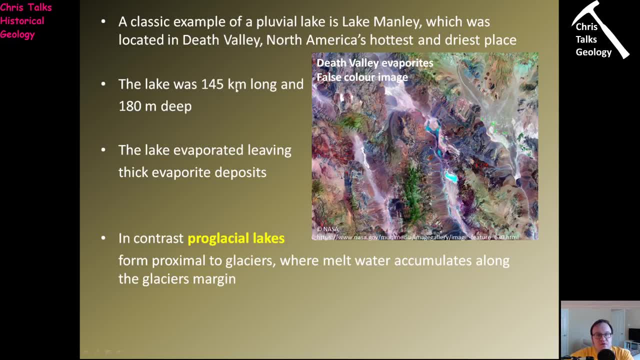 bit of a changing climate, eh, bit of a changing climate, eh so. so so we can see the lake itself was around. we can see the lake itself was around. we can see the lake itself was around 145 kilometers long and about 180 meters: 145 kilometers long and about 180 meters. 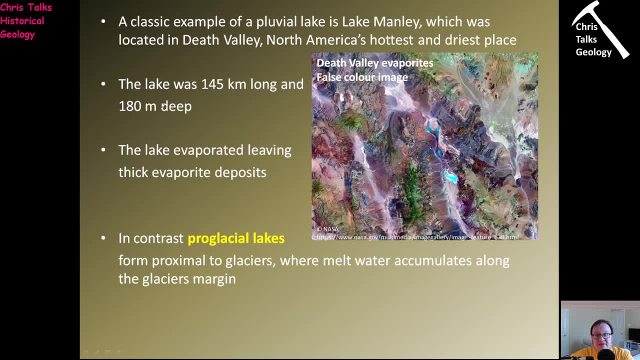 145 kilometers long and about 180 meters deep, so it's a pretty substantial body deep, so it's a pretty substantial body deep, so it's a pretty substantial body of water, of water, of water, and the lake has evaporated away and the lake has evaporated away. 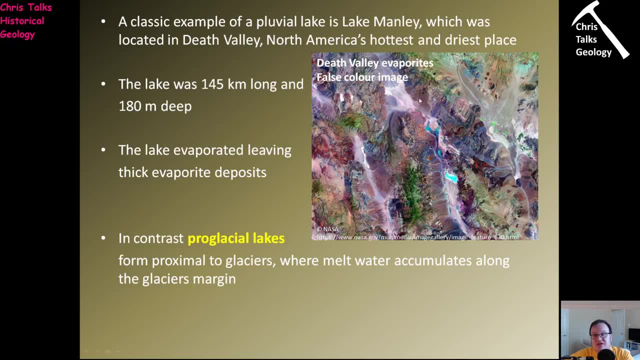 and the lake has evaporated away, leaving evaporating deposits. now this is leaving evaporating deposits now. this is leaving evaporating deposits now. this is a false color image. a false color image, a false color image. but you can see here these kind of these, but you can see here these kind of these. 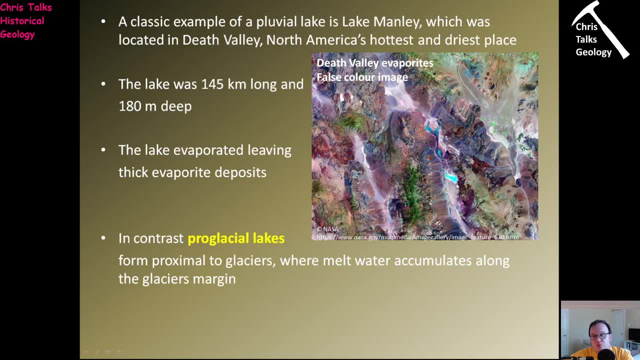 but you can see here these kind of these areas which are whiter areas, which are whiter areas, which are whiter, and these blue, the blue areas represent, and these blue, the blue areas represent, and these blue, the blue areas represent water, water, water, left, water that's left and the white 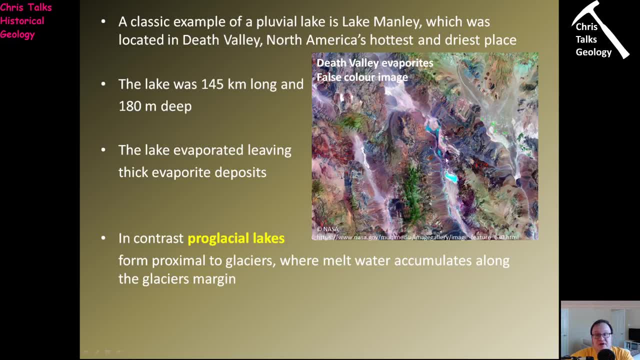 left water that's left, and the white left water that's left. and the white areas here represent the evaporites. areas here represent the evaporites. areas here represent the evaporites formed: formed: formed by the evaporation of this water and if. by the evaporation of this water and if. by the evaporation of this water. and if you were to go all the way along you, you were to go all the way along you, you were to go all the way along you. know the valley, you would see just a. know the valley, you would see just a. 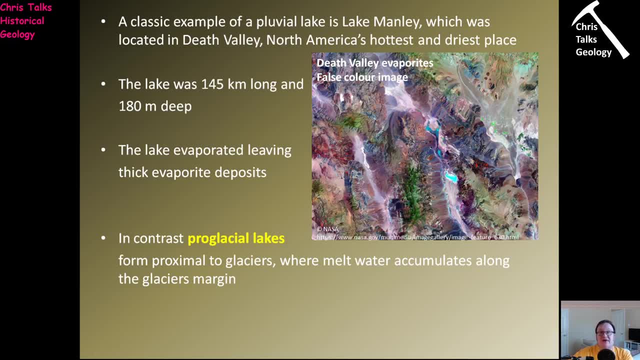 know the valley, you would see just a constant sheet of evaporites. constant sheet of evaporites. constant sheet of evaporites produced as lake manly went and produced as lake manly went and produced as lake manly went and evaporated away, evaporated away, evaporated away. now, in contrast, proglacial lakes are: 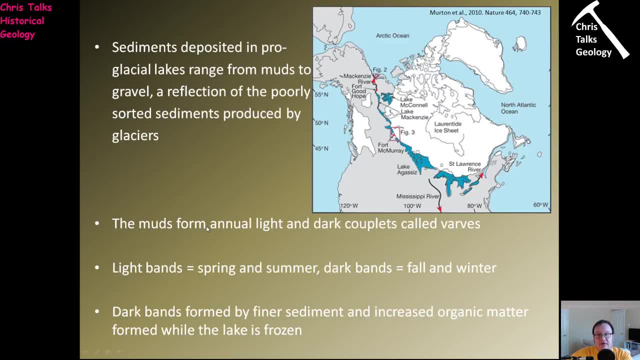 now, in contrast, proglacial lakes are now. in contrast, proglacial lakes are going to form, going to form, going to form right next to the glacier. okay, so here, right next to the glacier. okay, so here, right next to the glacier. okay, so here we go. 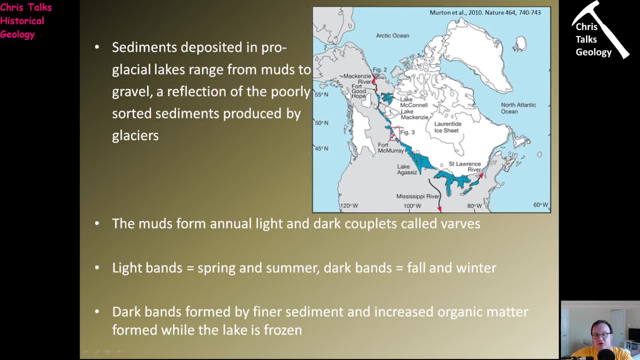 we go, we go. so these are the proglacial lakes now. so these are the proglacial lakes now. so these are the proglacial lakes now. typically. there will be something about typically. there will be something about typically. there will be something about the terrain that will stop the water. 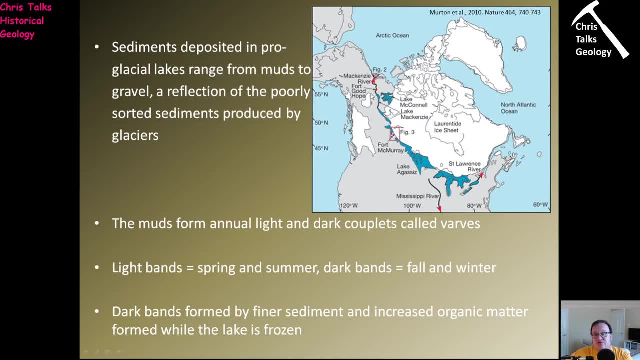 the terrain that will stop the water, the terrain that will stop the water escaping, escaping, escaping. okay, it could also be retained by a. okay, it could also be retained by a. okay, it could also be retained by a moraine, moraine, moraine, if a moraine is, you know, is tight, is. 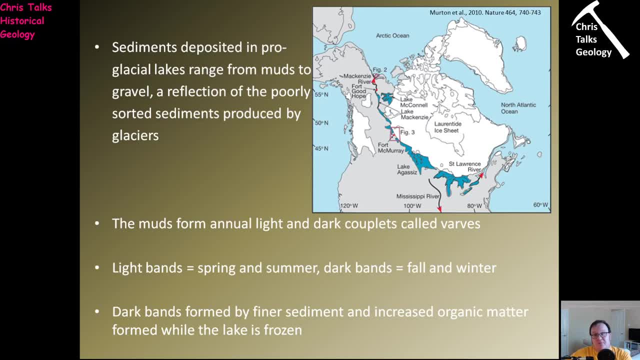 if a moraine is, you know, is tight is. if a moraine is, you know, is tight, is good enough it can retain the water. good enough, it can retain the water. good enough it can retain the water behind it, so forming a lake behind it, so forming a lake. 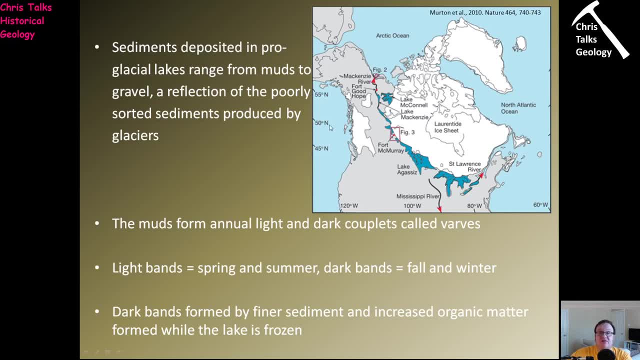 behind it, so forming a lake. so proglacial lakes will have sediments. so proglacial lakes will have sediments. so proglacial lakes will have sediments deposited in them directly from the deposited in them, directly from the deposited in them directly from the glacier. 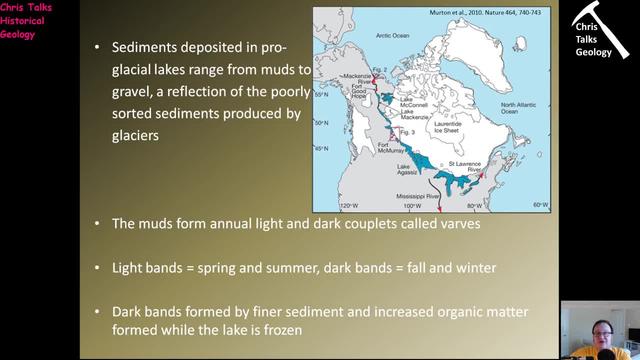 glacier, glacier. so that means you will have a mixture of. so that means you will have a mixture of. so that means you will have a mixture of muds to gravel. so you know quite a big muds to gravel. so you know quite a big muds to gravel. so you know quite a big range of sediments. so quite a poorly. 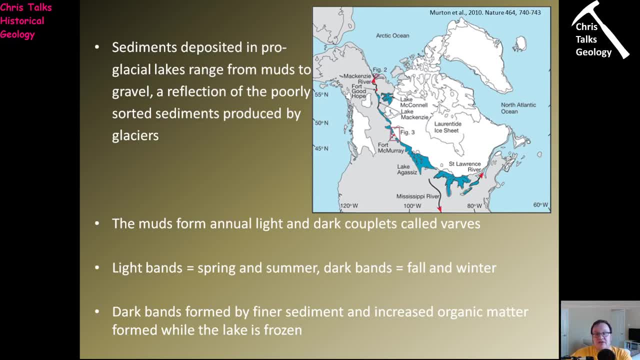 range of sediments. so quite a poorly range of sediments, so quite a poorly sorted range, sorted range, sorted range. now the muds form, what we refer to as now the muds form, what we refer to as now the muds form, what we refer to as bands which are light and dark and 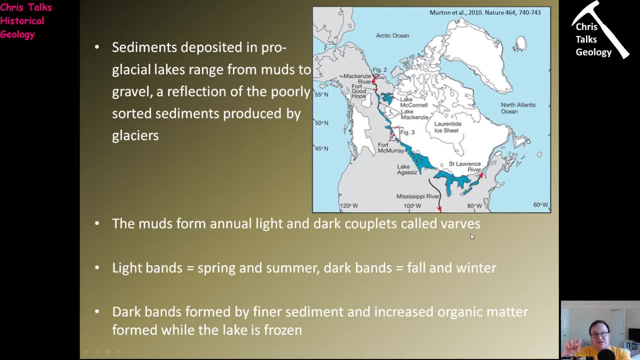 bands which are light and dark and bands which are light and dark, and they're called varves. they're called varves, they're called varves. so the light bands represent spring, and so the light bands represent spring, and so the light bands represent spring and summer, and the dark bands represent fall. 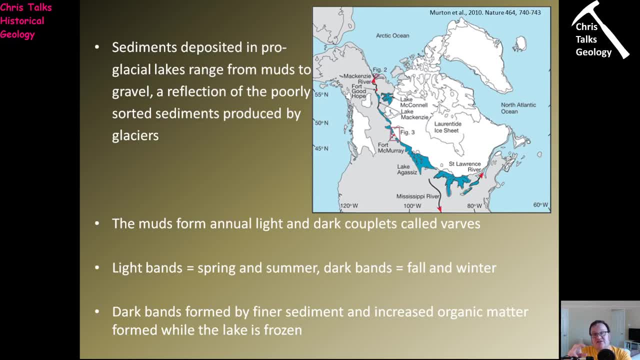 summer and the dark bands represent fall, summer and the dark bands represent fall and winter. so if you look at these lake and winter, so if you look at these lake and winter, so if you look at these lake sediments from the proglacial lakes, you, sediments from the proglacial lakes, you, 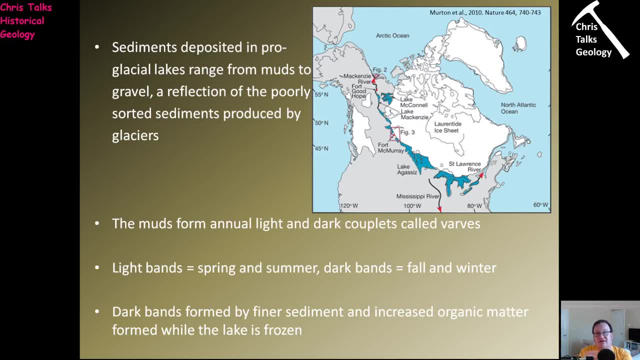 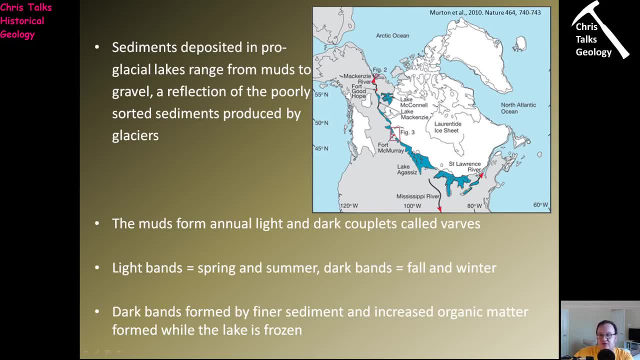 and that's formed by the very, very fine, and that's formed by the very, very fine muddy material. so, as you say, these are the proglacial. so as you say, these are the proglacial, so as you say these are the proglacial lakes here and they essentially form: 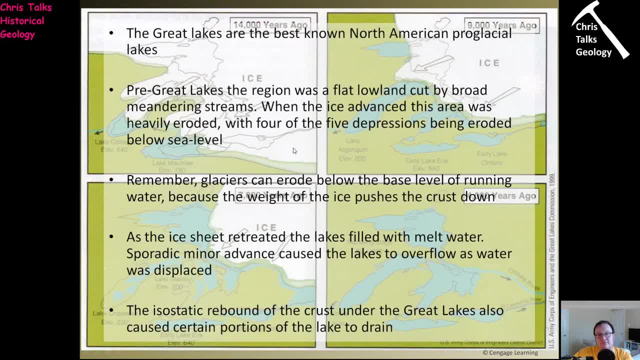 lakes here and they essentially form lakes here and they essentially form along the glacial margin. so, in terms of proglacial lakes, the best. so in terms of proglacial lakes, the best. so in terms of proglacial lakes, the best example, example, example are the great lakes, so the 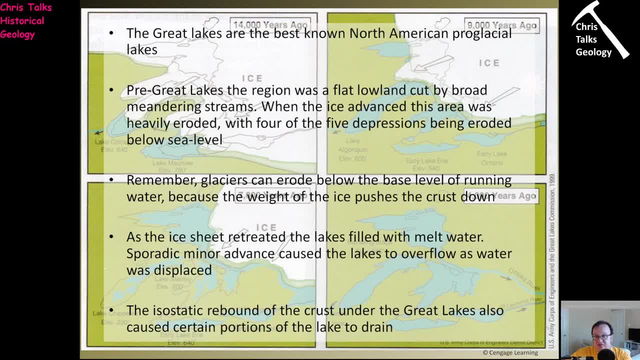 are the great lakes. so the are the great lakes. so the great lakes, uh great lakes, uh great lakes, uh, pre-great lakes, the region was an area. pre-great lakes, the region was an area pre-great lakes. the region was an area of low land cut by broad meander river. 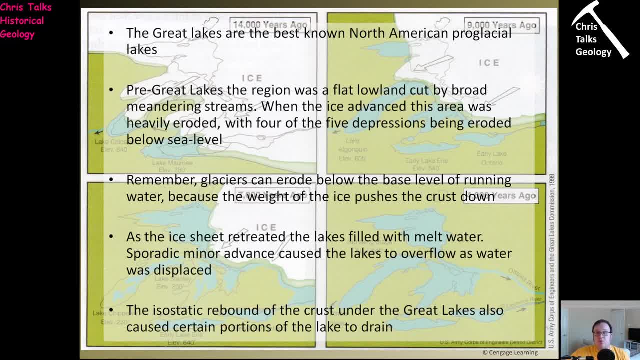 of low land cut by broad meander river, of low land cut by broad meander river. so it was so, it was, so it was very flat terrain anyway. so when the very flat terrain anyway, so when the very flat terrain anyway. so when the glaciers came over, once again, they 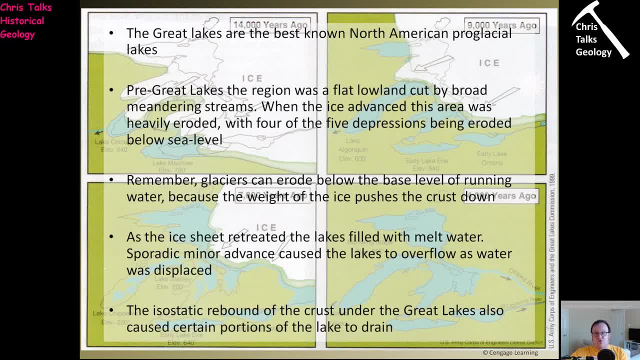 glaciers came over once again. they glaciers came over once again. they eroded the area. so any vegetation gone eroded the area. so any vegetation gone eroded the area. so any vegetation gone. any soil gone, so the glacier is moving. any soil gone, so the glacier is moving. 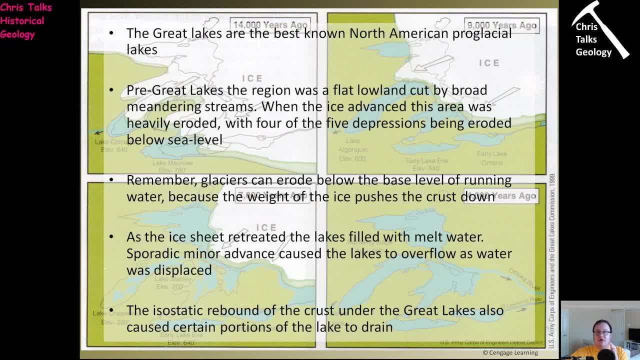 any soil gone. so the glacier is moving straight over the bedrock, straight over the bedrock, straight over the bedrock. but what does it do to the bedrock? well, but what does it do to the bedrock? well, but what does it do to the bedrock? well, it doesn't just move across it. 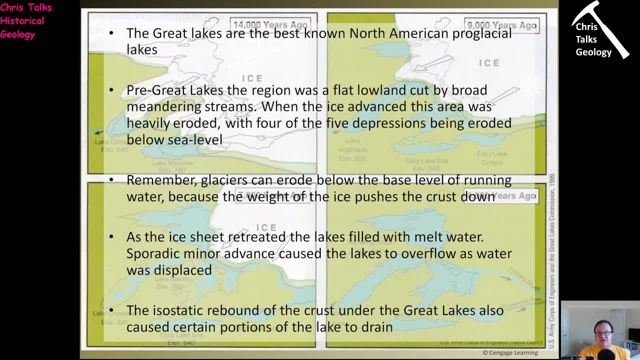 it doesn't just move across it. it doesn't just move across it, it grinds at it. it forms a depression. it grinds at it, it forms a depression. it grinds at it, it forms a depression. doesn't it, doesn't? it, doesn't it? it slowly grinds away at the, the bedrock. 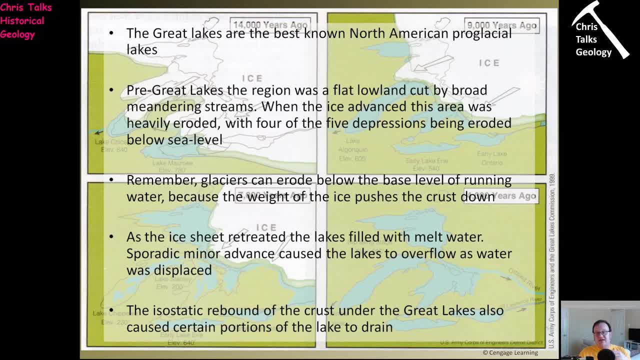 slowly grinds away at the. the bedrock slowly grinds away at the the bedrock. it's now lower, it's now lower, it's now lower. the other interesting thing is is that the other interesting thing is is that the other interesting thing is is that the glacier can actually cut below the. 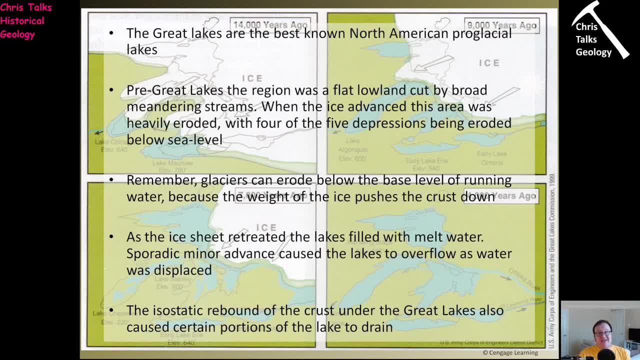 the glacier can actually cut below the. the glacier can actually cut below the base level, base level, base level. so if you remember the base level is so if you remember the base level is so if you remember the base level is the lowest possible level a river can. 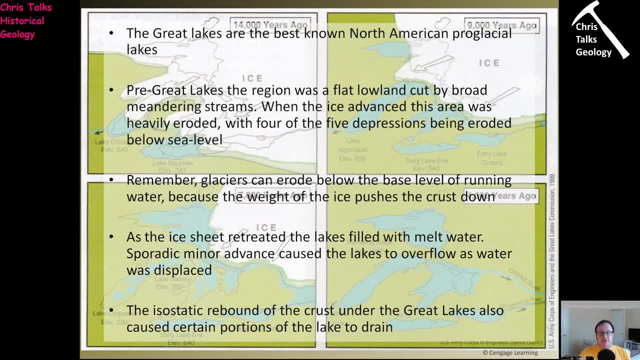 the lowest possible level. a river can. the lowest possible level. a river can cut to cut to cut to okay. so a river can only cut down to the okay. so a river can only cut down to the okay. so a river can only cut down to the base level, and the base level is: 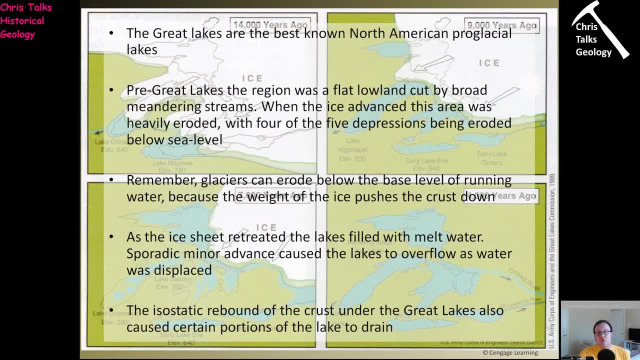 base level and the base level is base level and the base level is normally sea level, normally sea level, normally sea level. okay, okay, okay. when a glacier moves across the area on. when a glacier moves across the area on. when a glacier moves across the area, on the other hand, it can actually cut. 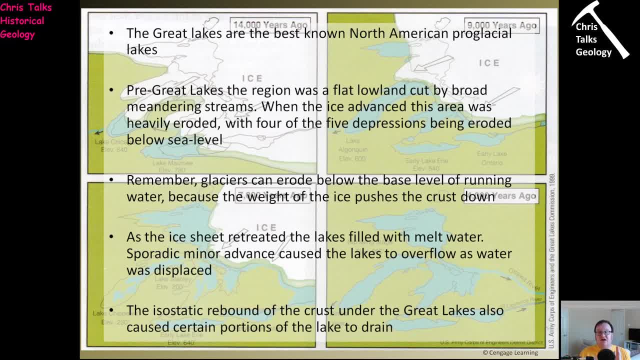 the other hand, it can actually cut, the other hand, it can actually cut below that base level, so it can. it can below that base level, so it can. it can below that base level, so it can. it can effectively cut below sea level, effectively cut below sea level. 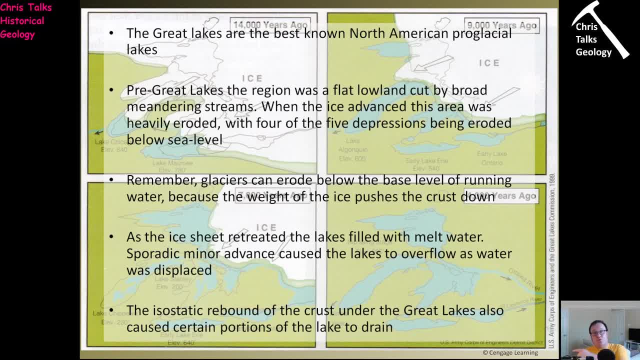 effectively cut below sea level. so that means that any river in the so. that means that any river in the so. that means that any river in the area, instead of flowing towards the sea area, instead of flowing towards the sea area, instead of flowing towards the sea, will actually flow towards that. 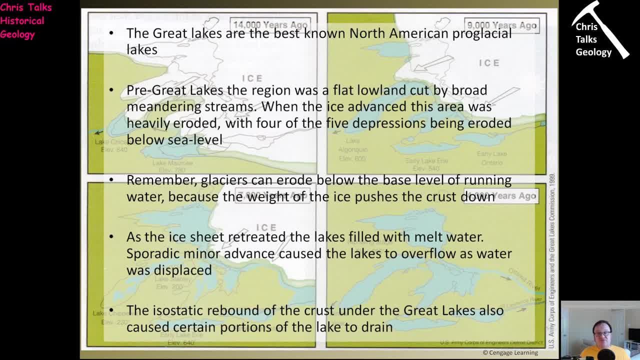 will actually flow towards that, will actually flow towards that: depression instead, depression instead, depression instead. so that's why, all of a sudden, you get so, that's why, all of a sudden, you get so, that's why, all of a sudden, you get rivers flowing into the great lakes. 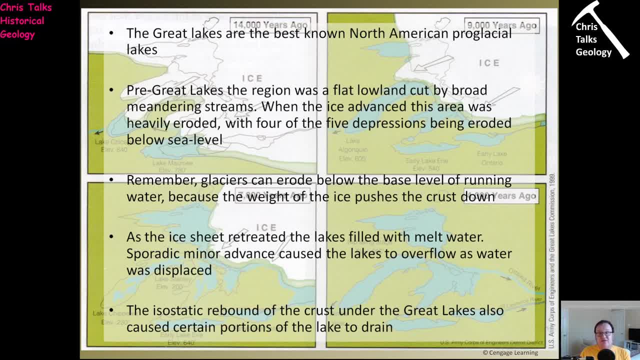 rivers flowing into the great lakes, rivers flowing into the great lakes, producing the great lakes. because producing the great lakes? because producing the great lakes, because they're a natural depression, they're a natural depression, they're a natural depression in that area which is which is lower, in that area which is which is lower. 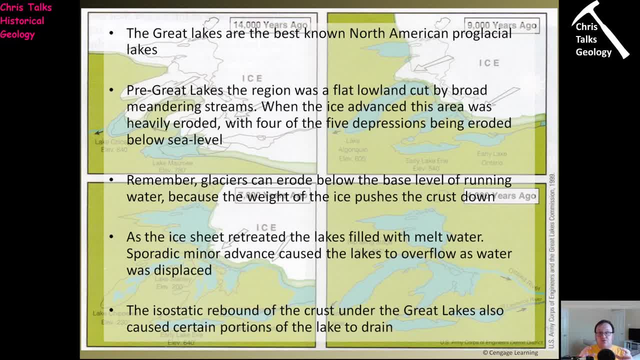 in that area, which is, which is lower than the base level. so you know water than the base level. so you know water than the base level. so you know water naturally wants to move towards them. so if we look here, so as the ice sheet. so if we look here, so as the ice sheet. 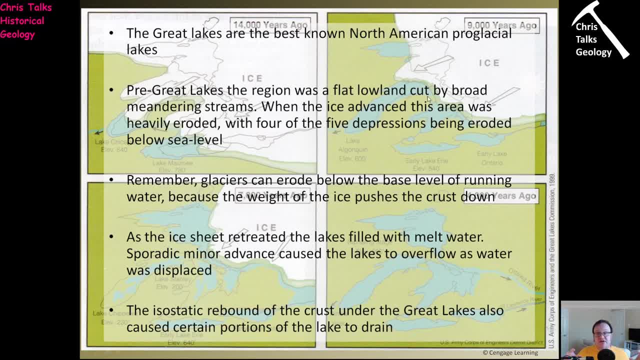 so, if we look here, so as the ice sheet retreats, obviously the ice water helps retreats, obviously the ice water helps retreats, obviously the ice water helps to fill the lakes, along with those to fill the lakes, along with those to fill the lakes, along with those rivers which are now channeling towards. 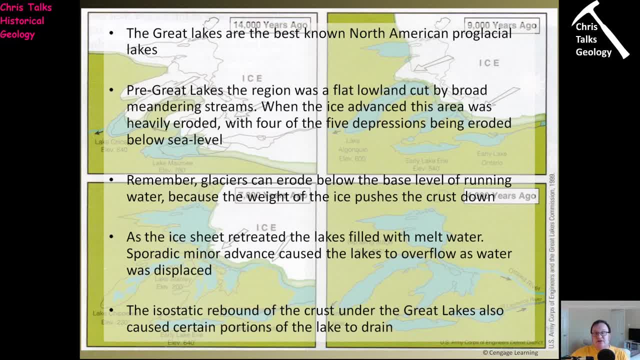 rivers which are now channeling towards rivers which are now channeling towards them, them, them and the lakes have been reworked to some and the lakes have been reworked to some and the lakes have been reworked to some degree by a bit of isostatic rebound. 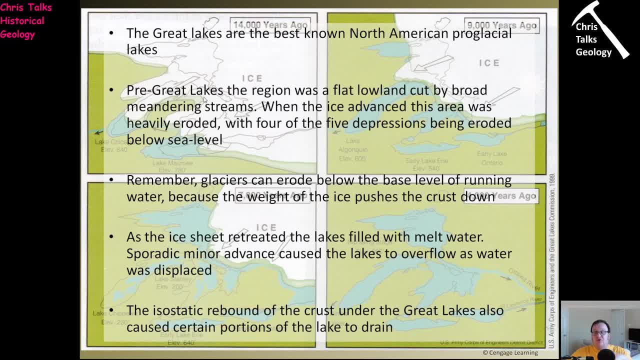 degree by a bit of isostatic rebound. degree by a bit of isostatic rebound because obviously, once the ice has gone, because obviously once the ice has gone, because obviously once the ice has gone, the area is springing up, not not a huge. the area is springing up, not not a huge. 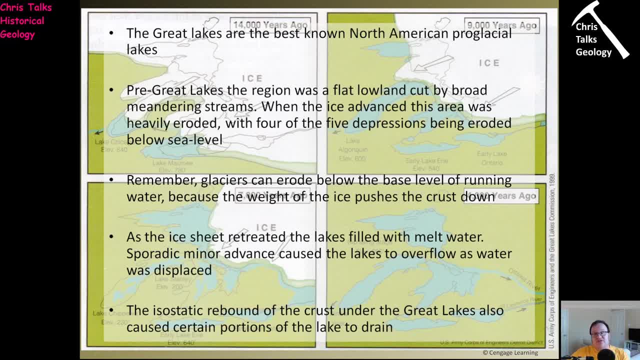 the area is springing up, not not a huge amount, but it is springing up and that amount, but it is springing up and that amount, but it is springing up and that is going to affect how the water is is going to affect how the water is. 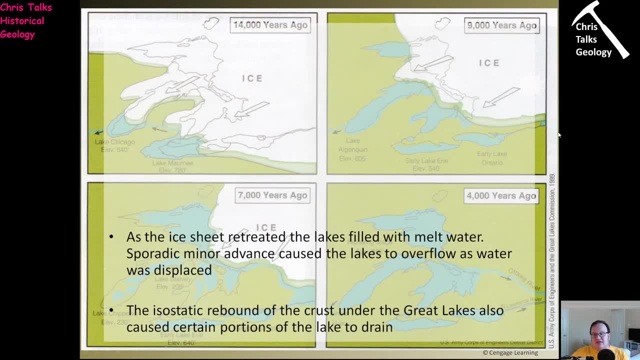 is going to affect how the water is distributed. so if we distributed, so if we distributed, so if we just get rid of this here and have a look, just get rid of this here and have a look, just get rid of this here and have a look at the diagram behind, here we go. 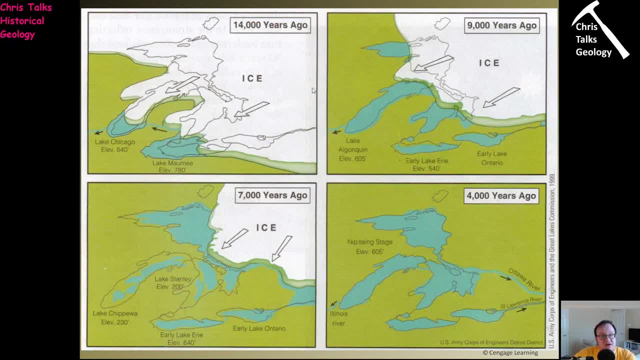 at the diagram behind here we go, at the diagram behind, here we go. so very simplistic diagram, but 14 000. so very simplistic diagram, but 14 000. so very simplistic diagram, but 14 000. you go here the ice. here's the ice sheet. 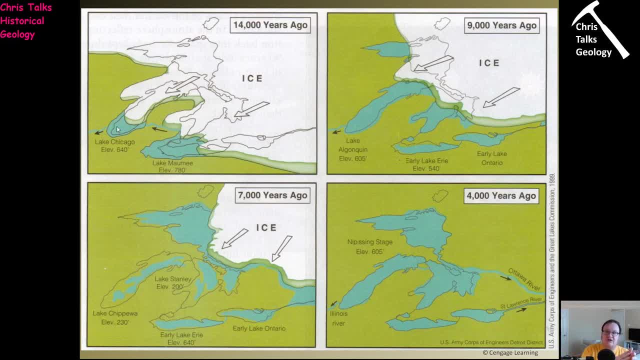 you go here the ice, here's the ice sheet. you go here the ice, here's the ice sheet over the top. now remember this ice over the top. now remember this ice sheet over the top. now remember this ice sheet is gouging into the bedrock, okay. 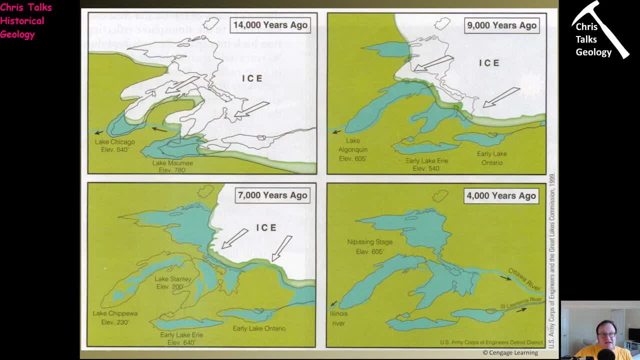 is gouging into the bedrock. okay, is gouging into the bedrock. okay, it's cutting down below base level. so it's cutting down below base level. so it's cutting down below base level. so it means the area of terrain here, that's. it means the area of terrain here, that's. 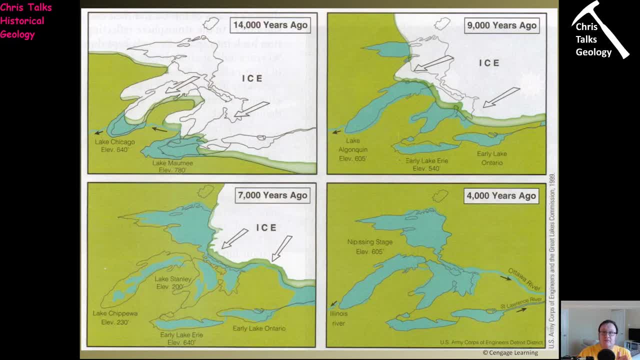 it means the area of terrain here that's covered by ice is going to be below sea. covered by ice is going to be below sea. covered by ice is going to be below sea level- level level. okay, so that means water is going to. okay, so that means water is going to. 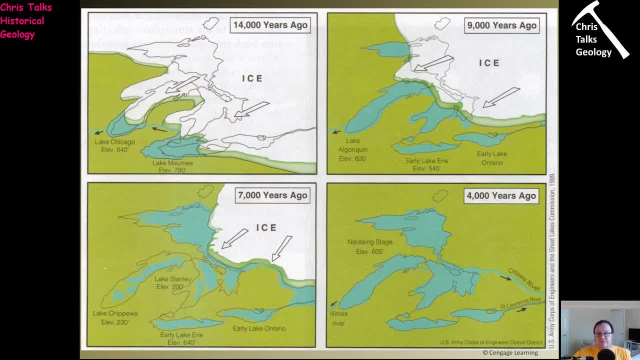 okay, so that means water is going to naturally want to flow, naturally want to flow, naturally want to flow into the, into the lakes, into the, into the lakes, into the, into the lakes. so so, so, around 9 000 years ago, obviously the, around 9 000 years ago, obviously the 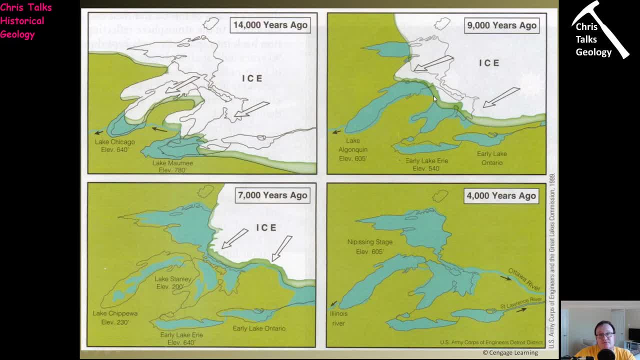 around 9 000 years ago. obviously, the glaciers are in full retreat. the ice glaciers are in full retreat. the ice glaciers are in full retreat. the ice water is filling the depression produced water is filling the depression produced water is filling the depression produced 7 000 years ago. now there is going to be. 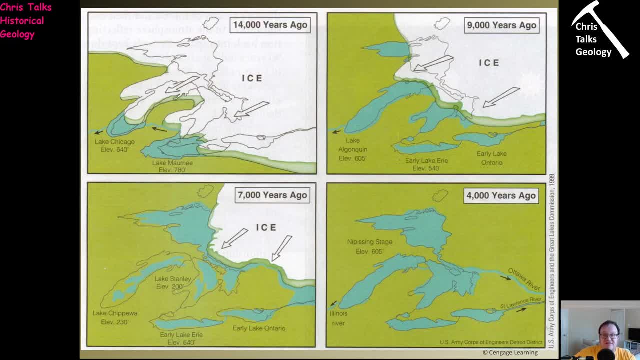 7 000 years ago now. there is going to be 7 000 years ago now. there is going to be some isototic isostatic rebound, which is some isototic isostatic rebound, which is some isototic isostatic rebound which is going to affect the lakes. so we can see 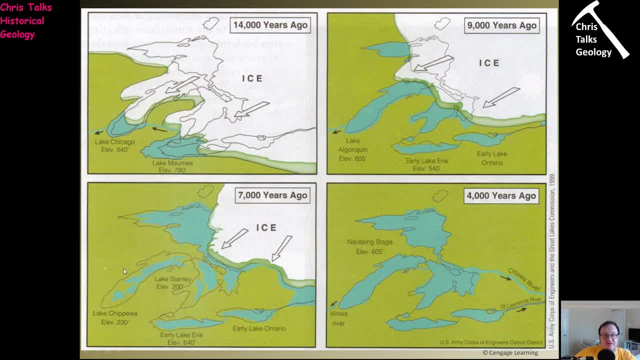 going to affect the lakes. so we can see going to affect the lakes. so we can see that some of the water is moving around, that some of the water is moving around, that some of the water is moving around in those lakes, some of it is, you know.